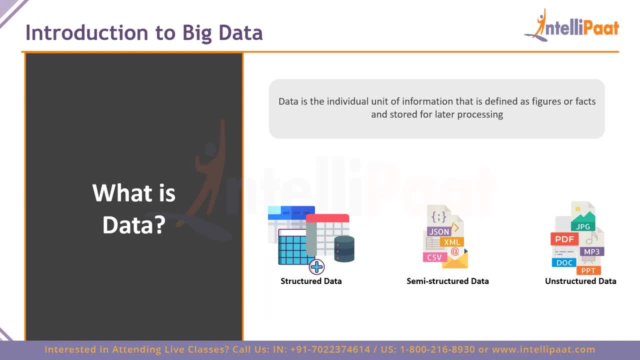 data with column names assigned, and column names have values, properly structured. If you want to run a query on it, you can easily run a query on it, right? So a fixed number of columns and values associated with every row of that column and primary keys if needed, and all of that So that 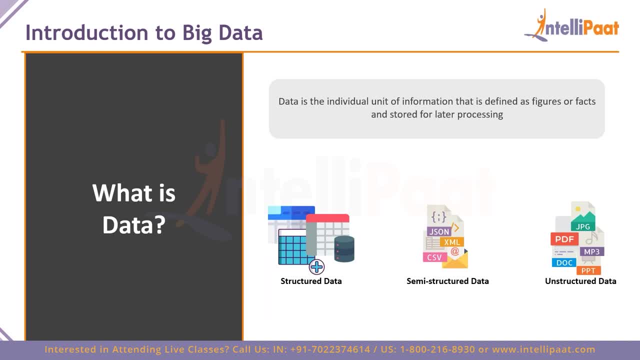 is structured data, data in a particular format Now. secondly, we have semi-structured data now. this is the trend for today. Today we use a lot of semi-structured formats. Semi-structured data is essentially data that is present on your computer storage, but unlike SQL tables, it is. 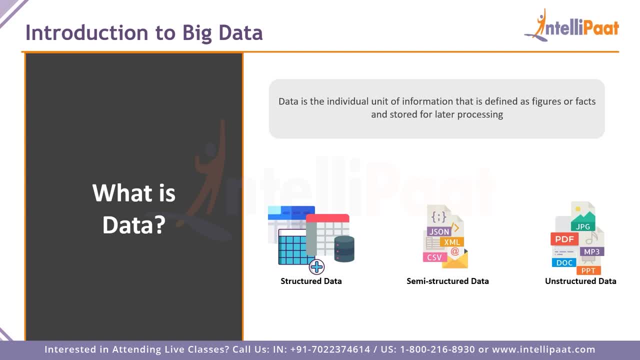 present in the form of files. So that means that you'll have data of different formats but it's not in the form of SQL tables with proper rows and columns. So this could be JSON files. this could be CSV files. JSON file has a particular format with the curly braces and key value pairs and everything. 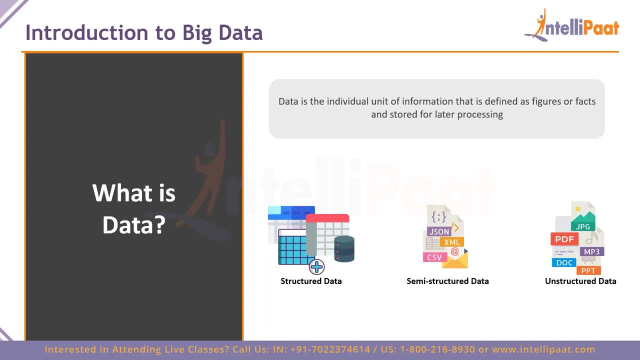 CSV files means comma separated values. So that means you have a text file, essentially, and instead of having columns that are separating your data, you have commas that separate your data. So that is what semi-structured data is. You can obviously very easily convert this data into structured data. 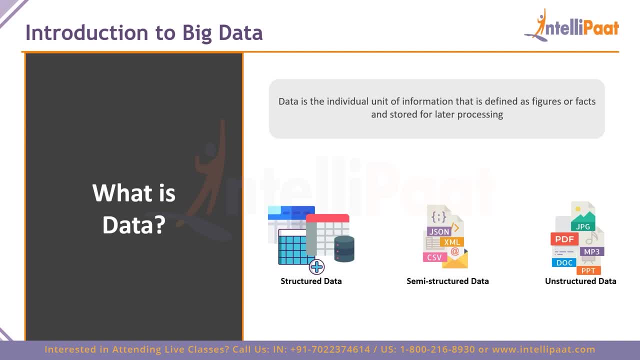 by simply importing it, by proper conversion and processing, into an SQL table, So it's very easily interchangeable as well. And finally, you have unstructured data. Now this is data that is random in nature. So if you convert an image, you would have data that is random in nature. So if you convert an image, you would have data that is random in nature. So if you convert an image, 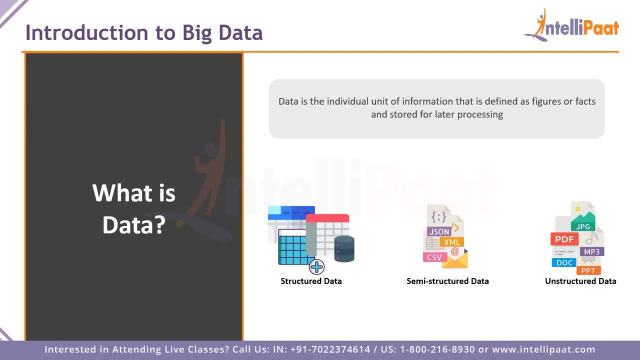 image file into a text file. if you open an image file as a text file, you'll see a random gibberish of information, right, nothing coherent at all. so that is this random data all bunched up together. same as with mp3, which is music files, mp4, video files, ppt, and all of these things, if you convert. 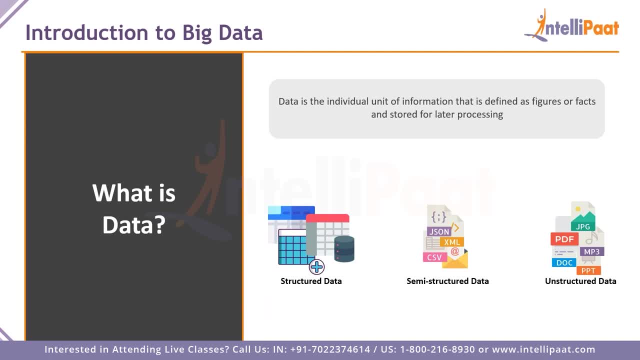 them into text files, you'll not see any order to it. so this is unstructured data. now it is up to you to find any sort of structure in it, if it is possible at all. so in computer storage, this is. these are the three types of data that you can essentially have, right? so this is what data is. 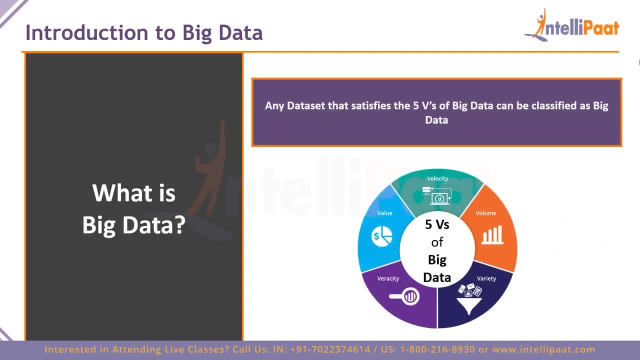 so what is big data? based on the previous definition of what data is right? so big data must mean something. any data set that essentially satisfies the five v's- uh, the five v's which are mentioned below- of big data, can be classified as big data. so any data, uh, that has velocity. 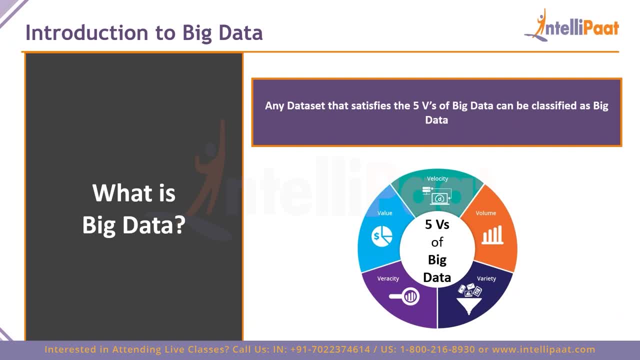 that means the data should be coming in at a really high speed. so it could be uh terabytes per uh per uh r. it could be gigabytes per second. it could be uh terabytes per day or petabytes per day, right, so that's that sort of speed. the the rate of data that is coming in should be extremely high. 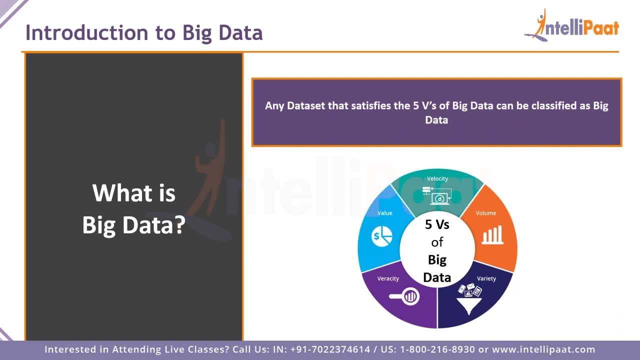 in the colossal numbers, so upwards of gigabytes, like at the extreme end of gigabytes, terabytes, petabytes, that qualifies for, uh, the high velocity that we need. next, the most obvious thing is volume. so when you hear the name big data, this is the first thing that comes to your mind: that data. 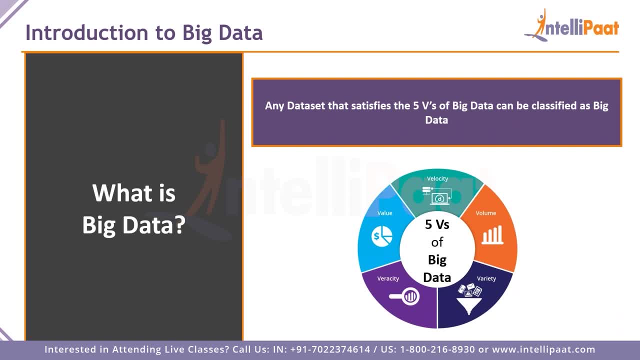 that is, is extremely large in size, is what's called as big data, so that largeness is associated with volume. so anywhere from terabytes to petabytes uh is considered as big data. is qualifying uh for big data essentially in on your storage system, on your hard drive or your ssd, and then uh, we have variety. 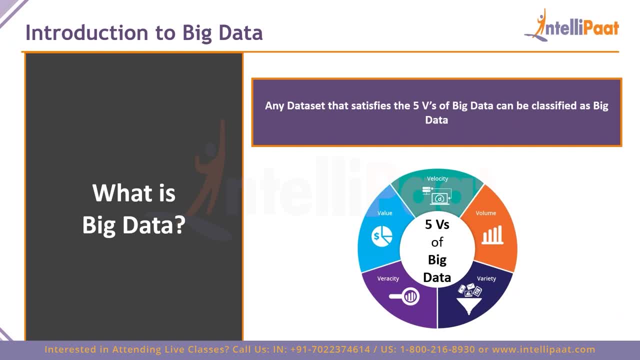 so the data should be coming in from different sources as well. so any in any real life scenario that you are going to be dealing with as a big data analyst, you are going to be having data that is coming in from different sources, so it's not just coming in from one. 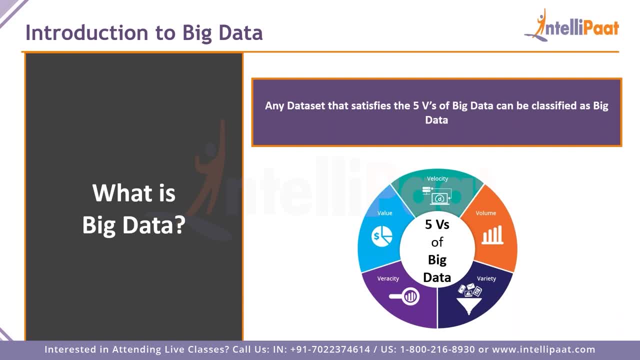 source like a sales data table. it's going to be coming in from a customer data table and a sales data table, it's going to be aggregated and you're going to be seeing it as a combination of views, right? so that's the word. that is what it means. it could be also that: 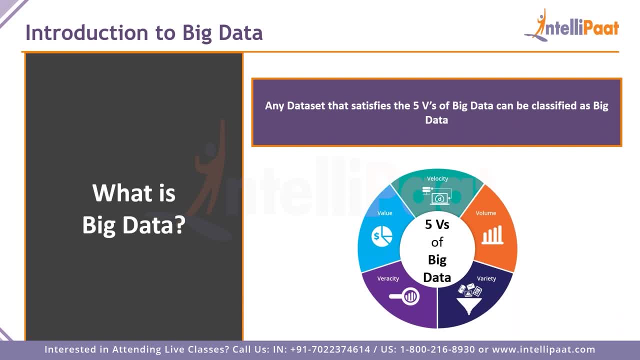 one file is a json file. the other file is a csv file. you're combining both of those datas together and you're getting your common aggregated data. so that is also qualified data. so you're getting your common aggregated data. so that is also qualified data. so that is also qualified. 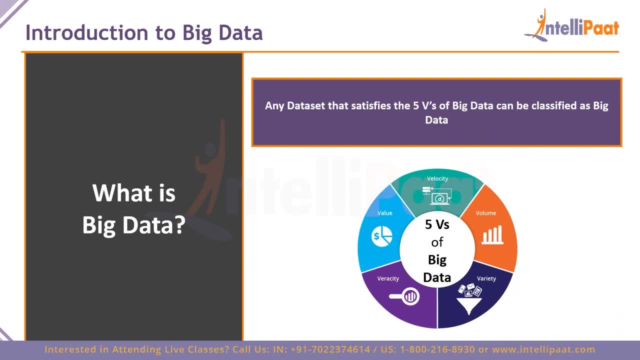 data, so that is also qualified data. so you must have some variety to it: different file formats or coming from different sources. then we deal with veracity. now, veracity means imperfection in data, so the data, when you're dealing with data that is on a petabyte scale, on a terabyte scale, you're 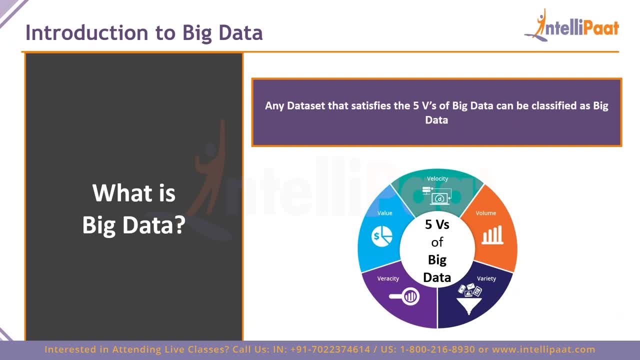 dealing with billions and billions of rows of information. so when you're dealing with that much information, no matter where that data has been collected from, it must have inconsistencies. it is in it and it must have some missing values or wrong information as well. right, so that means. 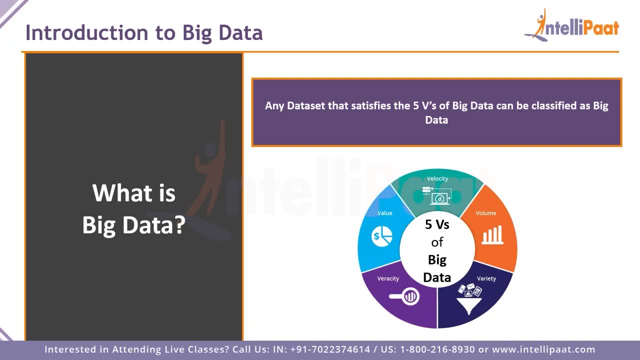 veracity. the data cannot be perfect when you're dealing with real life data at such a high magnitude. so that is what veracity means. and finally, we have value. so the data that you're taking in for creating your big data models should be of high value. so that means that, say for: 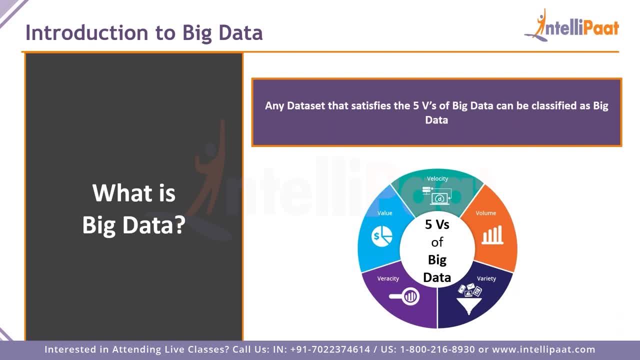 example, if you're picking up academic data of some college or university, so there are some columns for that data. columns that you'll have is the student name. you'll have the student registration number or roll number. you will have something like the grades that the student has attained. 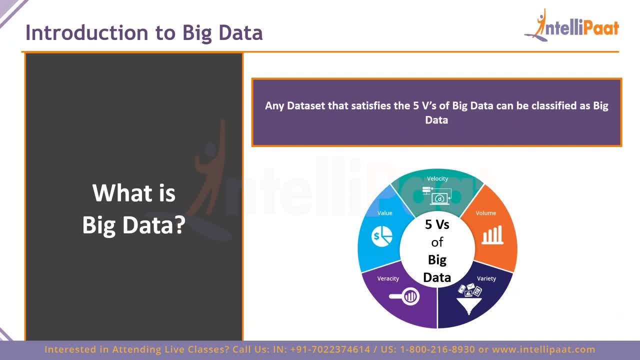 or the marks that the student has attained, the subjects that the student has taken. so, uh, some data in that is valuable, some data is not. for instance, the roll number is not valuable. so if you were analyzing anything with the roll number, which is just a mere indicator of what the primary 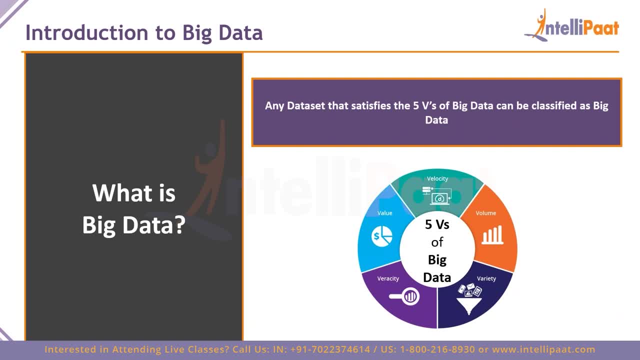 key of that student is it's not relevant to anything, right you? that data is not of value. so that essentially means you'll pick up the name if you have to. uh, just for identification purpose, you'll pick up the academic details, the, the marks that a student has scored, but you will 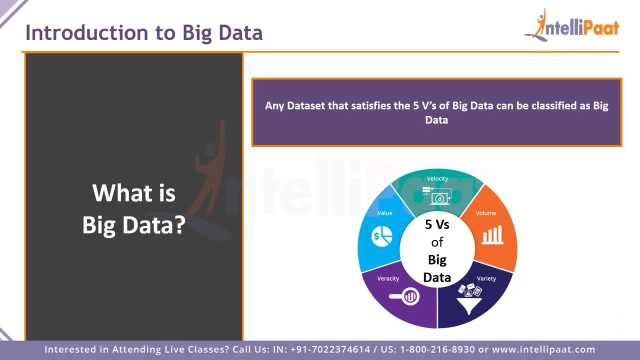 not pick up that roll number call, so that particular column, if you pick that up, even if it's in the terabytes, that does not account for big data. it should have value. so these are the five v's of big data that need to be satisfied. uh, in order for data to be. uh, qualified data to be. 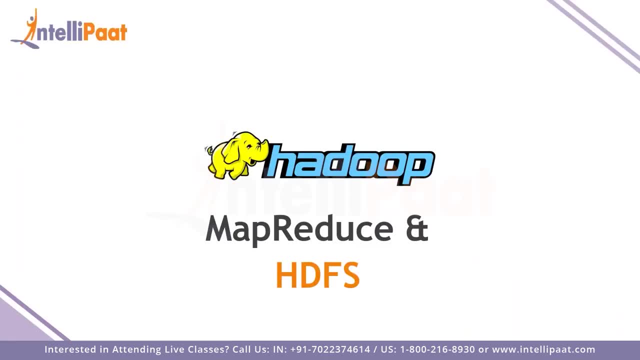 called greater to qualify as big data. so firstly, let us understand the initial solution that was created, uh to deal with the big data problem. so, obviously, if you're dealing with terabytes to petabytes of data, you uh. even the best of computers and laptops today, the inbuilt storage size is like maximum that you get is one terabyte in laptops. 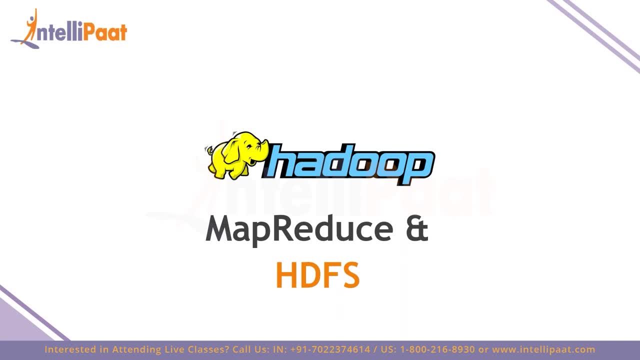 and then if you have a computer or a desktop, uh, you can upgrade it to two. there are two terabytes, but for a general consumer, that is all you get. like 500 gigabytes to one terabyte is the general end that you get for today, right? so that is what there is, so definitely you cannot take this one. 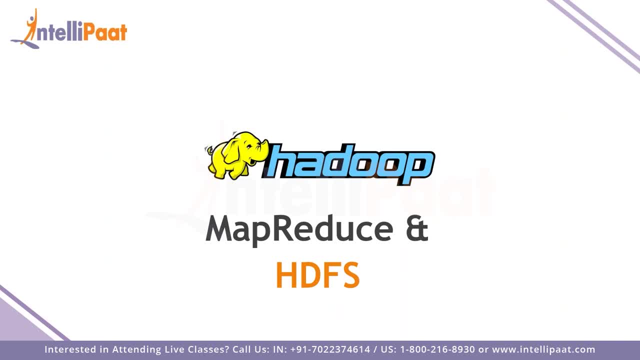 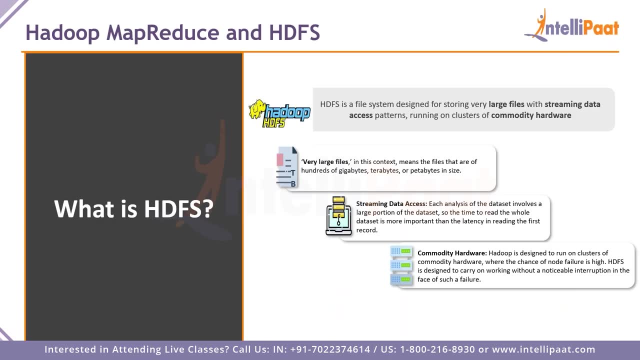 terabyte of data and put it entirely on your computer and then hope to analyze it in a reasonable amount of time. so that is where hadoop came in. hadoop is a framework that was developed in java to deal with the big data issue, so how hadoop solves this problem is quite interesting. 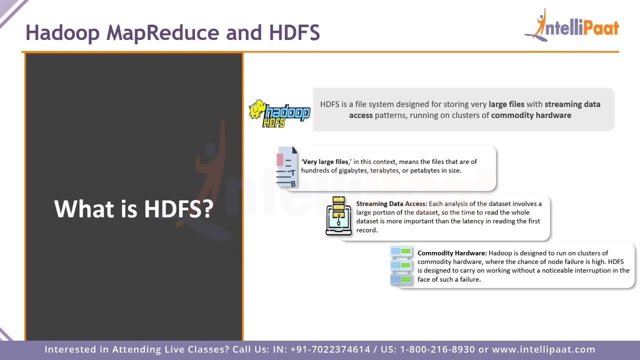 actually what hadoop does is it takes a computer network and there are a lot of computers that are together in a computer network, right? so there's a server and there are lan wires and all of those computers are connected to lan wires and essentially you're creating a network. so what? 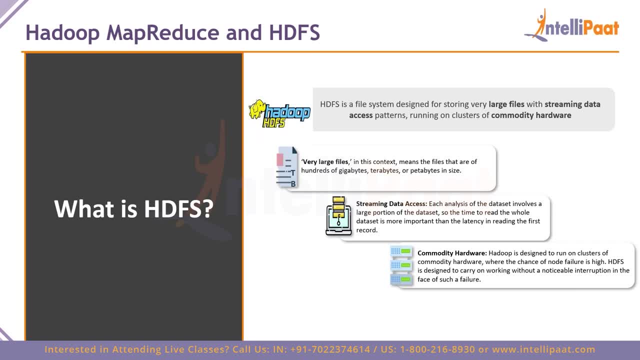 hadoop did, was it found a way to coordinate all of those computers together to deal with the big data problems. that means a certain area, a certain portion of the hard drive of each of those computers was reserved. and when it was reserved, uh there, it basically accounted for the hdfs. 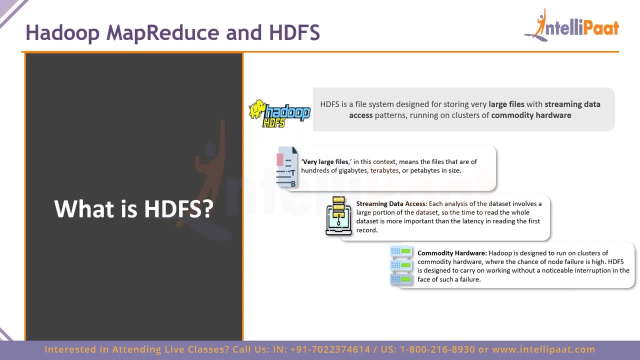 which is the hadoop distributed file system. so all of these computers act together to store this data. so whenever data comes in uh to the hdfs or the hadoop server, it gets divided automatically and is stored across all of these computers in an equal distribution to be able to deal with the 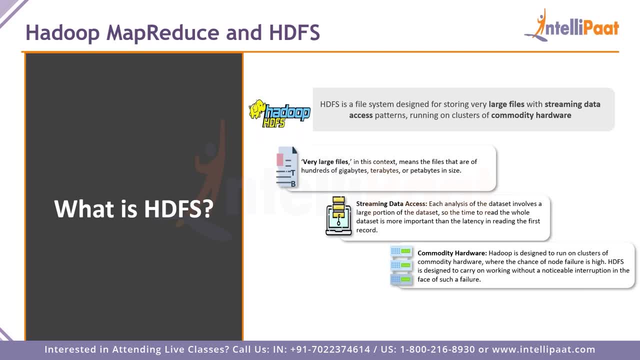 size issue. so one terabyte of data gets divided into, say, uh, blocks of 50 gigabytes of data, and one 50 gigabyte block is sent into one computer, and so on to the next, and so on to the next. so that is how we deal with this issue. 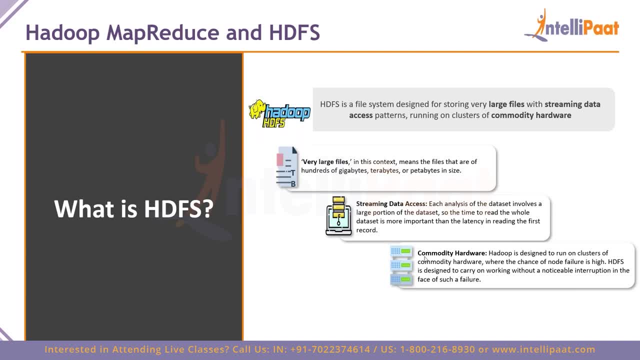 you solve the storage issue by dividing that data. so, uh, very large files in this context means the files that are of hundreds of gigabytes, terabytes, petabytes in size: streaming data access: each analysis of the data set involves a large portion of the data set, so the time to read the whole data. 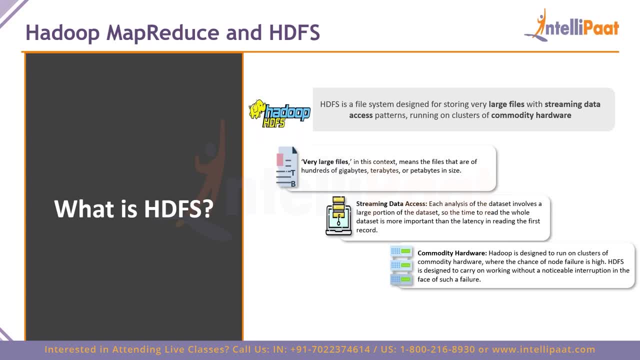 set is more important- latency that is required to deal with the first record. so that essentially means that you need a solution that minimizes the input output delay while analyzing the data. so if you need to be analyzing it at a really high pace to be able to deal with such a large amount of data, 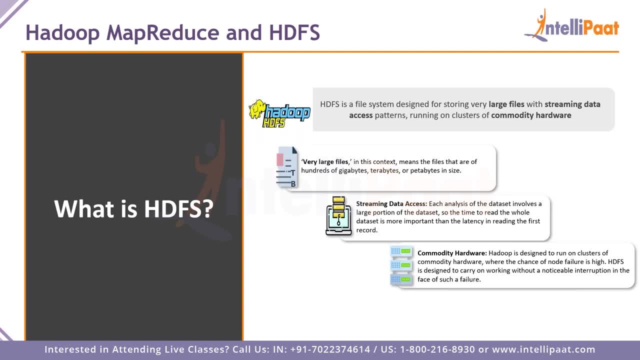 and then commodity hardware. hadoop is designed to run on clusters of commodity hardware. now, commodity hardware means that you have two options to run hadoop. earlier hardware was really expensive, so buying expensive server rooms and server farms to store inside your office and run your hadoop. 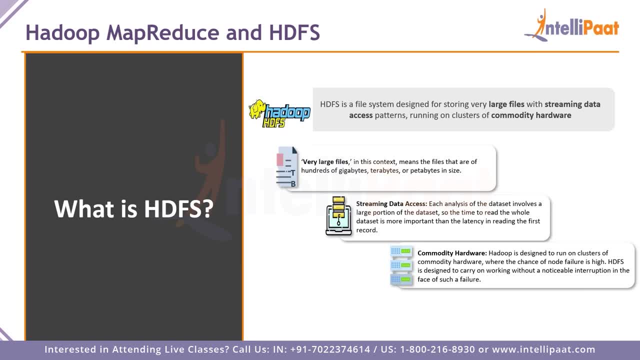 server on would have been really expensive. what they came up with is that you can simply use the that you use in your office as contributors towards your hdfs server. so that is what commodity hardware means. without buying anything new, you're essentially using the workstations that are. 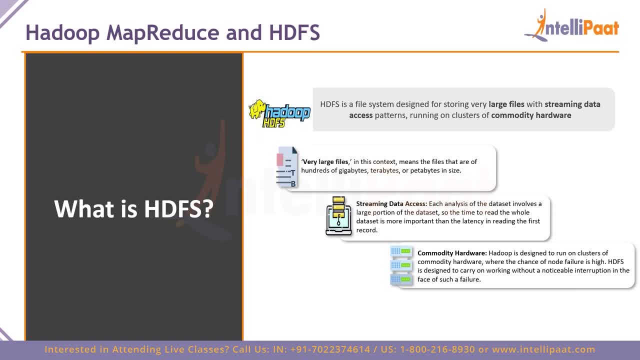 present in your own office space to be able to contribute to your hdfs server by dedicating a certain amount of hard drive space and processing power to your hdfs and hadoop server. so let me look at some doubts related to hadoop in general. so firstly, i'm getting is the first doubt that i'm 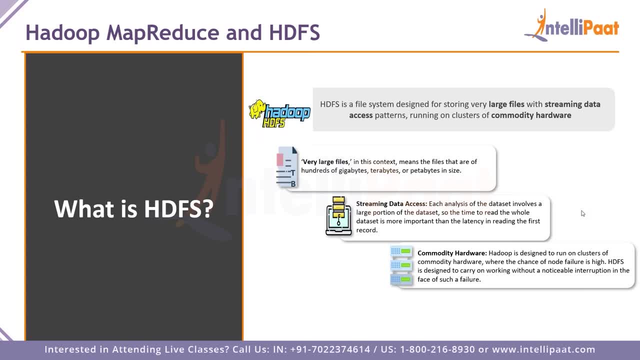 uh, what is map reduce? so we're going to be actually understanding what map reduces. briefly, because that is not the point of today's video. we're going to be understanding spark, but i'll just tell you what map reduces. firstly, this is what the hdfs is. hdfs is the solution of hadoop. 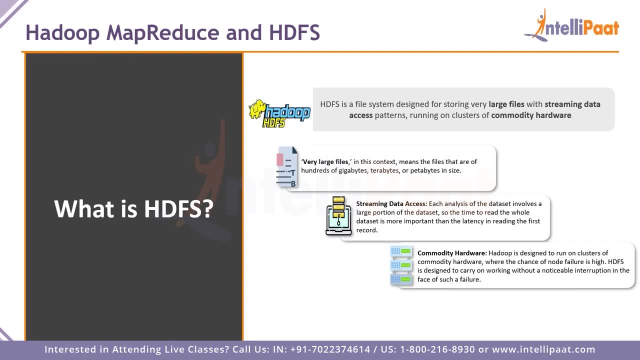 for storing data. now, this is not for processing data, this is for storing data. right, you store using uh, the division method, by dividing the file into blocks and storing it across various nodes in your. that is also called a hadoop cluster, by the way, or a big data cluster. secondly, uh, we have the second. 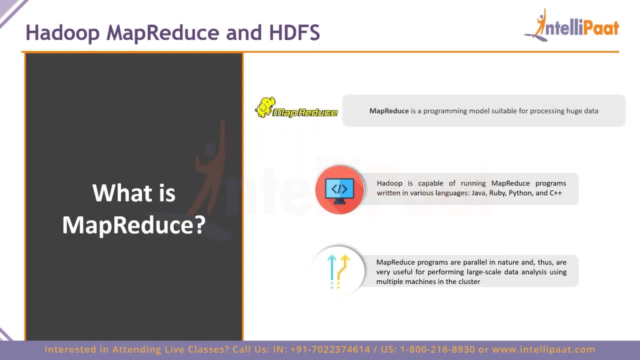 component of hadoop which was developed for processing. now you have all of this data stored in your hadoop or big data cluster. how do you process it? so for that also, uh, hadoop had a second component, the processing component, or the processing framework uh called map reduce, right. so 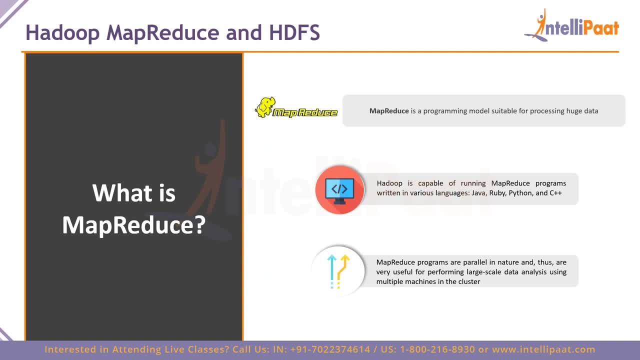 hadoop is capable of running map reduce programs with various languages, as you can see: java, ruby, python, c, plus, plus. so for that you have to have a big data cluster and you have to have a big data cluster to run it, and also you can use, uh, a lot of libraries, like you can see in the middle of 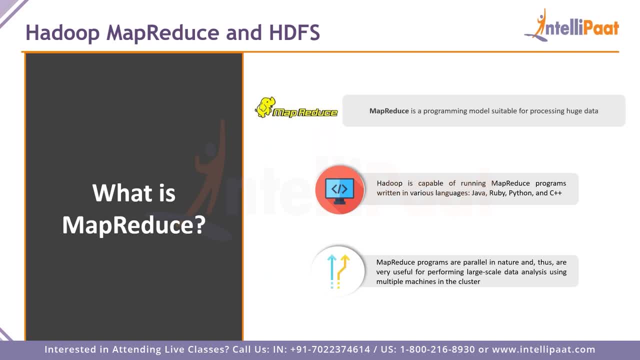 java you get hadoop libraries. if hadoop is already installed onto your computer or the server that is required to run it, uh, the libraries are already there present, and you can simply import those libraries into your java code and implement it accordingly and you can basically create a program. 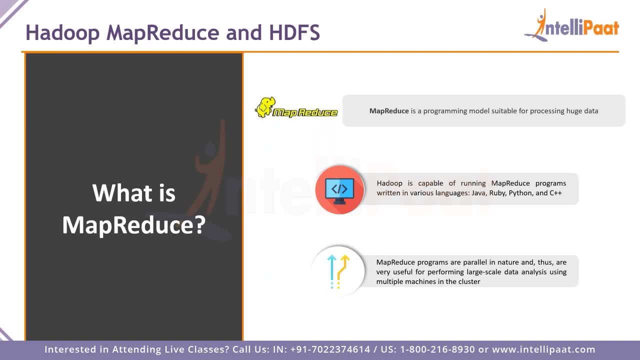 that uses all of the nodes that are present- or some of the nodes that are present- in your big data cluster run in synchronicity, run in parallel, to be able to execute all of those blocks data. so instead of having that data run in a sequential manner where it takes days to maybe. 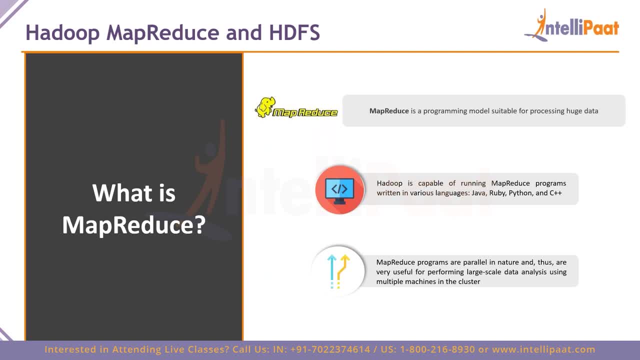 months to analyze that huge amount of data. you're simply analyzing each block of data on that respective node in parallel, reducing the time exponentially. so that is the advantage of map reduce: that you get the processing element. so let us look at the architecture of the hdfs and how. 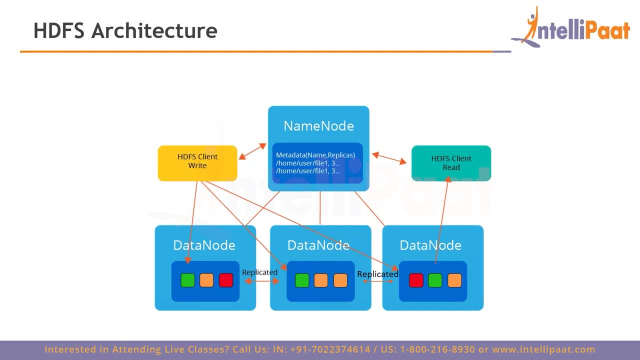 map reduce would actually operate on it right. so, uh, the architecture is quite simple. so imagine: uh, generally, the big data clusters and big organizations have hundreds, thousands of nodes attached together. here we're only talking about four nodes, just so. that's so you guys can understand what i'm actually uh talking about here. so, uh, firstly, there is 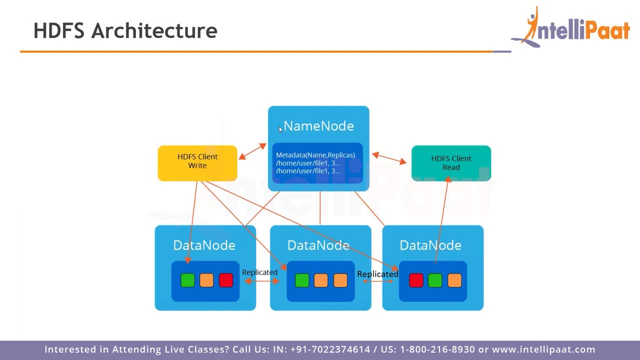 the name node. now, the name nodes could be multiple. the data nodes could be multiple. there's no limitation that the name node should only be one node. it could be multiple nodes, right? so what happens is, uh, you'll take the computer that has the most, that is the weakest, essentially, and you'll make it the name node and you'll take three average. 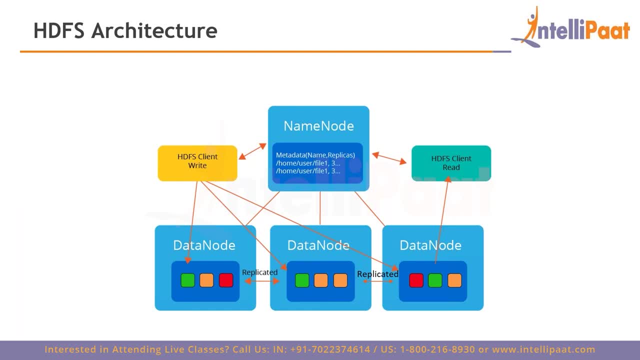 performance computers as data nodes, right? so whenever, uh, you're coming in as a client to that particular hdfs or big data cluster, you'll start to upload a file. say it's a terabyte file, right, and you're starting to upload it. so what will happen is you'll first contact the name or the 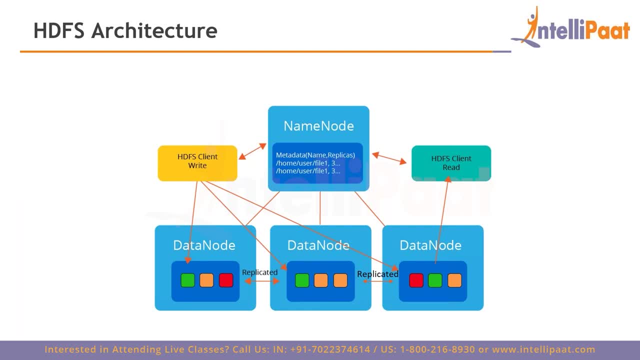 name node will then see which data nodes have the space. so it will check which particular hard drives in the ddo have the space to store that data. so firstly determine which data nodes you're going to be storing your data on. then, uh, it will. it will basically communicate the block size. 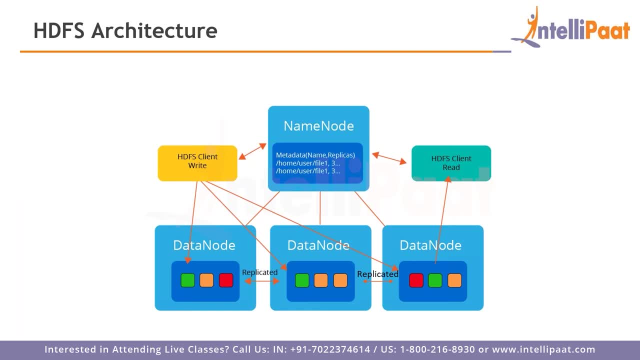 so the data will automatically be divided into the blocks of that size, whatever block size you've set, and then it will get start. it will get started to store on the data nodes one by one. so the first block- as you can see there they are colorized as well- the the first block, let us say the green block. 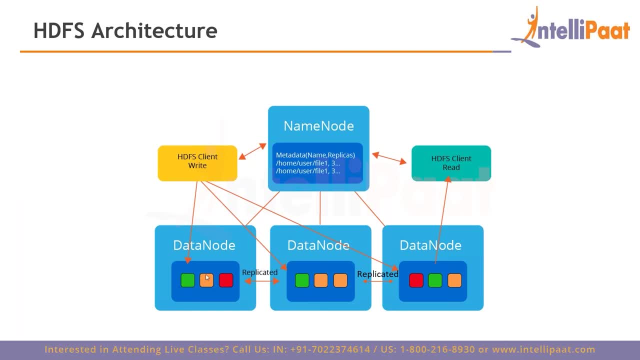 goes on the first data node and then the- the orange sort of block goes on the second data node right, and the third, the red block, goes on the third data node. so imagine that right there are also two other colored blocks. i'm going to be explaining what that means in a second, so imagine 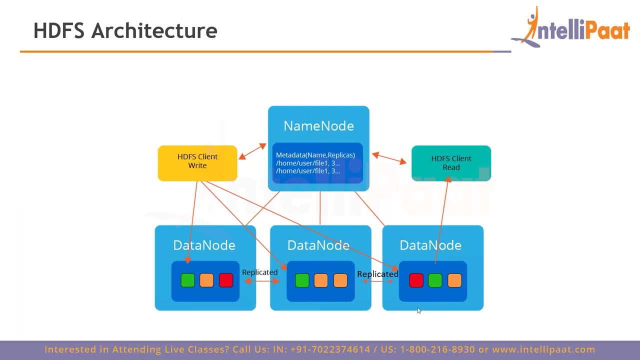 you've divided into green and orange went over here and red went over here, right, so whenever map reduce programs run on the hadoop cluster, the green block will be executed in data node one, the orange block will be executed in data node two and the red block will be executed in data node three. 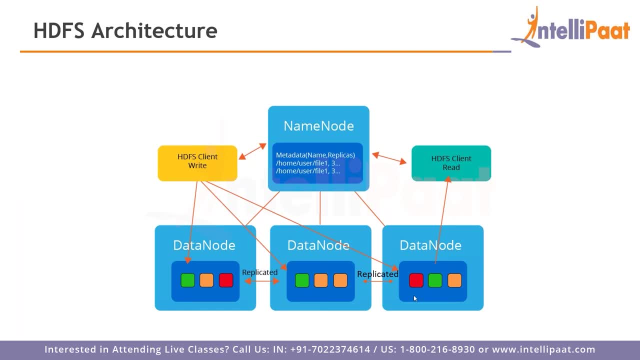 minimizing the time by three. so it will basically divide the time by three. so, and the next thing that hdfs helps you implement. now, this is not that prominent as we're only using three data nodes. right, if there were 100, then it would make sense, say you set the replication factor, the replication, 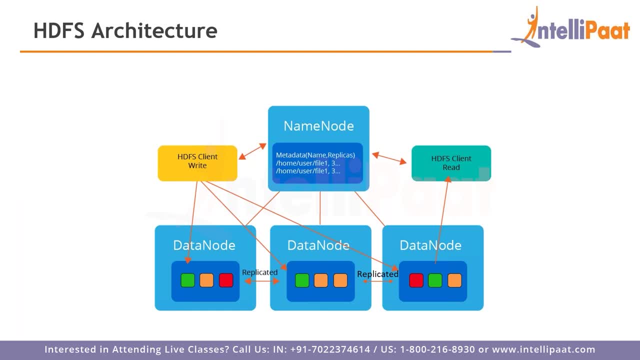 factor to two, right. so the replication factor essentially is a solution that helps you deal with data loss. so say, data node one fails, it goes bad or some hardware failure occurs. so you don't want to completely lose the green block, right, you don't want to lose the green block because that is just a part, that is a part of the data that you don't want to. 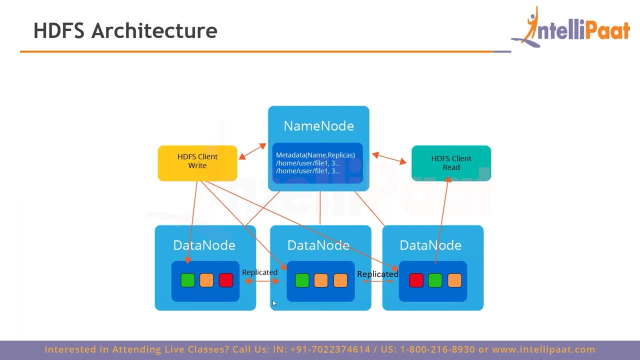 lose. so, hdfs, depending on the replication factor that you've set in your hdfs, if it's two, the green block will be replicated two times, so it will be replicated on data node two and it will be replicated on data node three as well. and if there are 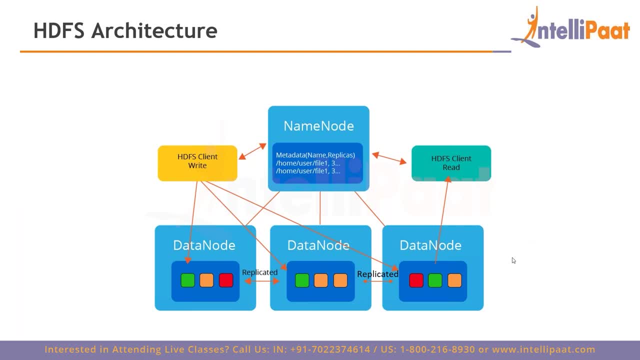 replication factors. three: if there is another data node, it will be replicated on that data node as well. right, so even if data node one fails, you still have access to data node the particular block that's green. so similarly, data is also replicated, whatever blocks that are put on the 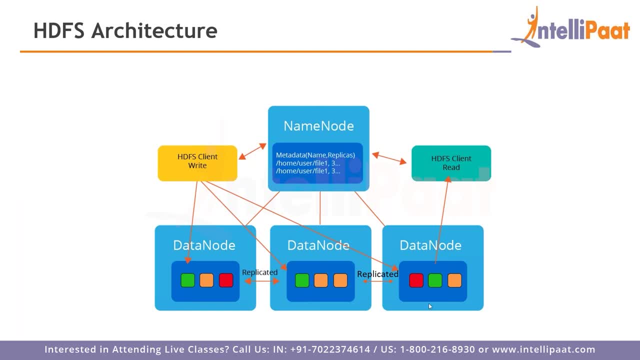 data node. so say, then you uploaded the file on the data nodes. the client comes in to read the file, right, he wants to access that file that you've just uploaded- the other client that wants to read it. so what will happen is he'll be automatically connected to the data node. 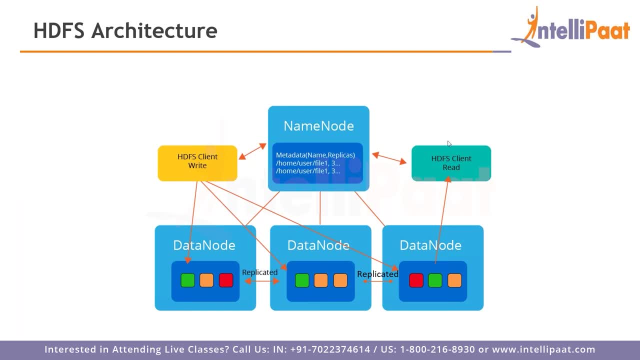 once he contacts the name node, he will be automatically connected to the data node that has the that is the closest to him, so minimize latency, essentially. so if data node say if this is in- uh, say for example los angeles, and this data node is in, say new york, they're all connected. 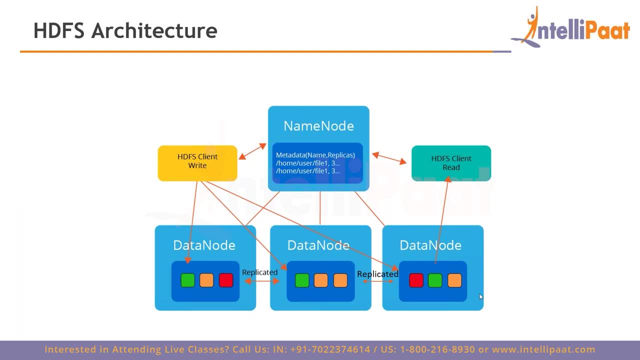 together for some reason, if they're not closely located, for that matter. so if this person is in new york, he'll be getting access to this data node, because that is the closest right. if they're, all of the data nodes are present in one location, so so in that case it doesn't really matter. 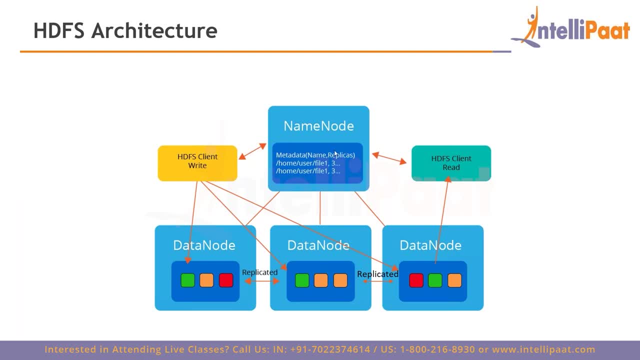 in that manner. so the name node is storing where the data begins and where the data blocks end. the name node is storing that information, the data of the data, the metadata. so it will store where the green block is, how many times it has been replicated and where the replicated blocks. 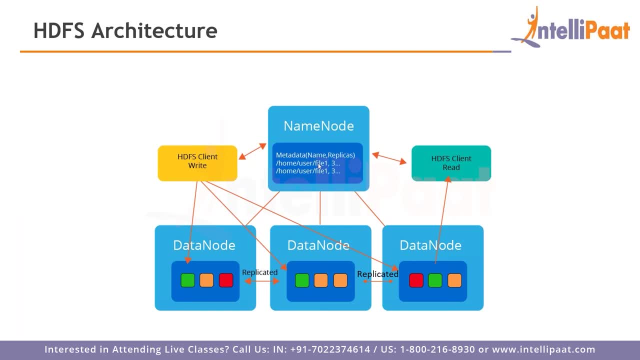 are right. so that is what the name node will store. so in that manner the hdfs essentially runs in a very conjunctive sort of way where everything is organized and stuff. can we integrate hadoop with azure, or it needs linux system. you can easily integrate with azure, azure and 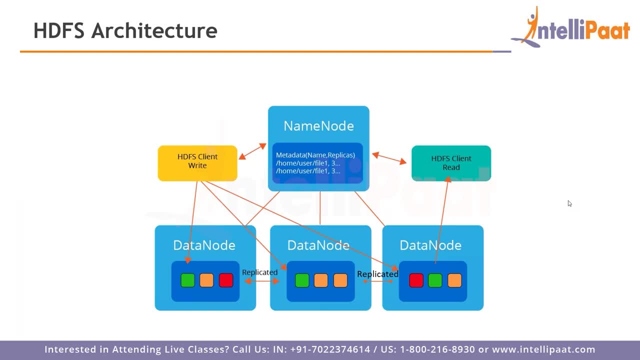 has a service altogether, uh, for that particular aspect. so firstly, azure: you can use data bricks with azure. azure is a microsoft cloud service, for those if you don't know. you can use data bricks with azure and it has all of the cluster computing elements already built in without you. 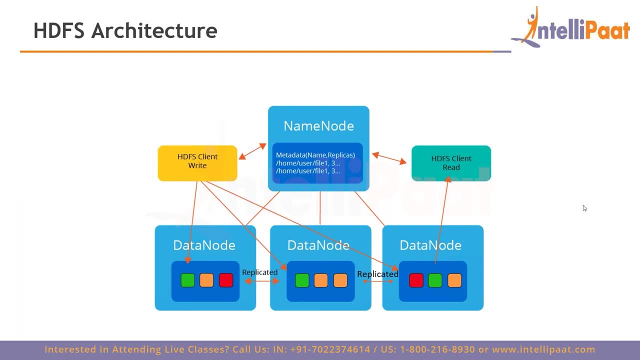 having to install anything. okay, map reduce runs on the same hadoop cluster that stores the data. uh, using the nodes to process in parallel? yes, yes, it does that. so the server, what? what is this the next question that i have: using map reduce for storing huge data so that using server is reduced? 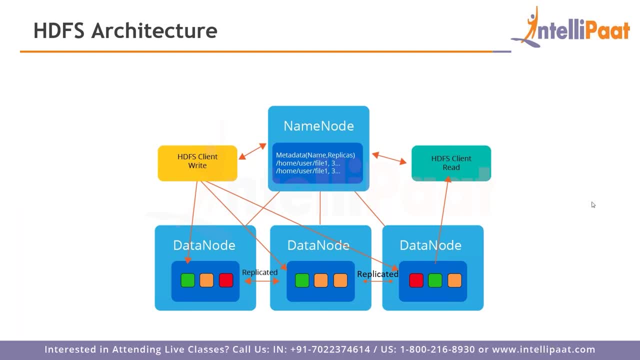 or not. so see, in today's day and age, server technology is really cheap. so when hadoop was developed, originally servers were really expensive. so, uh, servers are really cheap now they're not as expensive as they used to be. so earlier, when this was made, servers were really expensive. 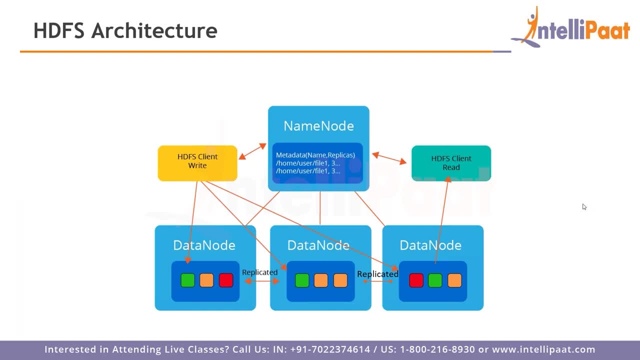 but now we can use servers as well, server rooms as well, to be to use hadoop with all right. so it's not an issue, it's up to you, it's up to the financial status that your organization has, uh and uh, how much usage you have for that particular technology. that determines. 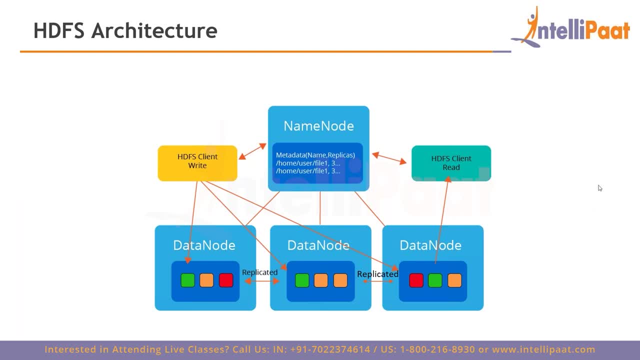 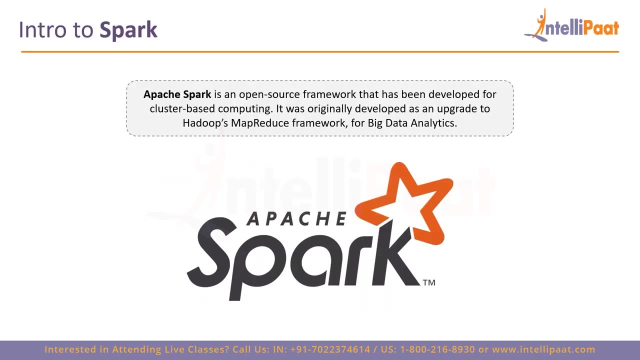 whether you will buy a server or not for hadoop. all right, so let us continue now. intro to spark. now we understand what map reduce and hdfs are right, so we need to know what the step up is right. so apache spark is an open source framework. open source, which means that you can go and 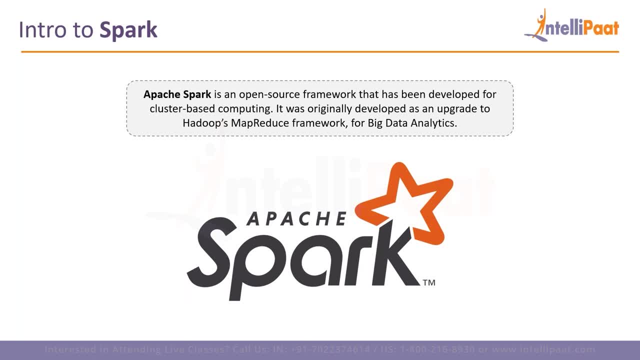 look into the source code of that particular program and make changes to it or contribute to it or make any changes to your code as well for your use case, if you have any custom use cases. so it was developed specifically in mind with cluster based computing or hadoop, cluster computing. 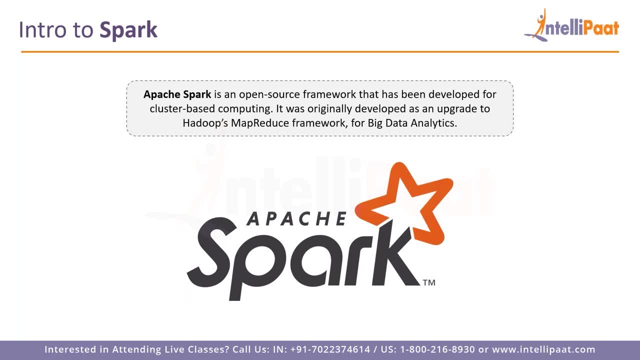 or big data cluster computing. it was originally developed as an upgrade to hadoop's map reduce framework for big data analytics. so keep in mind one thing over here: it is an upgrade to the map and upgrade to the hdfs framework, so that means apache spark is also a framework that deals with. 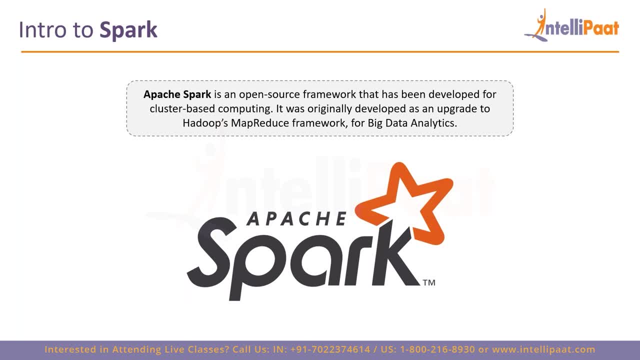 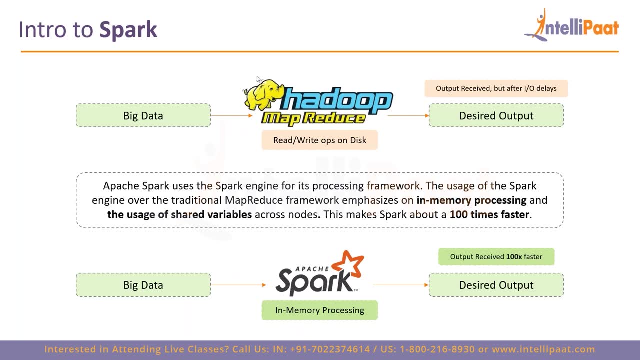 purely programming elements, the processing elements. it does not deal with storage. so let us continue. so imagine uh. firstly we'll look at the hadoop map reduce- so big data. you have big data sets uh present on your hdfs. you use the map reduce framework to basically analyze that big data. or 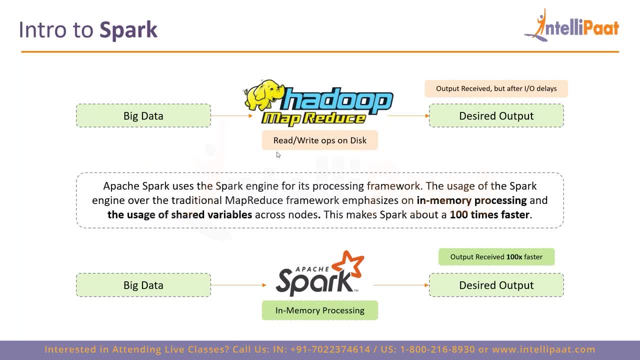 process that big data and you get your desired output. the problem with this is that the big data is uh, with hadoop, map reduce. at the time when it was made, ram or random access memory or physical memory was really expensive, so they used to use a disk for that or hard drive for that. so uh say the 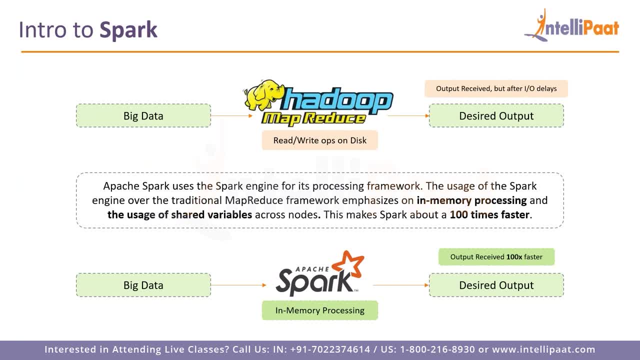 big data was present on the hard drive. a certain amount of that data is put into the ram and then processed and then put into the output section and then the uh data is picked up from the hard drive- again- the remainder part- and then it is put into the ram and then it is processed, and then it is. 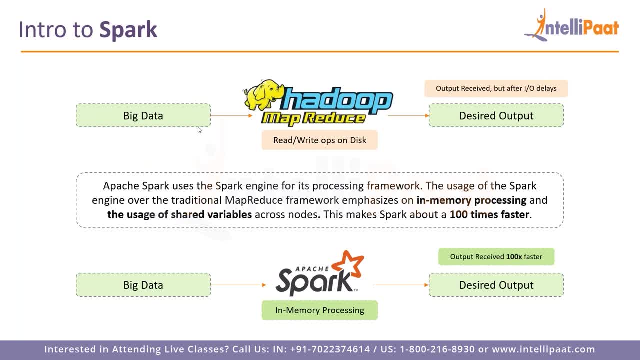 wouldn't be output. so in all of this, you will see that the big data was put into the output. so in all that, what happens is when you're picking the data, when you're transferring the data to and fro from the ram and the physical drive that you have on your computer or the hard drive that you have. 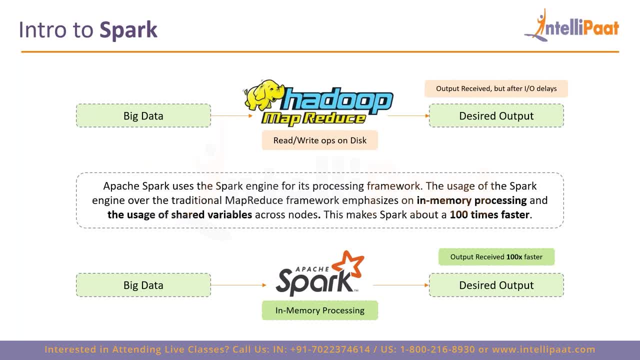 on your computer there is an input output delay. what does that mean? that means that, uh, that time that it takes for data to be transferred from hard drive to ram. it is not much if you're dealing with small amounts of data, but when you're dealing with large amounts of data it accounts to a lot. 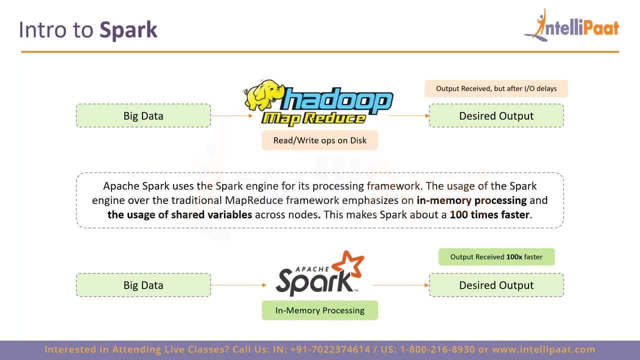 it adds up the time a lot, right, it makes your process a lot slower than it needs to be. so when, eventually, ram got cheaper, now on your mobile phones you have 64 gigabytes of ram, right? that is how cheap ram is today. so as ram got cheaper, uh, we came up with a different technology to deal. 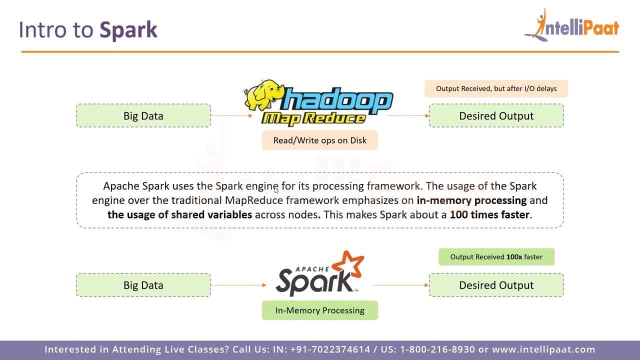 with this particular input output delay. so apache spark uses the spark engine for its processing framework. the usage of the spark engine over traditional map reduced frameworks emphasizes on in-memory processing and usage of shared variables across nodes. so this makes spark about a hundred times faster. so for 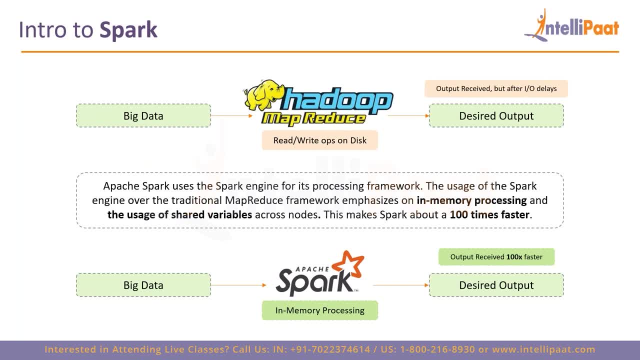 small data sets for, like megabyte data sets, it you will not see the difference. but when you're dealing with terabytes to petabyte sized databases or data sets, then you will see how fast apache spark is, because over time it does not add any input output delays, it adds very minimalistic. 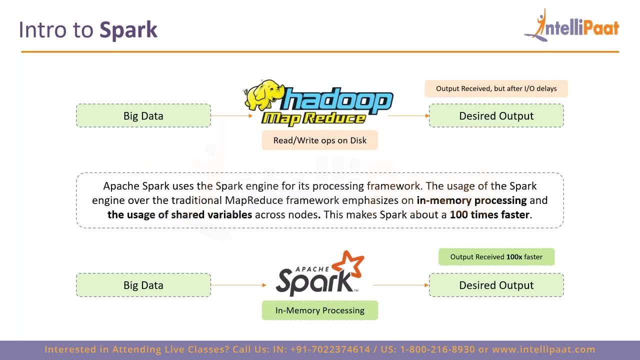 input output delays right as compared to when we were dealing with hadoop and map reduce specifically. so you have big data, you have in-memory processing, so essentially what happens is say: uh, your block size, you have particular block size of uh. the data that is present on a particular node is about. 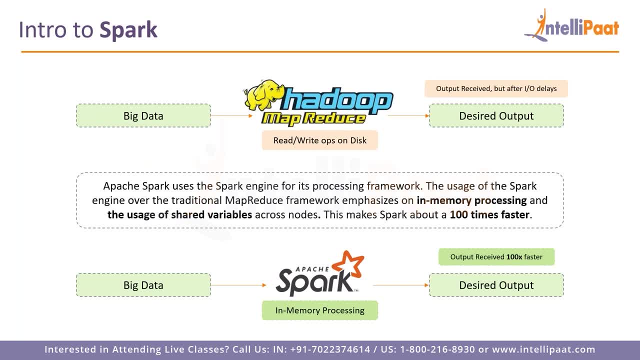 three to four gigabytes. that is how how much data was divided and put on one node of the terabyte data set that you have. so it's three to five gigabytes. you have a ram of eight gigabytes on your node right, so that three to five gigabytes will entirely go into the ram right at once. it. 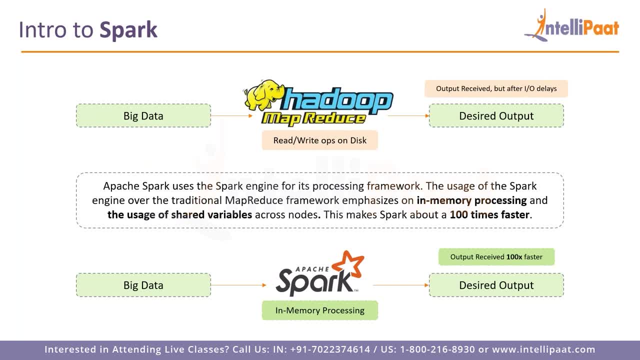 will go into the ram and it will stay there for a long time. so you have a lot of data that is there until the job is finished. so whatever intermediate outputs you get, whatever processing you're doing, it is all happening instantly because the data from the ram is going into the cpu and the 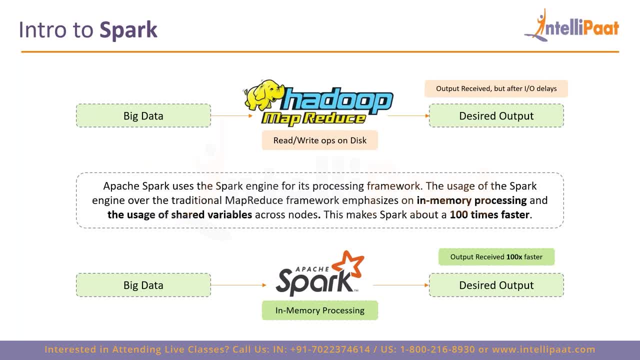 intermediate outputs are coming back into the ram almost instantly right, so it minimizes the input output delay. the only delay that you get with spark processing is the cpu delay- how much time it takes the cpu to analyze that data. you don't have to deal with the hard drive transfer time. 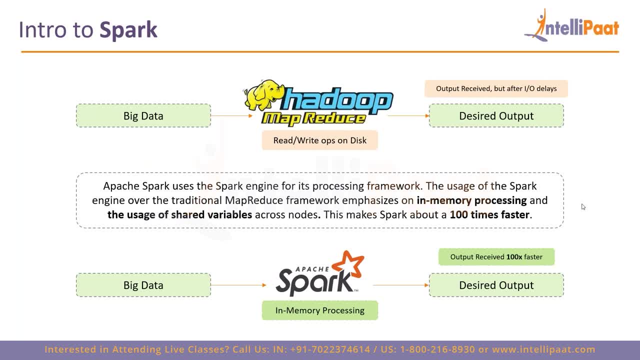 right. so that's actually the real challenge and obviously it's quite a lot of things that people are doing to reinforce what they're doing, to use the hard drive. so what would those things mean? and, as you said, we're going to go into the matter of communication. so this is what we do in the 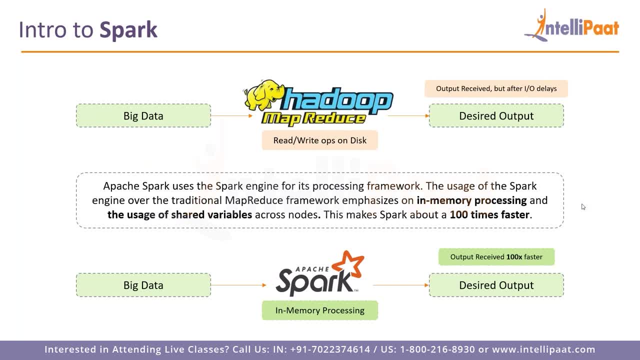 the process and in the tutorial we're going to look at, uh, the png and the, the project data and how it speeds up the process. one particular query that i'm getting is: because we now have more ram as compared to the earlier days. yes, because earlier even one gigabytes or two gigabytes of ram. 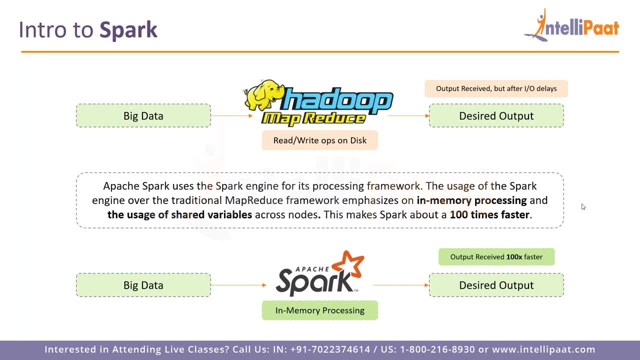 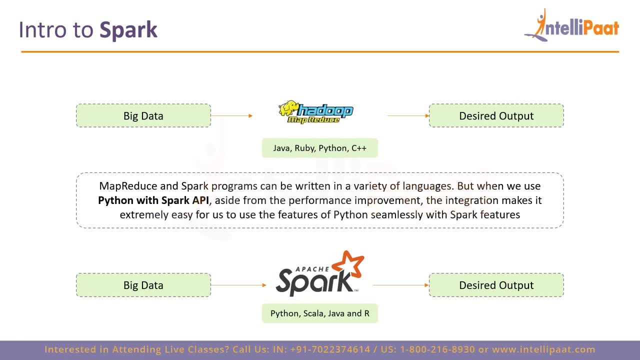 like general user-based laptops. that is how cheap ram is. so that is why. so, firstly, let us understand the next step. uh, big data. when you're using it with map reduce. when you're processing it with map reduce. you can use java, ruby, python and c plus plus, so these particular languages have libraries. 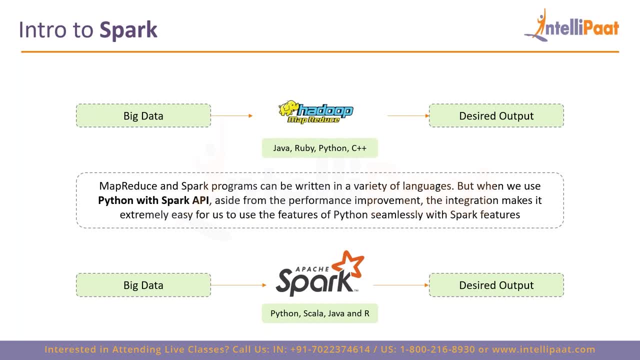 for map reduce and you can integrate that in your code and analyze that data with the input output delays that you have with. so map reduce and spark programs can be written in variety of languages. but when we use python with the spark api, so for uh, apache, spark provides four apis essentially. 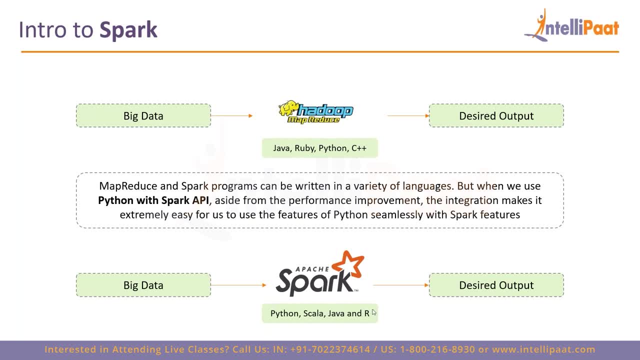 so one is for python, one is for scala, one is for java and one is for r programming right. so for those of you who are coming from a data background, you might be familiar with python and r at minimum right, and java and scala are development based languages for those of you who are coming from. 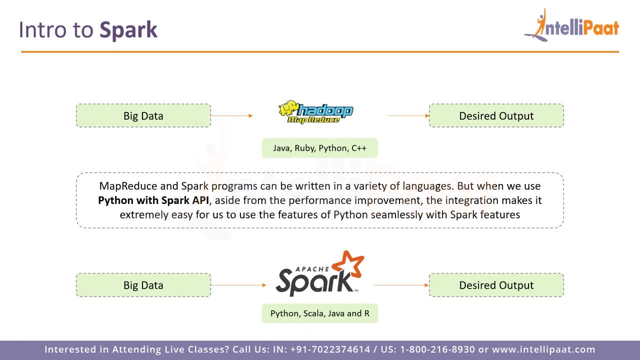 a development language, right. so it depends on what kind of background you're coming from and what would be easy for you, but would recommend python- right, because python is very easy to understand and it is generally recommended if you want to progress in the big data field, if you want to do more things with 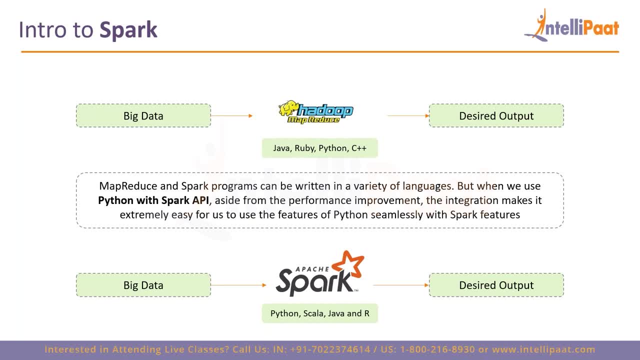 big data. even r i wouldn't recommend as much as i would recommend python, right. r is more somebody who's purely uh, from a data analytics field- right, he does not do one. i want to do anything more other than data analytics and visualization. does not want to develop anything or do some. 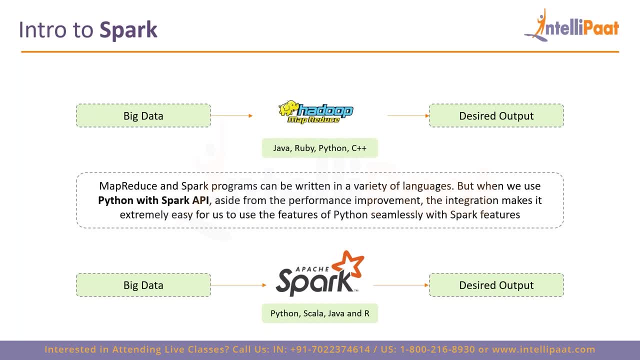 customizations with the data. so r is a very limited language in that regard. python the best language, i would say, for data oriented jobs. all right, so, aside from the performance improvement that you get from using the spark engine, the integration makes it extremely easy for us to use the features of python seamlessly with spark features, so that 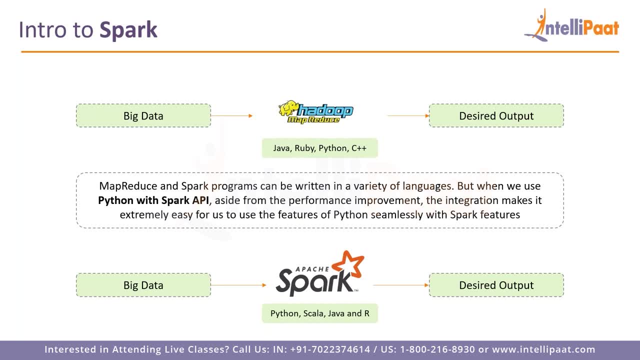 means other than the spark api. you have the mat plot clip in python. you have a scikit, the sk learn library that you have, which is for machine learning right. you have pandas, you have numpy. you have all of that. so you can integrate that almost seamlessly with the spark data frames and the 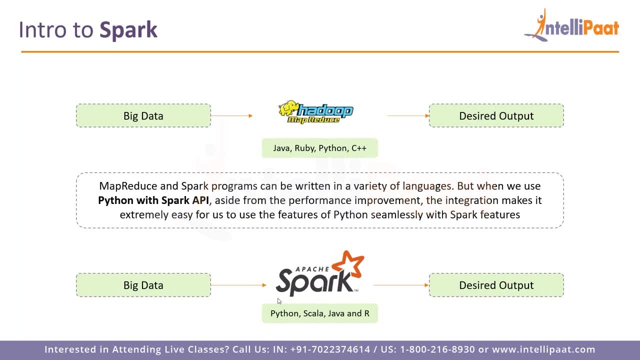 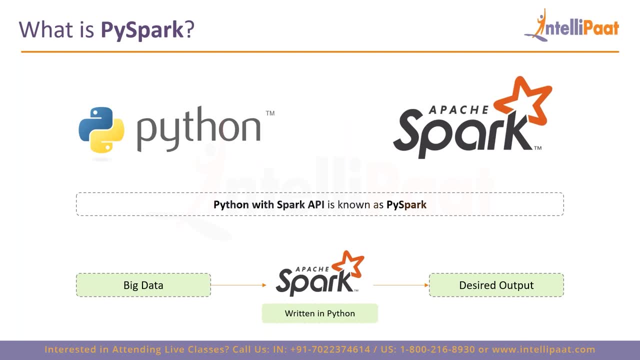 spark features that are there. so, uh, that makes it extremely convenient if you're doing with python. so essentially, python with the spark api is known as spark by spark right. so integration of python and spark. so that is straightforward, i would say at this point. so let me look at some doubts before. 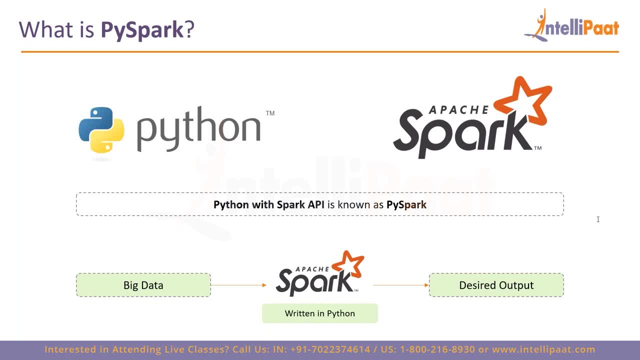 we actually get into the demo. so one question that i'm getting is: what is the minimum size of ram required for spark? so, uh, if your node uh is functioning, if your cluster is functioning, uh, particularly, it is recommended that you have at least two gigabytes of ram on your node uh to be included in the cluster uh. otherwise, uh, you can. 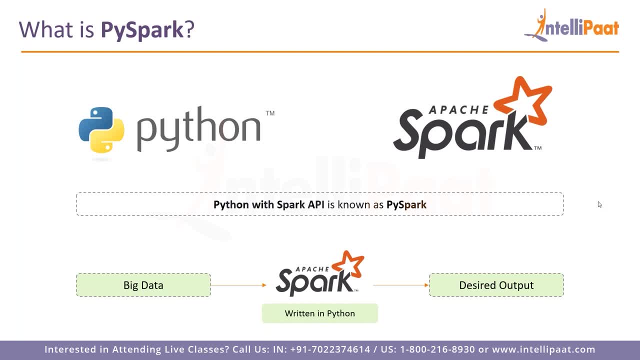 still configure it in a way where it would run, but there is no minimum requirement, uh, unless you're running a single node cluster, right? if you're running a single node cluster, where you're doing it for training purposes and you only have, uh, two gigabytes of ram, then it might cause you. 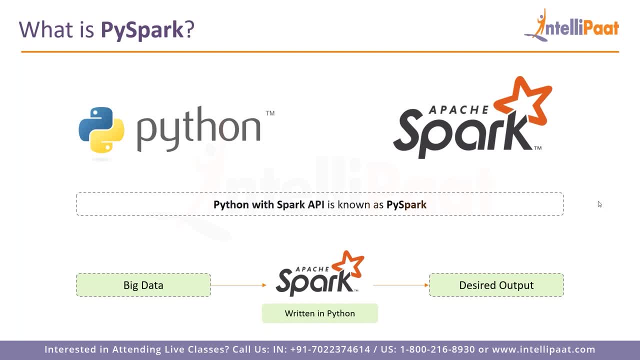 some trouble, but if it's part of a cluster, you can easily uh move your way around it and do some configurations where it could run. so how to get pi spark in system? so, uh, pi spark has a complex way of installing it. that is not something we're. 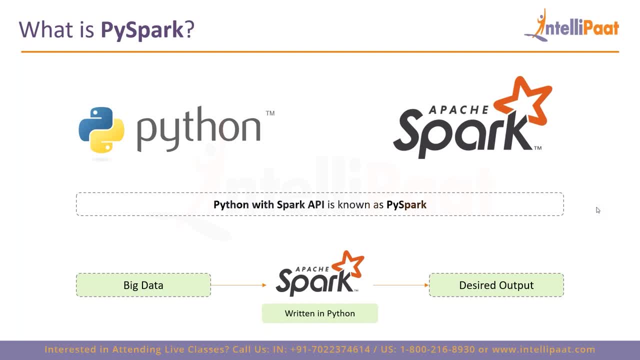 going to be getting into today, but i'll tell you how you can implement spy spark on your own by simply going to a google tool that is there called google collab, and i'll tell you how that happens. it's spark open source. yes, it is open sports. what we are going to be doing today is, uh, we're going. 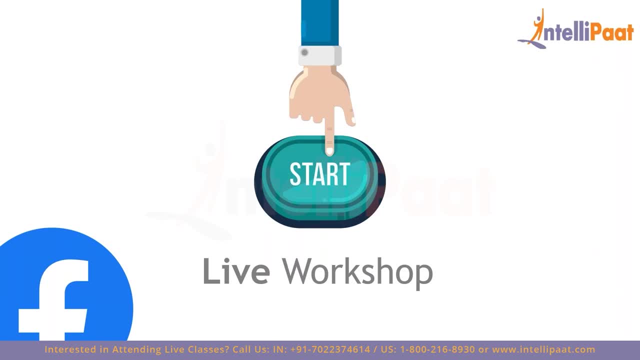 to be analyzing a facebook data set. right, it's not that big of a data set because i obviously i'm not going to be using a lot of data set, but it's a data set that is available on the google service or the google collab right. but when you're dealing with this at an industry level, it is almost the. 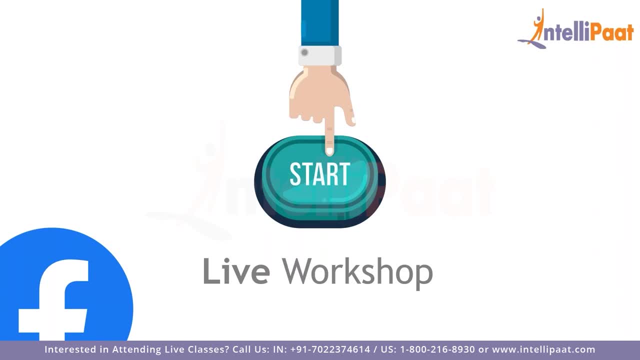 same procedure. you only have to deal with the providing the link to that data, and hadoop manages everything. the hdfs manages everything on its own, so you don't have to really deal with all of the blocks of data. it all it all happens seamlessly. so let's go to the chrome tab that i have open. 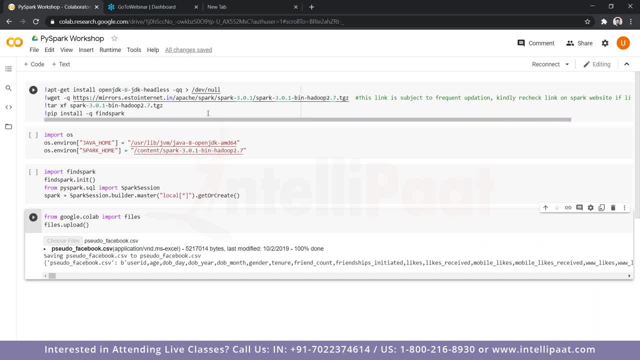 so, uh, i currently have my chrome tab open over here, right, so i have already written some things that are important for me to be able to do as we're just starting this course, but i want to show you some things that are very important to me, so i'm going to show you some of the things. 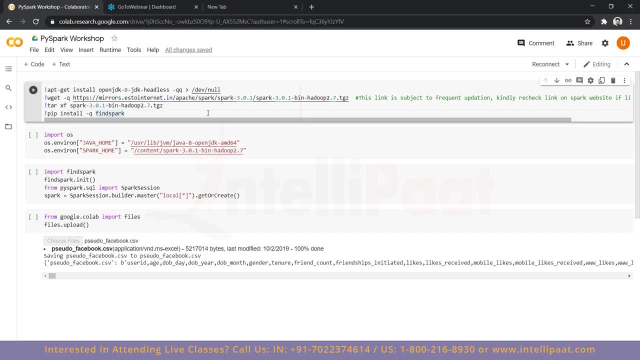 that are important for me to be able to do and they are actually, uh, start up this particular process, right? so if you sign up for the course or something that we have, you'll get access to this particular code, but it's easily available as well online in this particular regard. so the 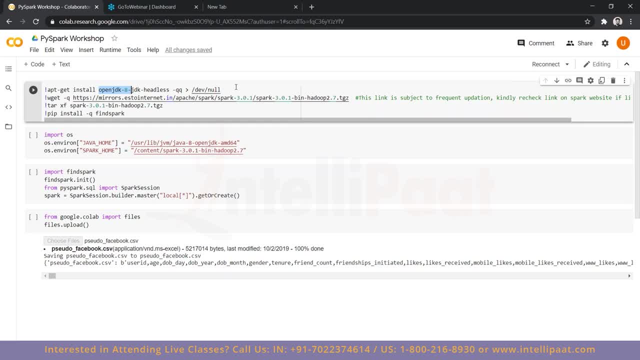 first thing that you obviously need is java 8, right? so java 8 is something that is a prerequisite, uh, for hadoop. so if you're, if you're having hdfs on your system, you need this particular. So you need Java installed. so that is why I've installed Java. 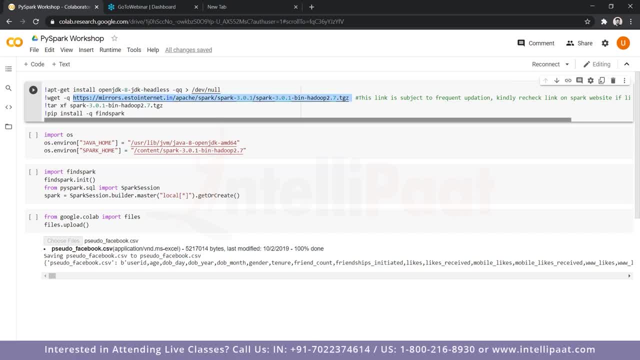 And then I've installed my Spark, my Spark and Hadoop combination over here. So that is the link that keeps changing from time to time depending on the repository- And then I've extracted it and then I've installed Find Spark, which helps us integrate. 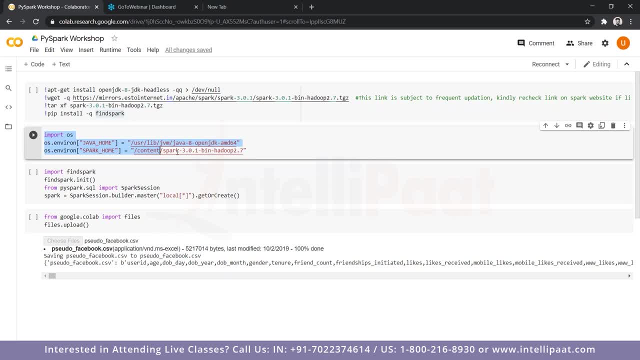 Python with Spark. I've set up some environments for my Java and my Spark so that I'm able to access it, And then I've started with my Python code. So firstly I've imported Find Spark, So we've connected our Python with our Spark by initializing the Find Spark module. 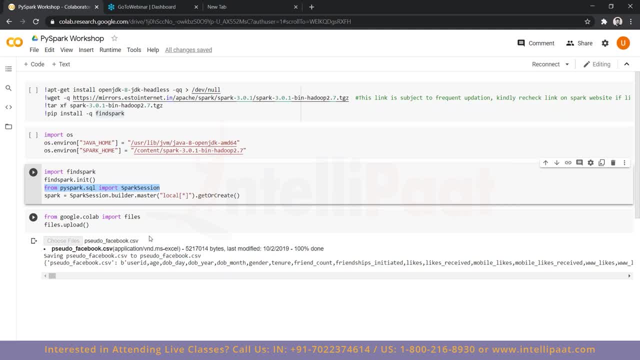 And then I have imported one module that we're going to be needing for our session today, which is the PySparksql module, where we're going to be writing some SQL code within the vicinity of PySpark. So the first thing that I would do is initialize my Spark session, right? 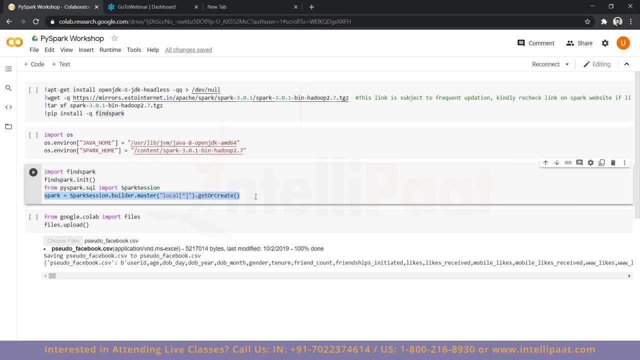 So we need to initialize Spark sessions before we actually use the Spark variable, right? So I'll be able to do that. So I'm going to be uploading my dataset with the Google Colab implementation. So, firstly, I'll play this. I actually have to play this from the start. 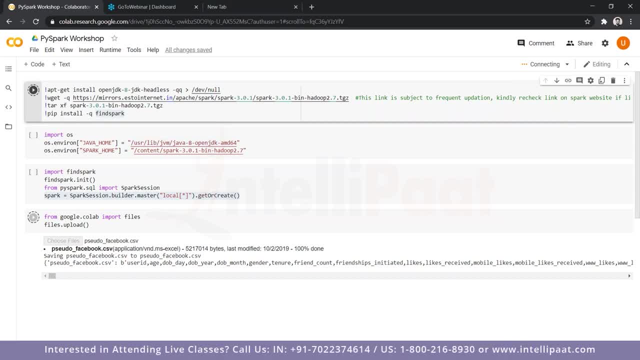 So I'll be playing that, firstly. So it takes some time because it connects to the Google servers, and then we are able to do that. So the website is colabresearchgooglecom. If you go there and type anything, you'll be able to do it. 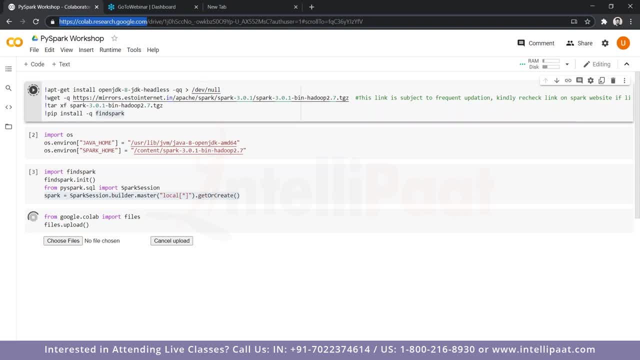 You'll be able to create your own Jupyter notebook. So this is essentially an implementation of the Jupyter notebook that we have. So it takes some time for it to download, and let's wait for that. One question that I'm getting. a pretty interesting question: where are you running this? 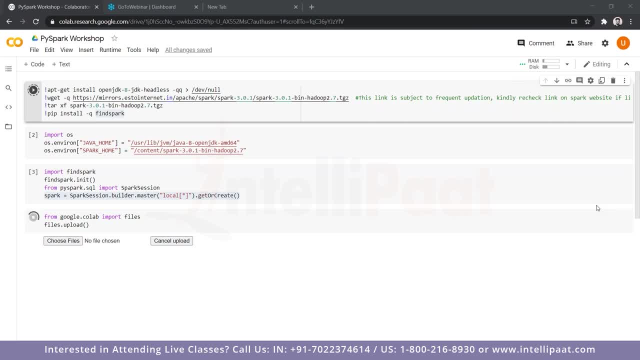 Is this on a Hadoop cluster, So Spark does not need a HDFS storage system to run, but it works. it is compatible with an HDFS storage system. The advantage that you get with Spark: you can use Amazon S3 as storage as well. 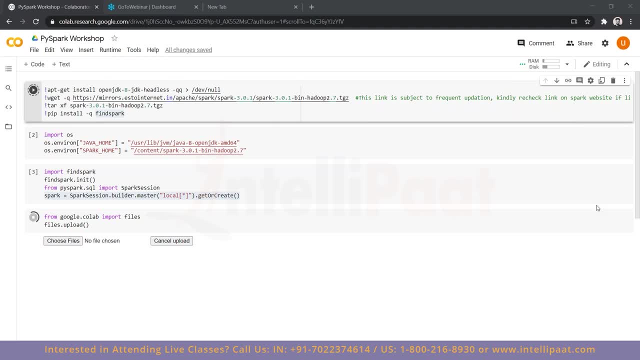 You can use your own file system as storage as well, But if you have HDFS installed onto your system- which we do have when we're dealing with big data clusters- You can also use HDFS with it. So I'll tell you where the difference happens. 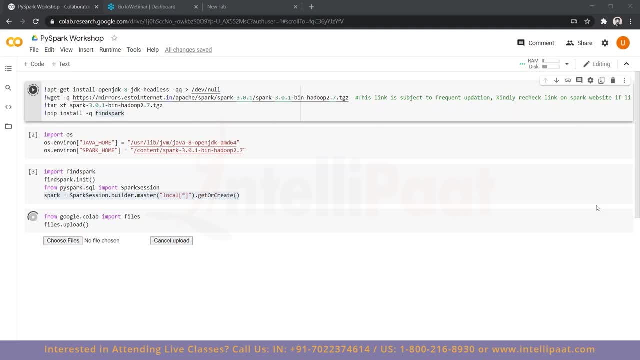 It's not that much. Depending on the link that you have of the file, it'll automatically pick up that file from that location. So whether it's in the HDFS or the actual file system that you have or a Amazon S3 cloud link, it does not matter. 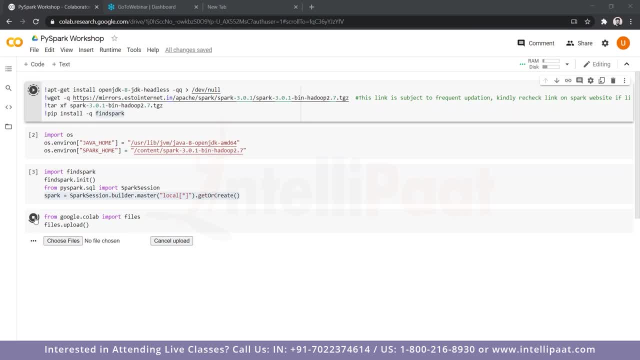 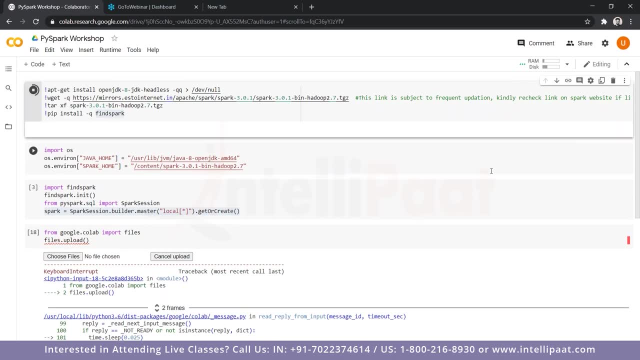 Let me run it. It actually takes some time, So sorry to keep you guys waiting. I'll just pause this one for the time being. All right, So I'll play this. firstly, The problem that you have with Google Colab And specific is that every time you start the notebook again, you have to run the commands. 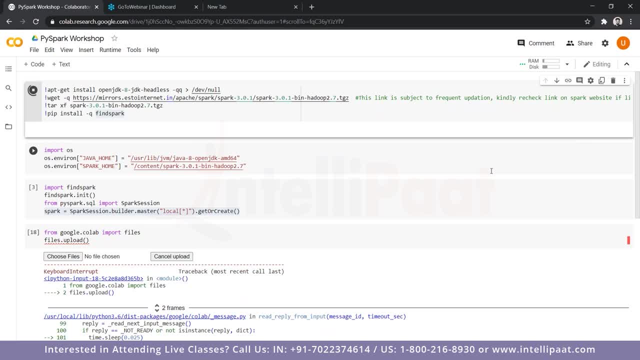 again. So it's not like you are getting access to an already built Linux system. So every time you start Google Colab, you're actually initiating a Linux sort of cloud, right? So you have to install all of these things again. It's good for practice, I would say, but it's not good for actual development purposes. 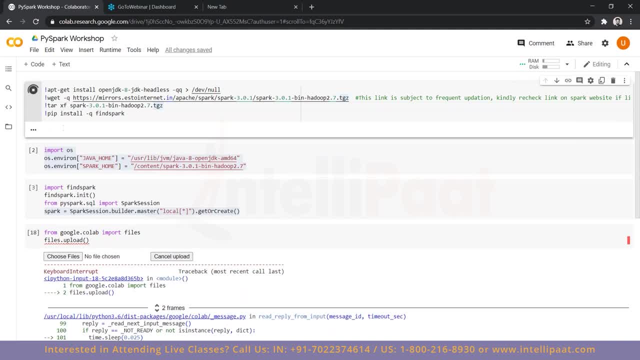 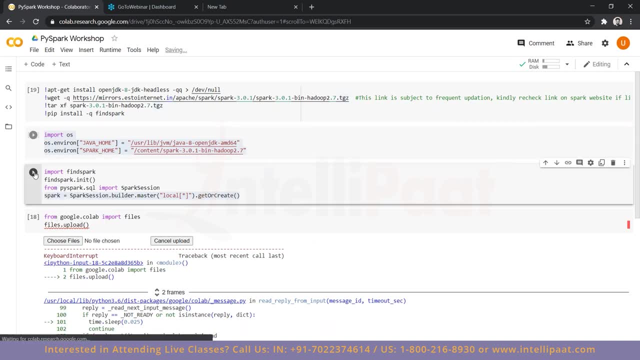 Yeah, so we've successfully run the first block. Now we will set up the environment. This will take no time And we'll initiate the Spark session Right. That will also not take any time. So firstly I'll upload the file. 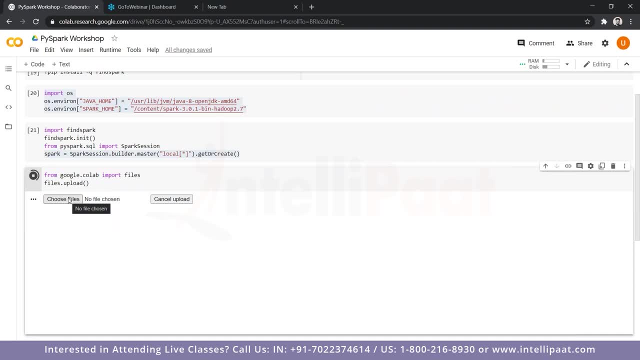 So it asks me an option to when I type files. it asks me an option to select the file that I want. So I want this Facebook dataset, So I click on that, And once I've clicked on that, Google will automatically put it into the drive and then 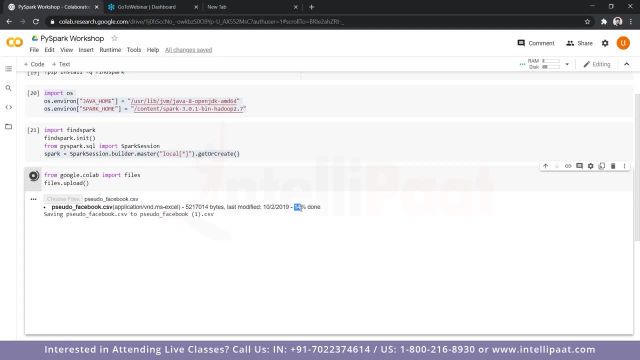 I'll get the access to it. So 12% done. So here you can see the percentage. So is this building a Spark cluster for you? No, it's not. actually There's not a cluster involved, It's a single node cluster, if you may speak. 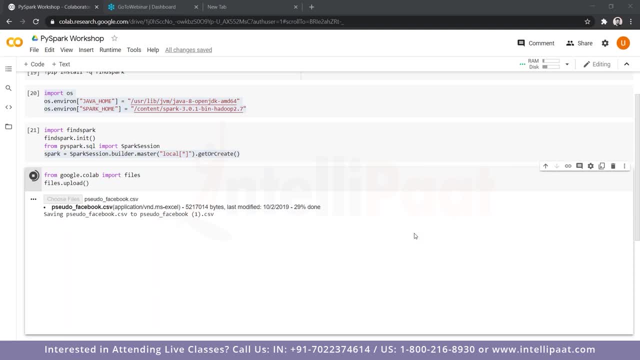 So, if you, it's basically like you're installing Spark on one system and it's emulating the cluster, Because I'm not actually dealing with actual big data, where we have terabytes to petabytes of data, So it's not actually going to cause us any performance issues. 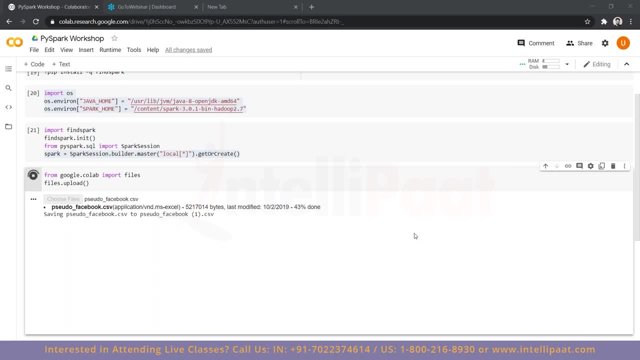 But we're dealing with a single node, Spark cluster. If you add multiple nodes and we have Spark installed on multiple nodes together with the HDFS underlying storage system, we could have used it in multiple systems as well. So 59% done. It takes some time. 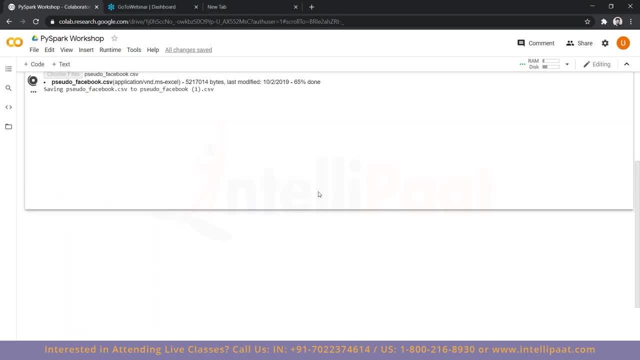 Let us finish with that. So meanwhile I can write some other code as well on the bottom. So we'll just go ahead and do that just a moment. Yeah, So firstly, while this is uploading, let me type in some code. 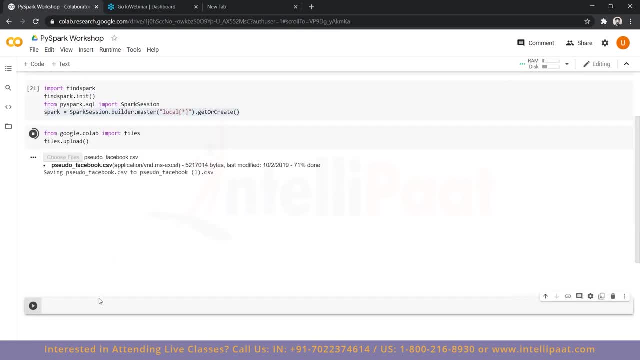 Right. Meanwhile, any doubts if you guys have, you guys can ask regarding this technology or what we're doing right now. So, generally, what you get with the big data is Mark. if you're dealing with organizations, right, Organizations obviously want to boost their businesses and and, and, and, and, and and. 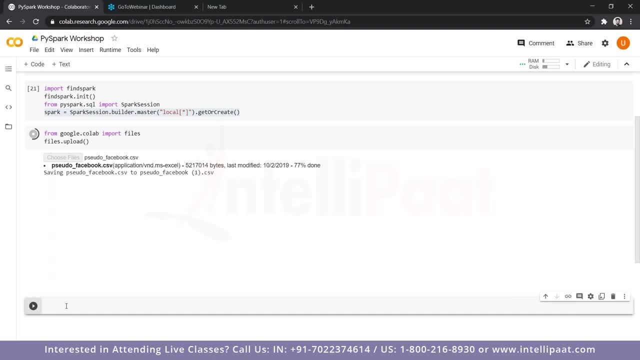 the way to boost their businesses is through marketing, So the marketing is the number one thing. that actually is the success key for businesses, Right? So a lot of these organizations are online, like Amazon. like Amazon, Right Yeah, Like Google. 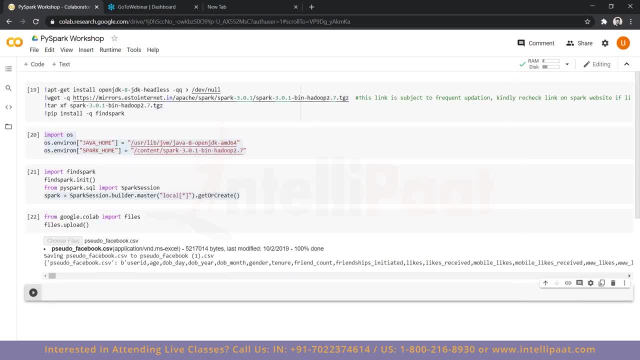 And they have large user basis, like enormous user basis, And all of these users have data sets. they're generating data almost on a day to day basis. So if you go on Amazon, Amazon knows what you like. Amazon has idea about how many stars you've given to a product. 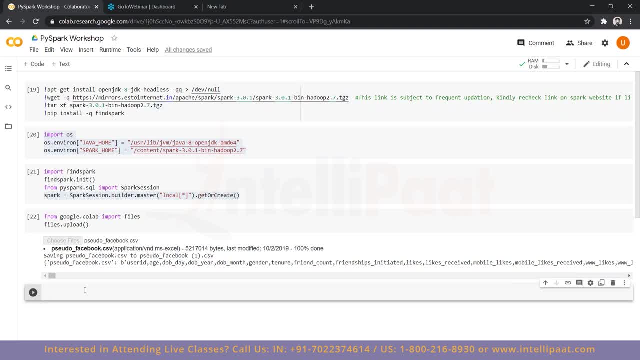 So all of that data Amazon has. So what Amazon will do is give you, give that data to the big data analysts and the big data analysts will basically answer some questions, find some information out of that data And they will give that, visualize that data or basically summarize or document that data. 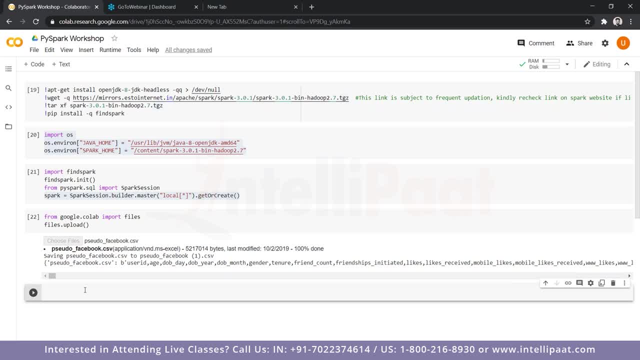 and give it to the marketing team, And then the marketing team or the sales team can make their pitch based on it or make their marketing strategy based on it to maximize profits. Right, If you're dealing with a data science team, you can forward that information to the data. 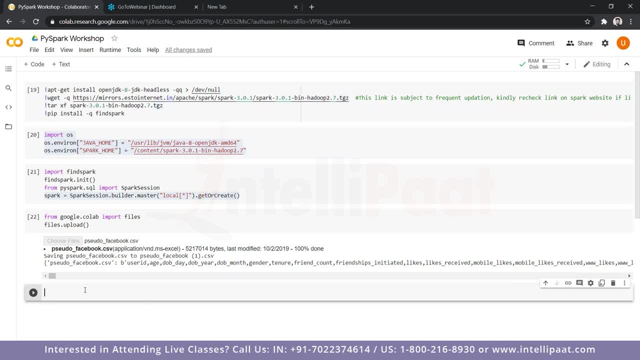 science team, the data science team and the machine learning team can implement models based on that data to be able to create recommendation engines and properly recommend the customer. Know what the customer likes, right? So that is. that is how all of that works. 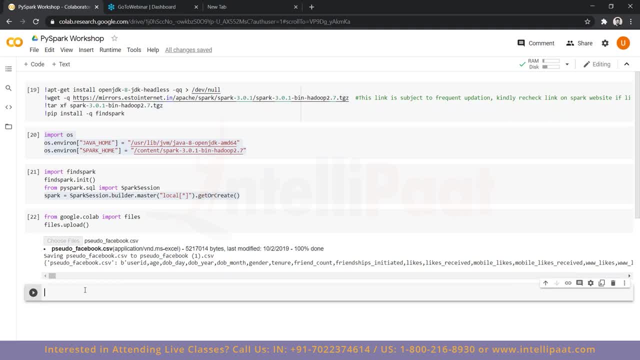 So, firstly, we'll create the data frame out of this data, a data set. So DF is what we'll call the data frame, and it's it's like a Python variable. DF will like be like a Python object. DF equals to sparkreadformat. 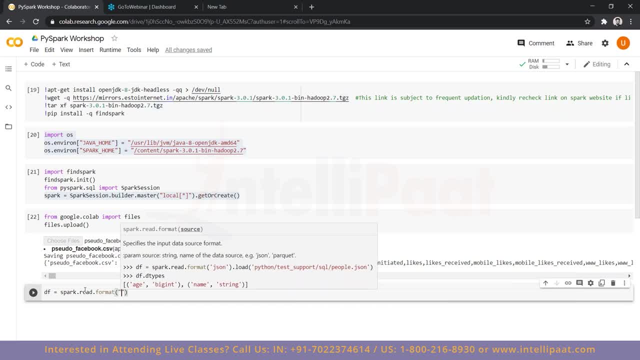 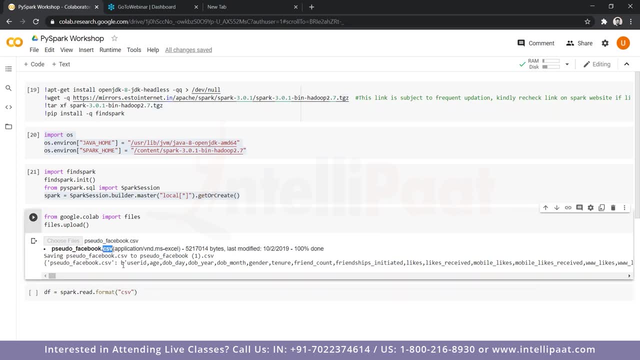 So we'll specify the format that we actually want our file to be. So currently, what we're importing is a CSV file, Right? And we want to include the headers, because the data set that we are dealing with has headers. So the first row of the data set is the header name, and we'll put it to true. 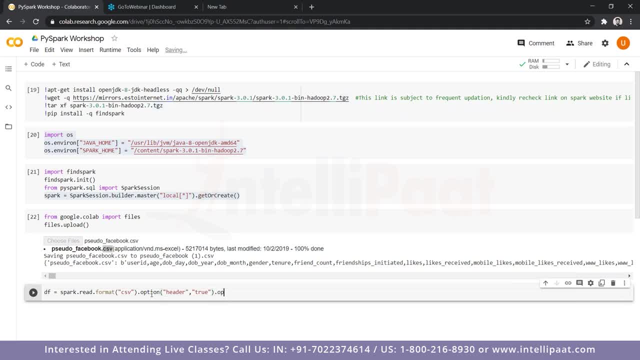 So the header status is true. Yes, We want to include the headers option and first schema, So input schema, and then we put it to true. What it will do is it will automatically detect The data types of the values, So it will create columns based on those data types. 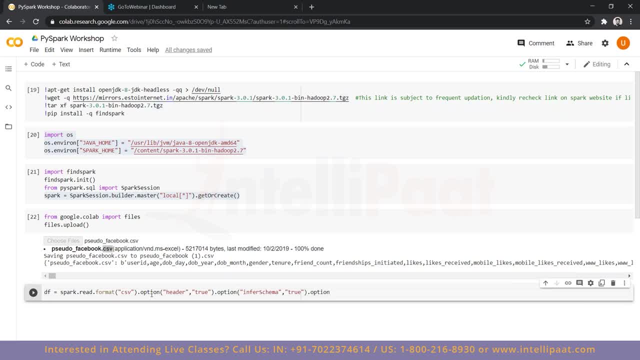 So if it's a numeric one- two, three, four- column- then it'll assign an integer to it, And if it's a name based columns- a name based column- then it'll assign string to it. So the next thing that we'll do is a mode will be fail fast. 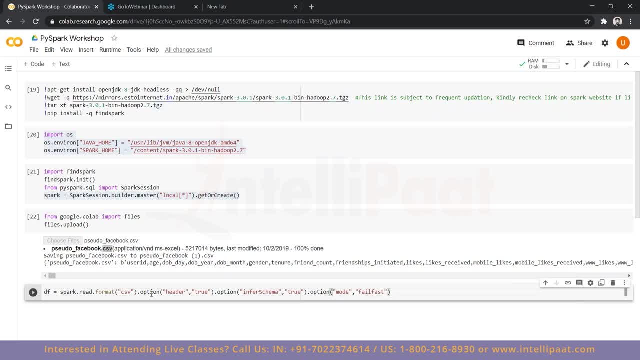 So if there are any exceptions, it will automatically be detected and then load. Then, finally, this is the part of what I was telling earlier on That no matter where you have your data, you'll simply put in the location here. So if you have data presented- the HDFS, you'll do something like this and, given the location, 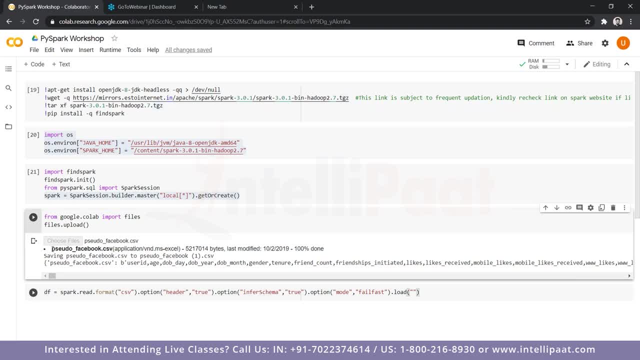 if you have data present in the in the directory- the present working directory- then you're simply given the file name. So I'll copy the file name, put it over here So, and then I'll click on play. So when that place starts executing, we'll have our data in our location, right? 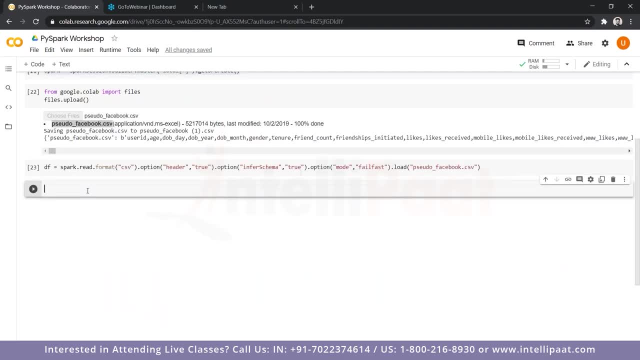 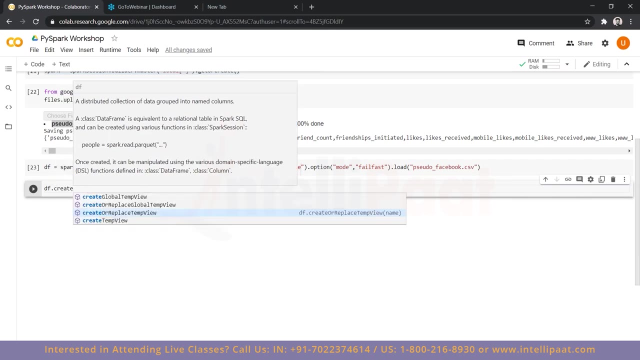 So just to confirm, uh, first thing that I'll do is actually create a temporary view out of this data and put this data frame and the spark SQL context right. So first thing that I'll do over here is type in: um what was it? create or replace temp. 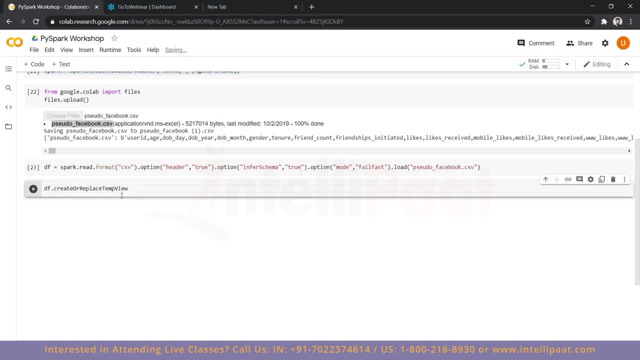 view right. So the other advantage that you get with using Python is also get this auto recommendation thing right. You can get all of the details of that particular uh uh function that you're using. That is not the case. that is possible when you're using Scala, sort of a command line. 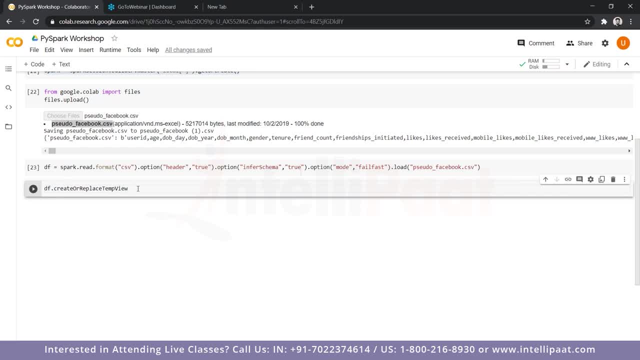 libraries, right. So if you're using this from the command line, it will be a lot difficult for you. If there is any error on anything, I'll assign the name. um, let us call this FB, because FB is short for Facebook, and we'll click on pay. 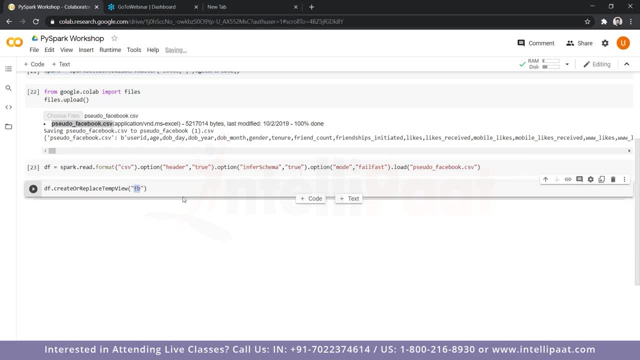 So what will essentially happen now? uh, this FB name is what we are going to be referring to- DF- in the spark SQL context. So spark will create a virtual SQL environment. right, A virtual SQL environment means that there's not an actual database that we have installed. 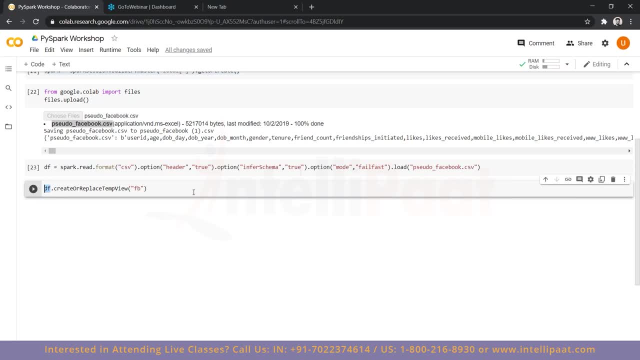 We don't have a minus, We don't have an actual database, but spark will mimic in SQL environment. It has created a virtual environment in which this data frame is going to be considered as an SQL table. So that is what we are calling this virtual table, as like FB. 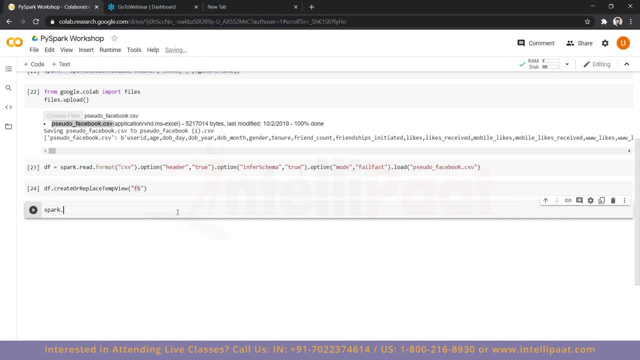 So cold. uh, let us see how this looks. Spark dot SQL is simply after: type that and type in the normal SQL statements, select asterisk from the table name that we've just signed it FB and put it in a dot Sure. 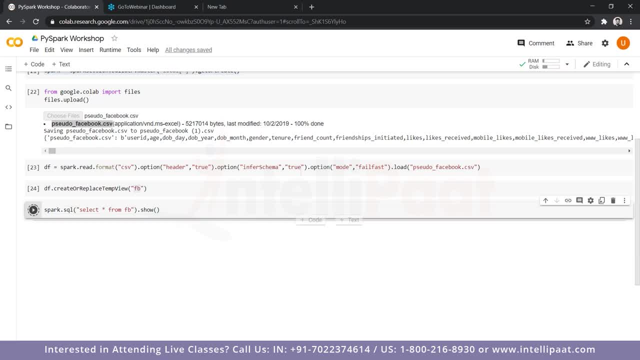 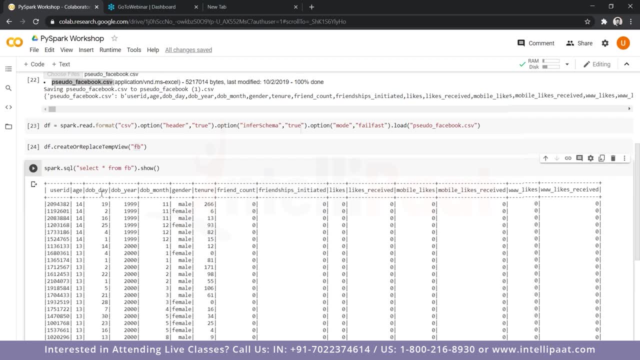 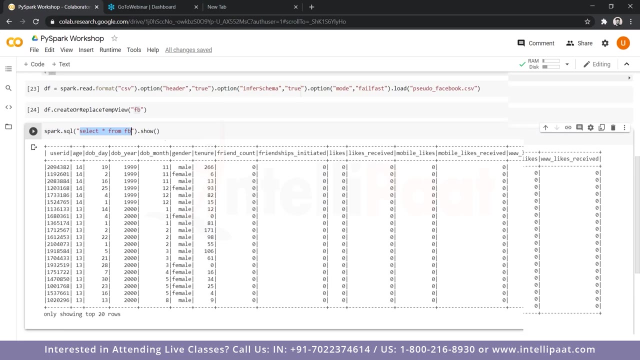 And then we click on play, uh, it'll actually give us the data set, as we can see, Right, Um. so keep in mind that, uh, this is something really convenient If you're coming from a database management background, right, you can see, uh, these. 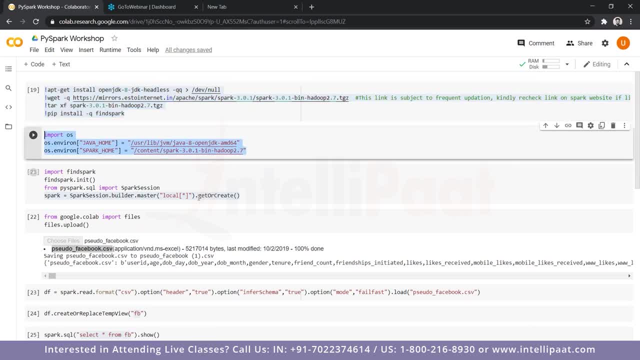 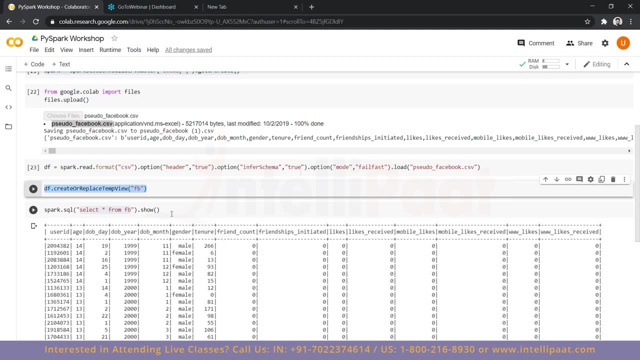 are the only new commands that you essentially have to deal with. a little bit of Python And, after you've done the steps until here, if you're using simply spark SQL, if you're not using any sort of complex Python, This is how easily you can get started with big data. 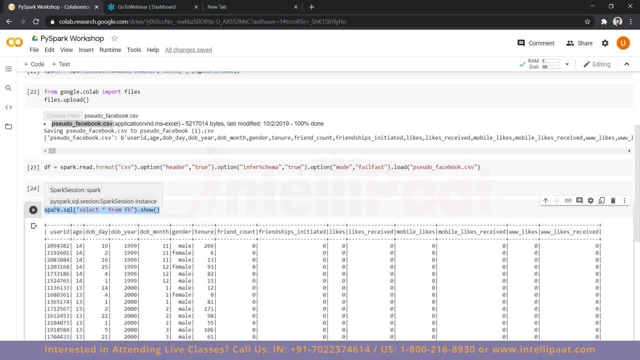 So we're coming from an RDBMS background and if you want to deal with data that is of enormous size right And your SQL skills are really good, You can get ahead and basically create your career out of this right. You can create a career in big data analysis as well, and then you can expand upon it with 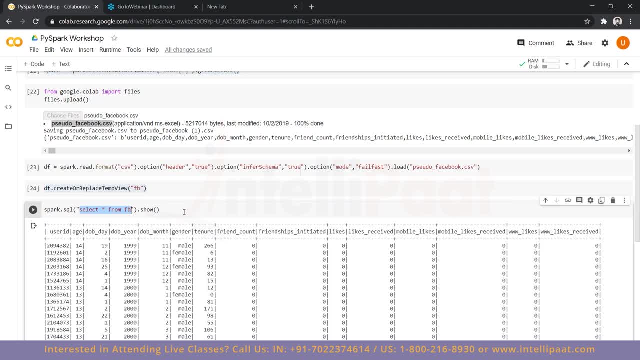 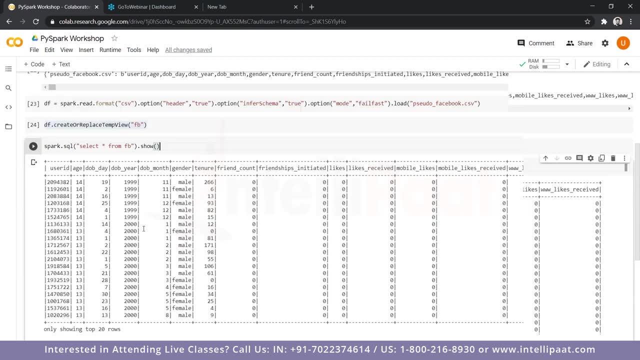 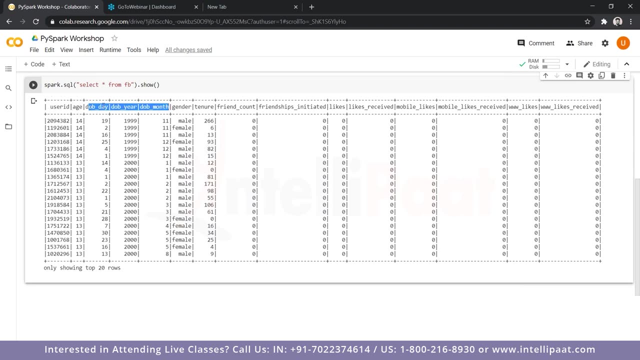 other knowledge as well as you move ahead with Python, with Scala or any other technology, you've chosen to start your SQL, Spark SQL career with Right. So we've done that and we can see that there's user ID. So the unique primary key number, the age of the Facebook user, the date of birth, the 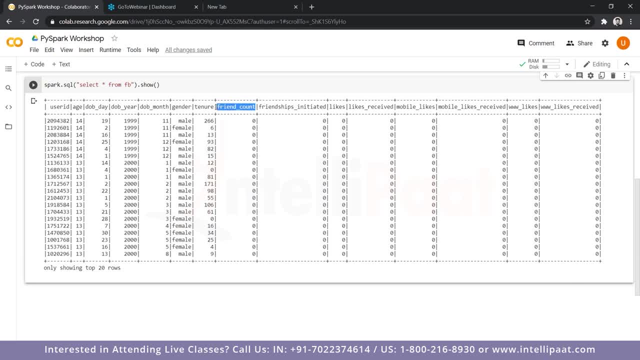 gender, how many days the person has been on Facebook. the friends count that the person has, the friendships that the person has initiated. That means the number of friend requests that the person has sent, the number of likes that the person has. I mean the person has given to other people, the number of likes that the person has received. 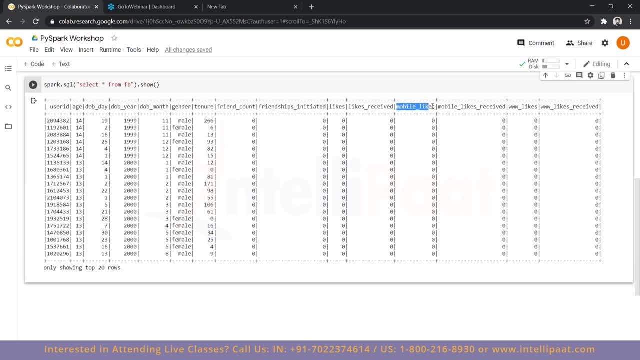 And this, this particular number of likes, Has been divided into mobile likes. So the number of that that has been done with mobile phone applications and the number of that that has been done with web browser applications like Google Chrome or Mozilla Firefox, 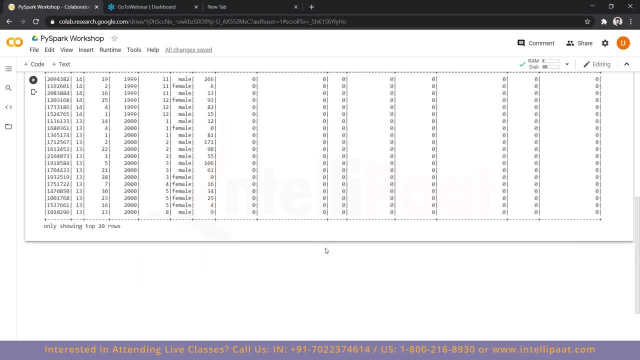 Right, So that is also accounted for Right. So let us do some analysis with this data now that we know what the column names are, So it's quite simple to do that as well. Firstly, uh, let us evaluate the average age of Facebook users. 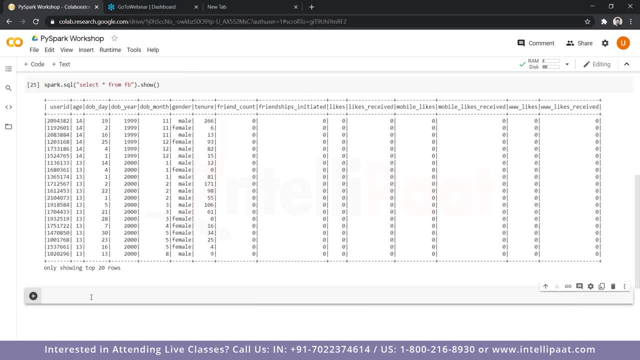 Okay, So the average age of a person on Facebook, right? So what you'll do for that is- or we could- just the first thing that we could do definitely is type in sparksql and, uh, open up an inverted comma and pass our SQL query: select count. 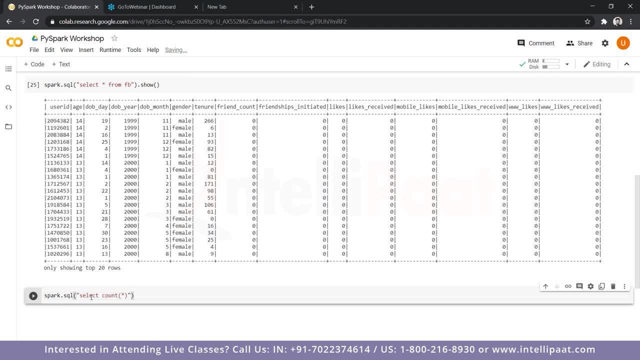 and given an asterisk over there. So this asterisk means we're using all columns, all columns and FB. So when we do that and we type in dot show and we click on play, so it will give us all of the the count of the columns. 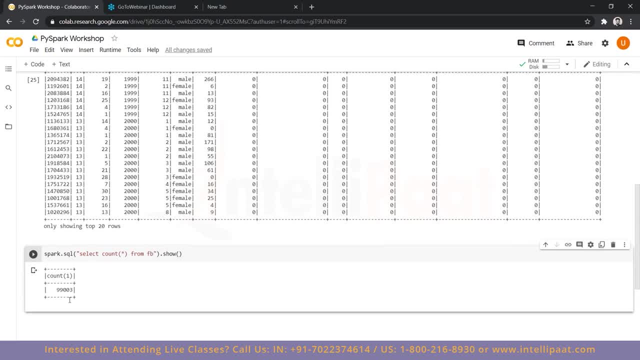 Uh, count of the rules that are there. So there are about 99,003 records and this particular database, right? Um? so this particular uh advantage that you get with this is: uh, you can simply write dot show as a Python function and you'll get your answer. 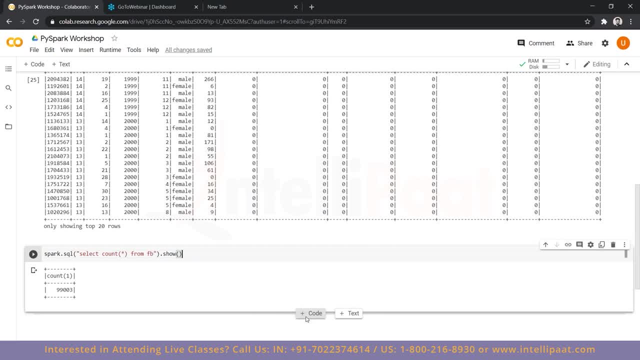 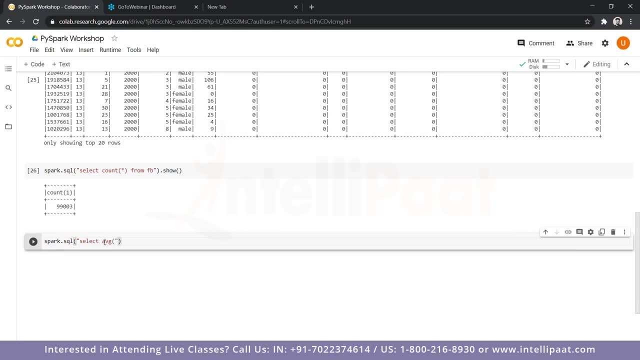 Right, Uh, there are other things that you can do. this do with this as well. If we go with a spark or SQL and given another query like select average, and uh, we didn't, we didn't even a column name. 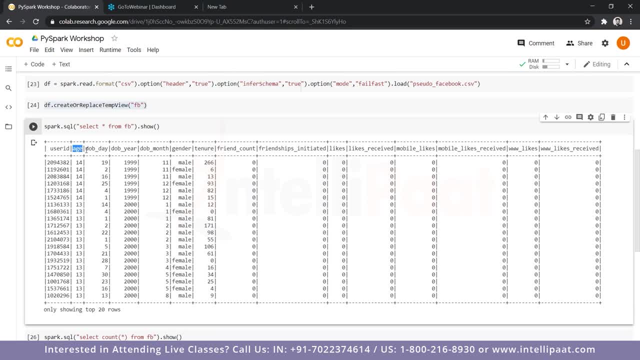 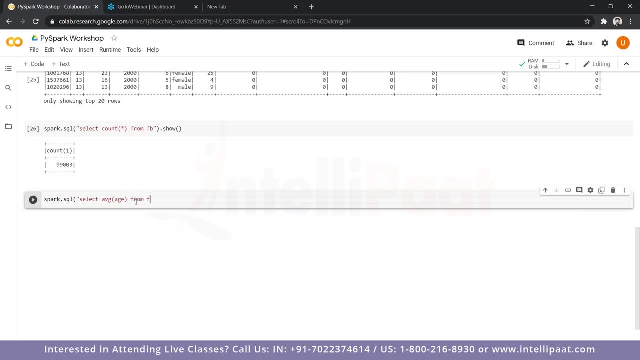 So, for instance, If we want to go with age, we want to find out the average age of a person on Facebook will type an age over there in the average section And from FB we put in that and we close this up and type in dot show it. do that. 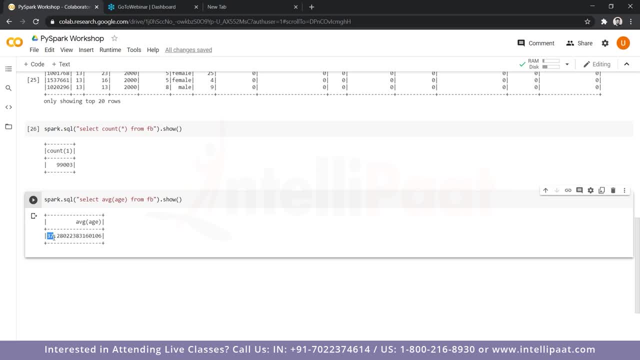 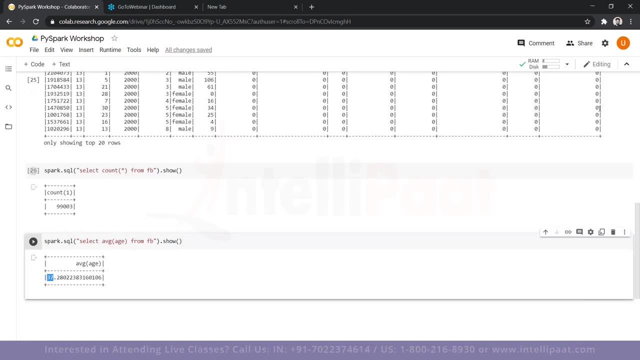 And we click on play. So it gives us the average age is about 37. So the current average age for an individual on FB, based on this limited data set that we have, is about 37. So I think it gives us a right, rough estimate, right. 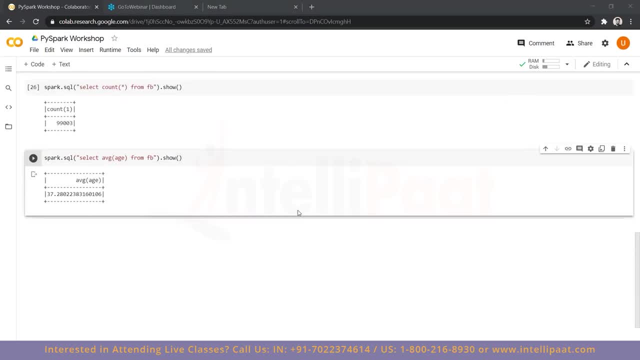 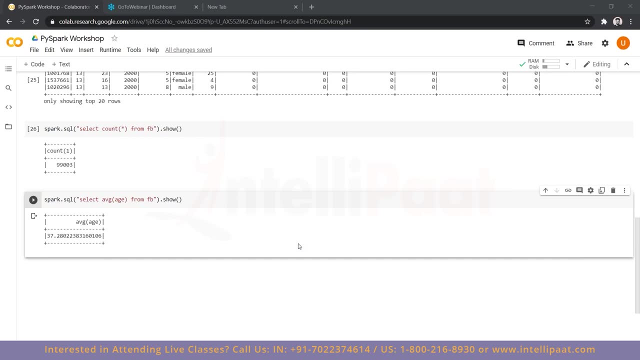 So uh say, for instance, the marketing team wanted that question out of you. Now they have it. So the advantage of running this with spark is that, no matter the size of the data set, uh, whether it's in terabytes, and there are billions and billions of records- you can. 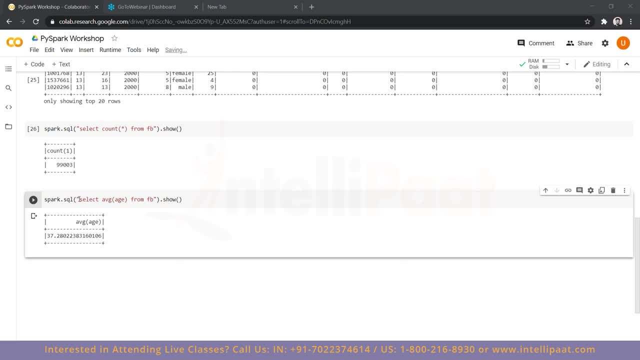 do it pretty easily, very easily, for this matter. it can happen really fast if the cluster is big, uh, and the processing is happening in parallel on different nodes. This will happen in almost the same time as it happened for me over here. 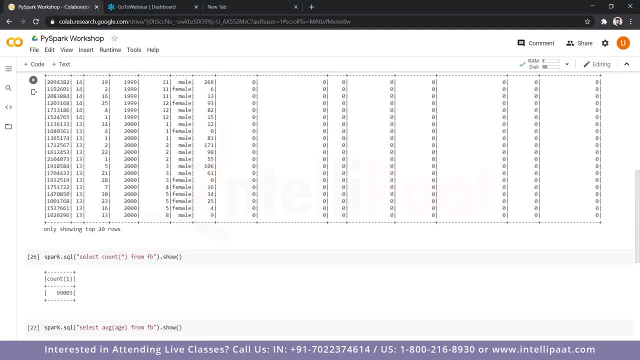 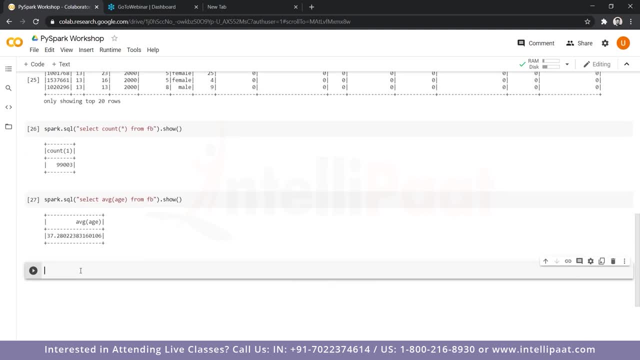 So go on another And we can do something else. Okay, We can do some creative things with it. Uh, we can also find out the account of males and females and basically, uh, uh, do this average age thing as sort of a male- female thing. 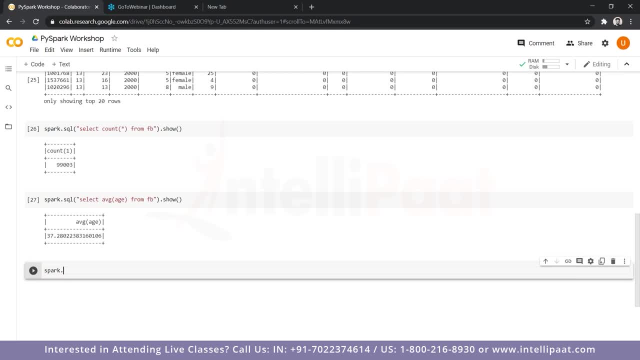 So let us try that: Um spark dot SQL select um average age. So once we've selected, uh, average age, uh, we also want something Okay That we are going to group this column on. so we want to group this by gender, right? 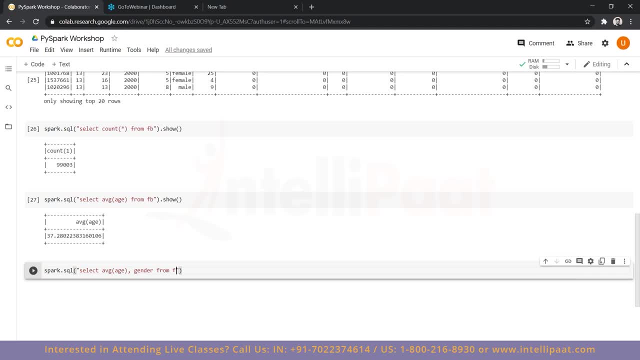 So once we uh include that column name and we type in from FB- so this is basic SQL, by the way- and type in group by gender, When we do that and type in what show over here, click on play. So it will categorize the average ages by gender. 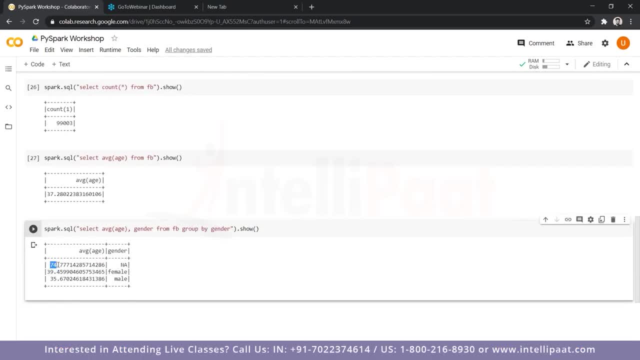 Right. So for the gender that is not disclosed, we have 74.. Okay, For female we have 39 and for male we have 35. So it's double value. It's a double value, by the way, right now, but uh, that is because it's actually calculating. 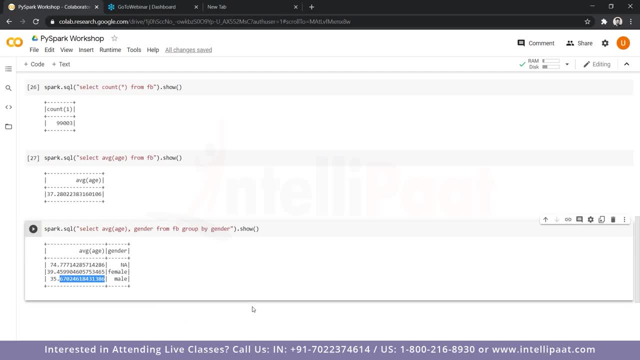 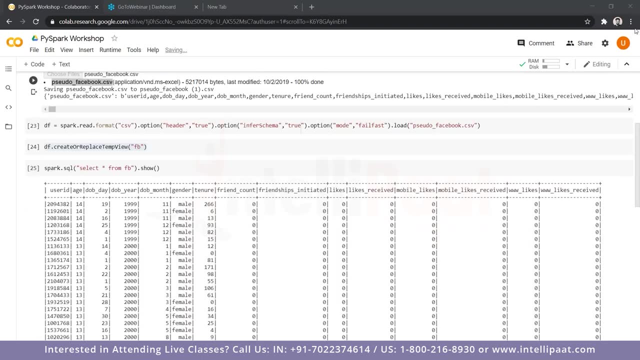 average, and average, by default, is calculated, calculated in double. So that is there, So the next thing that we can do something more creative with it. by the way, you guys can ask some doubts, uh, any doubts that you guys have, uh, then I can continue. 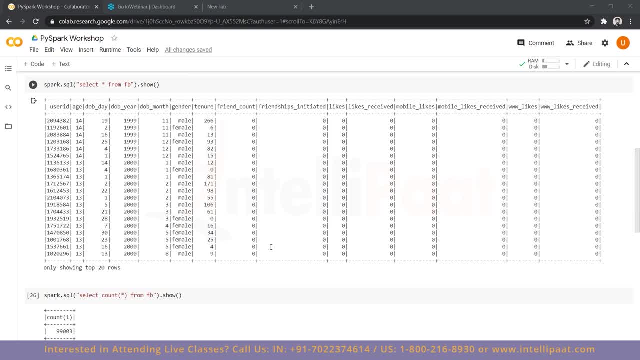 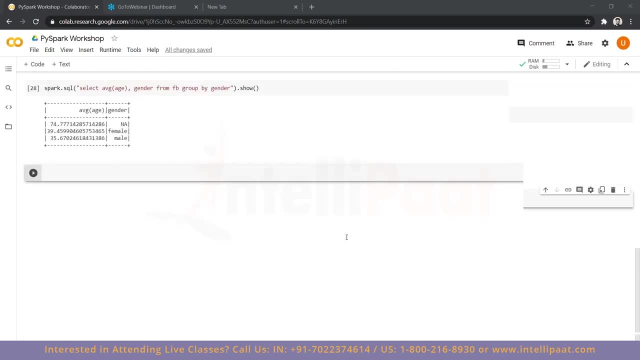 So I'll wait for like 10 seconds and then continue. If you guys have any doubts, Right, I'll return the questions box, All right? So, uh, there is one doubt. Um, so the doubt that I'm getting is: uh, how does Spark operate in a battle? 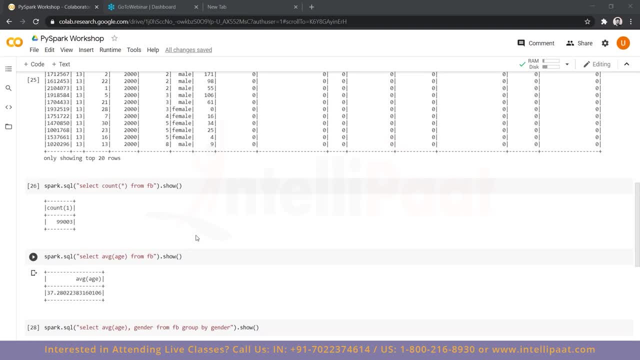 So a Spark actually operates quite simply at battle uh, similar to MapReduce. you're actually installing Spark on all of the devices that are present in your big data cluster, similar to how you would install Hadoop. So say, for instance, you have HDFS already installed- uh on all of the devices. 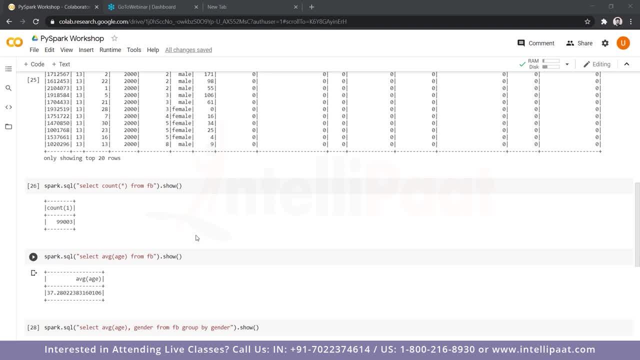 So it's already Hadoop? uh, the Hadoop cluster has already been created. Now your administrating team will come in and they will install Spark on each of these systems, Right? So when you go ahead and like over here when I created this particular data frame, right? 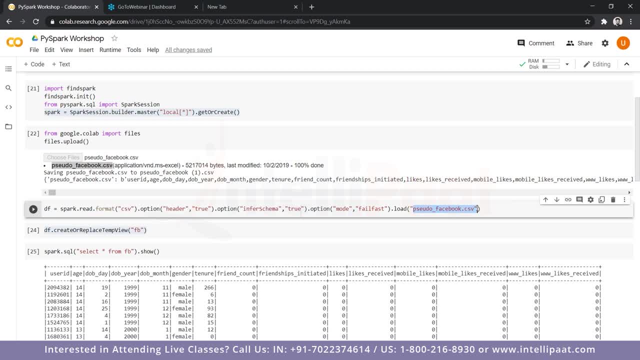 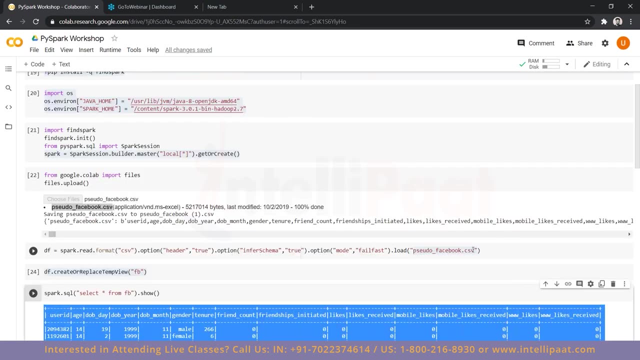 And I specified an HDFS address, right? So whenever I specify the HDFS address, it will automatically take all of the blocks that are present across all of the nodes. Okay, So we have a combined view over here, right? So we don't need to concern ourselves with block one, block two, block three, block four. 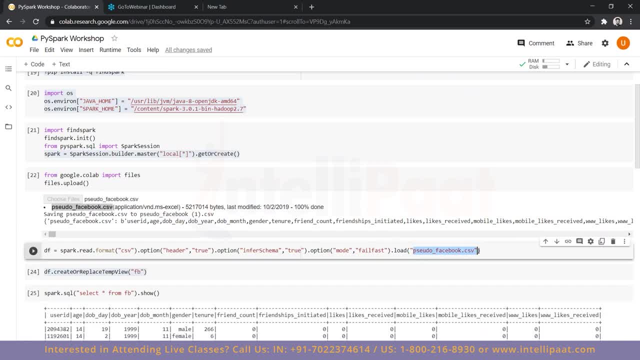 so on. When we give in the file name right, it'll automatically go to the name node understand where all of the parts of the files exist. It'll import that file in the data frame. We don't have to deal with any of the complications. 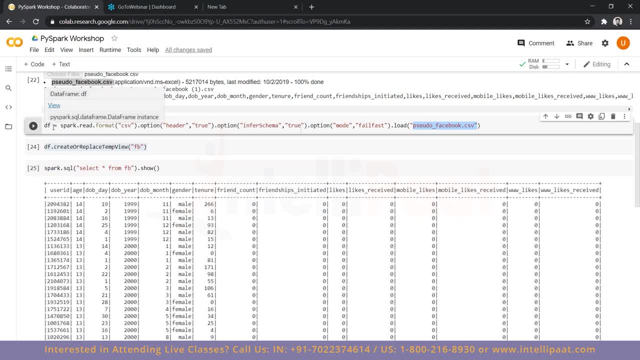 We just have to store the file on the HDFS and we have to import the file using Spark. So that is how easy it is. Will any changes made through Spark Be reflected in the original database? No, So this is the advantage with Spark SQL. 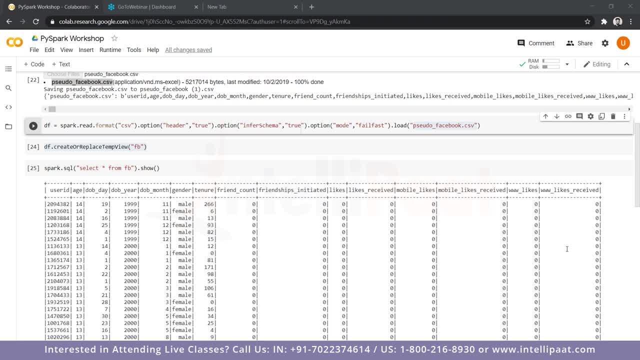 You're essentially housing this entire data set in your RAM, right? So this is a temporary view of that data set. So here you can make changes, but you can create a new file with it, right? Or you can overwrite the existing file that you have, right. 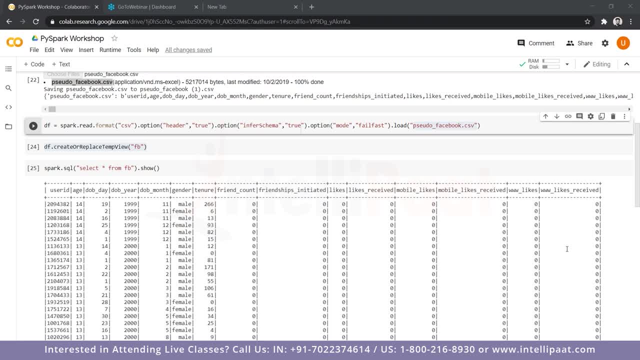 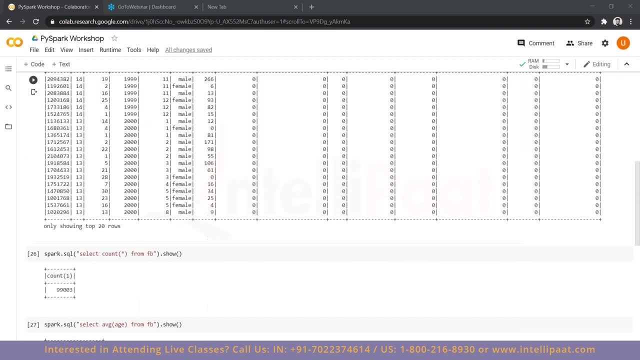 But it's not necessary that any changes that you would create, any data frame changes that you would create, will be reflected on there. Okay, It's reflected on the original data frame. In fact, these things, these particular data frames that you create, this PDF is immutable. 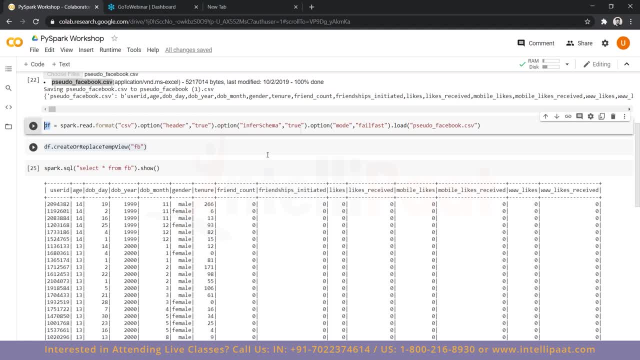 in nature. So immutable means anything that you want to change to this data frame as well. even in the RAM right, You will have to create a new data frame out of it. So say, if I wanted to alter the value of 106 to something else, you would have to create. 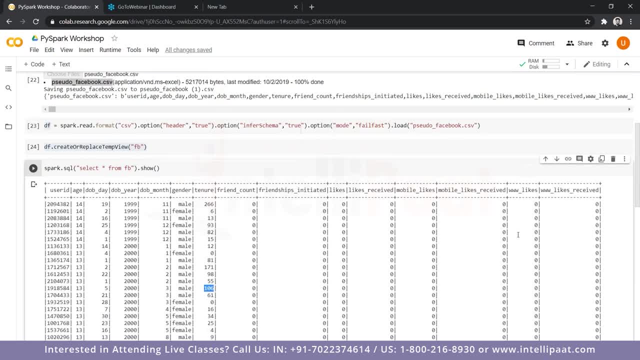 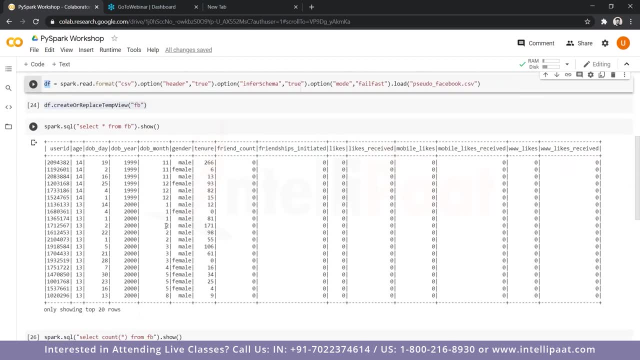 a sort of new data frame for it, right? If you wanted to add a new column to it or remove one column from it, you have to create something like DF2, right? So the way we manage that in Spark if you want to create new columns in it- is firstly: 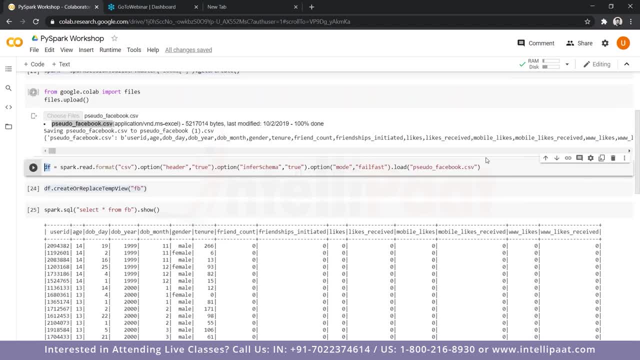 we'll create a new column out of the existing column And then we'll use garbage collection to remove this column, so that we are not actually over our RAM limit or we're not actually overusing our memory right. So let's continue with that. 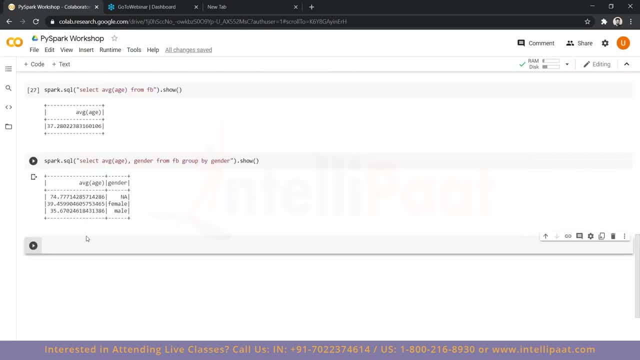 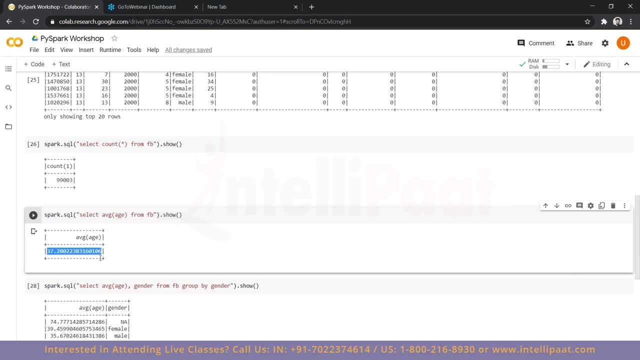 What else was I talking about? Yeah, So now let's see, This can be integrated with Python pretty easily. So say, right, here we had the average value like 37, right, What if we didn't want to see this like in our table format? 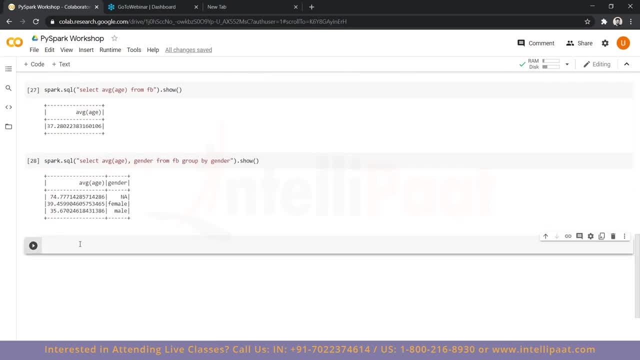 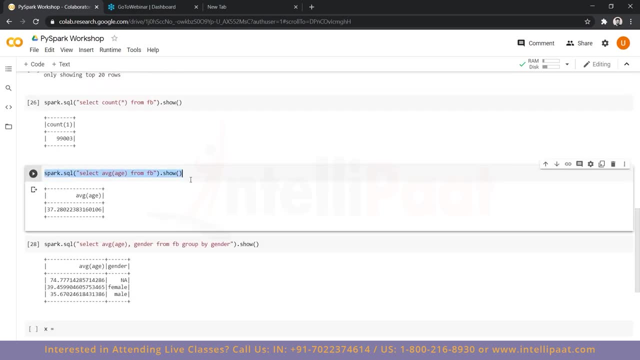 What if we wanted to store it in a Python variable? That is quite easy as well. So say, our variable name is X, right, And we want to basically have this data stored in that variable so that we can do further Python for Python operations with it, right? 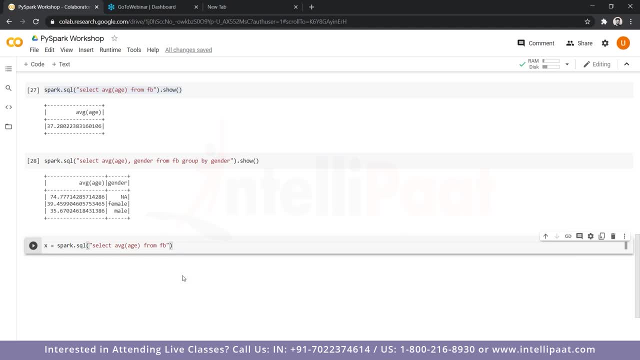 So we do that. We remove the show because we don't actually want to show it over here. The thing that we will do is type in garbage collection, Right. We type in dot collect And then, since this is a table value, this is a table value, right. 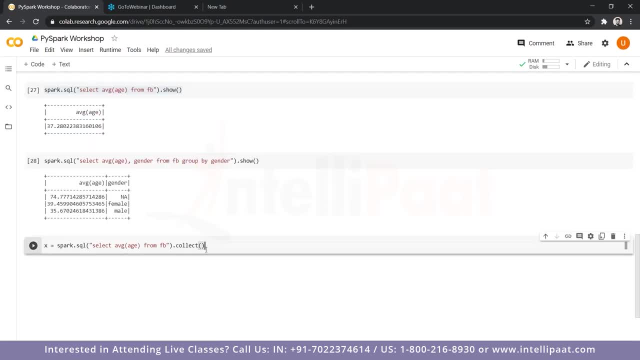 So this comes automatically in the form of an array, right? So we cannot actually collect it in a single sort of X and expect to see the value as a singular value, So we'll treat it as a two dimensional array. So anything, any, any SQL table that you will have in life is sort of a two dimensional. 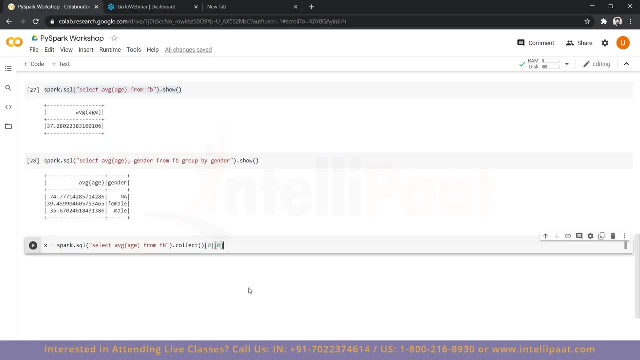 array, So the first would be zero and the second would be zero as well. So you're essentially taking the first value, Zero, zero position value, right And that when you do that and you click on play, it executes without any issue. 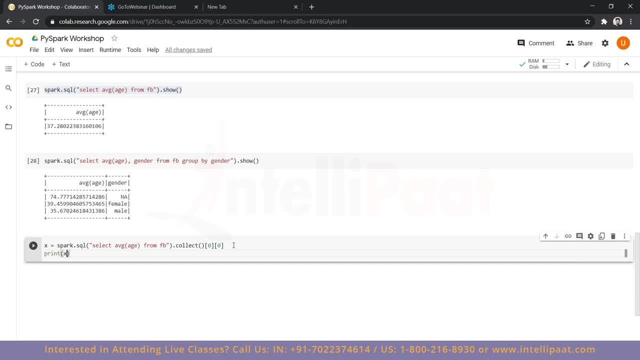 And when we click on print, say, for instance, X plus two right- So when we do that and click on play, so instead of getting 37 and this, you get 39. So I hope that is pretty clear as well. 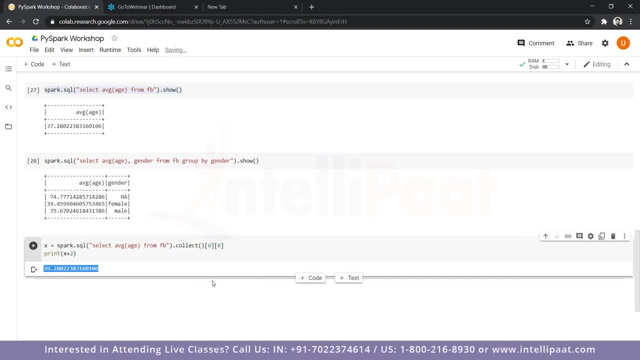 So if this is a similar to Pandas, the one question that I'm getting is: is this similar to Ponder CF? Yes, This is similar. Quite simple, Right. There's not a difference between that and Ponder CF are also immutable data frames. 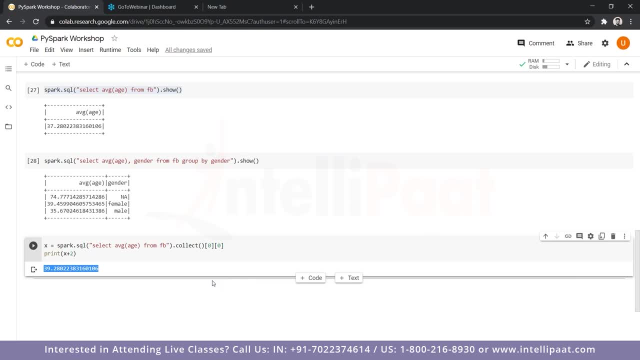 They cannot be updated as well. So whenever you're updating a Ponder CF, you're actually also creating a new DF, So yeah, it's in here. when you're dealing with Spark SQL, you're actually. this particular thing is considered as a Python object and you can do anything with it. 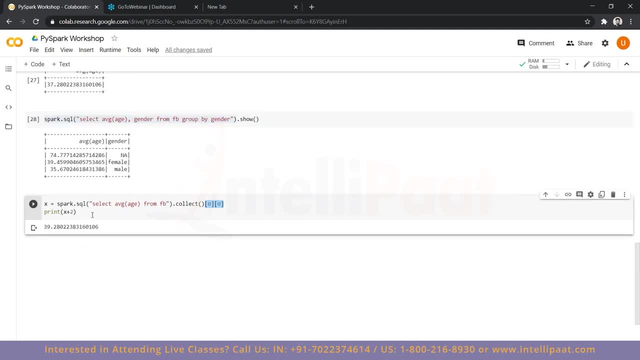 So here we referenced it as an array and we collected the value, and we can do anything else with it as well, Since this comes in handy. the collect function comes in handy when we are trying to integrate different Python modules with it, so that we can take that data from Spark SQL and actually 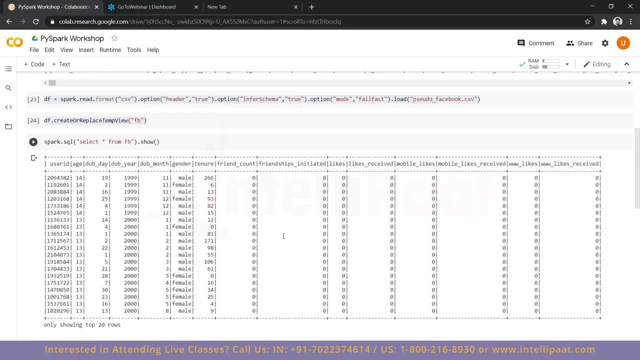 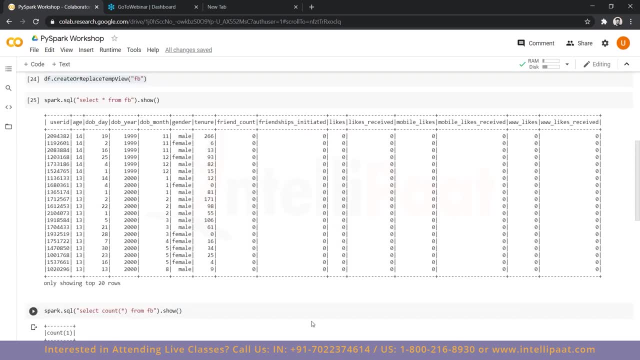 implement something with it. So let us do something else with this as well. All right, We'll now continue. So the next thing that we can do is say, for instance: we can find the likes received at an average for a female and a male right. 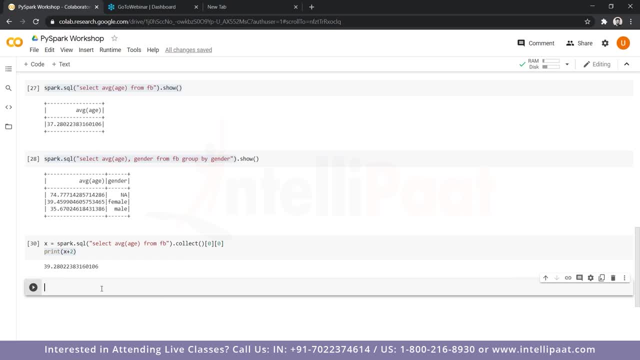 So that is something that is quite interesting as just curiosity point. at an average, What are the likes? Okay, So what gender received the most? receives the most likes on Facebook? So these are the sort of interesting questions that you're going to answer for your marketing. 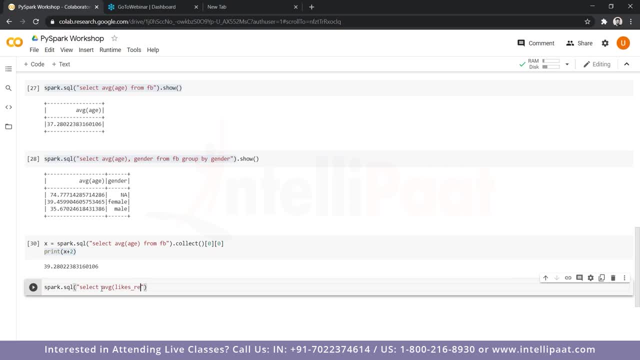 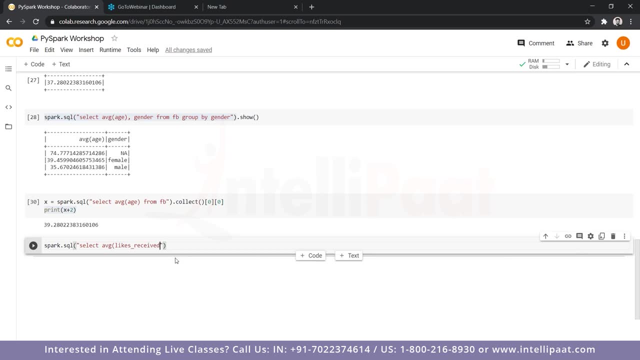 team or your sales team. So average likes underscore received. I think we're correct with the spelling E. I always make sure I don't mess that up- and average likes received. And then we copy gender over there from FB and we can. what we can do now is something. 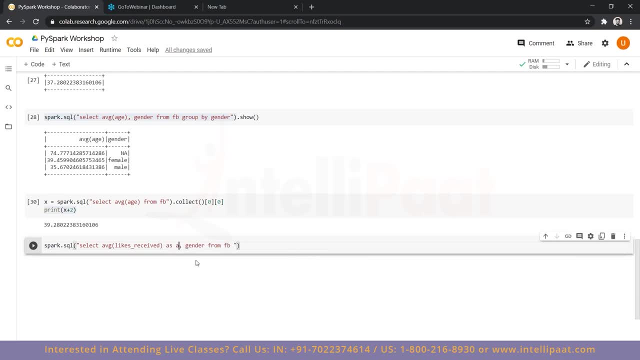 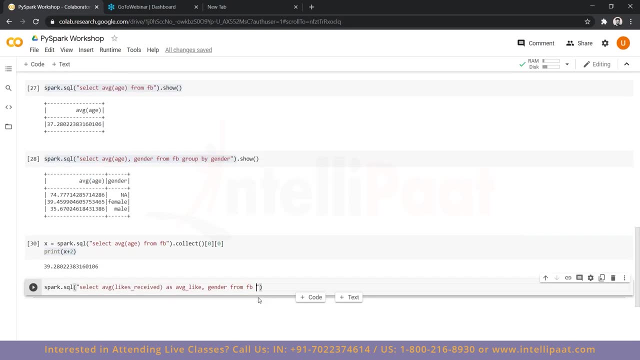 like. I can provide an alias to this so we can call it average like right, So I can refer to it as average like instead of something like average age, and then we can do a group by gender and an order by average like right. 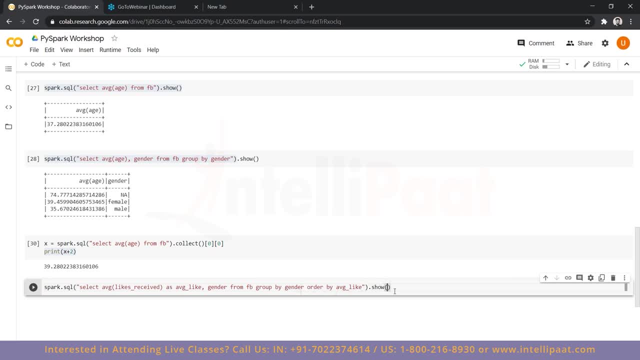 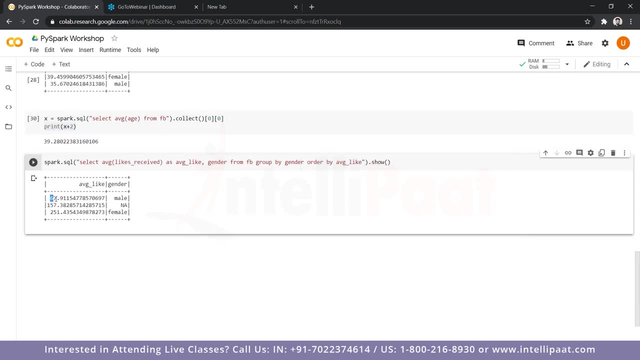 So what this will do is it will also grouping, it'll do the grouping and it also do the sorting. So it will be sorted in ascending order and click on play. So firstly we have the minimum average, Okay, And then we have the average like. so that is 67, that is for male, for non-disclosed genders. 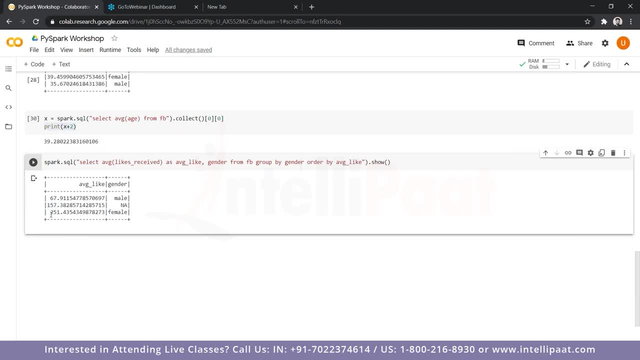 We have 157 for female. We have the average like of 250 months. So gives us some demographic data right. So we get that data out of this. We understand how gender dynamics work on Facebook. What sort of the behavioral personalities of people are on Facebook? 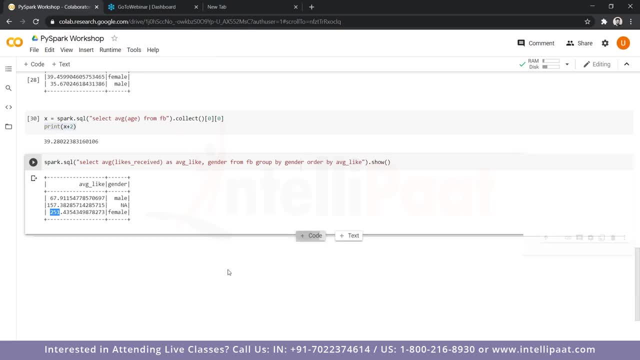 We can understand from this, these data sets. that is how easy it makes it. And then remember, you'll always have this data in extremely long formats to give you an accurate viewpoint right. So if you have 10 records of data, it wouldn't actually give you anything specific to go. 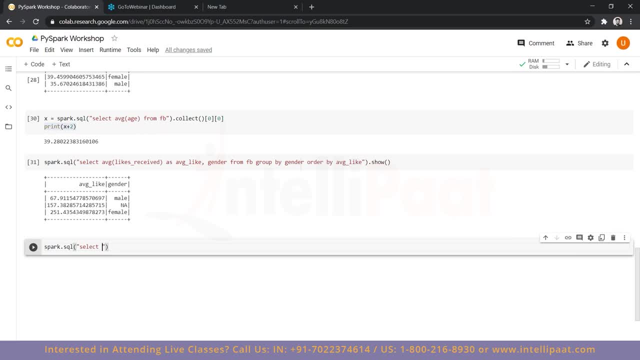 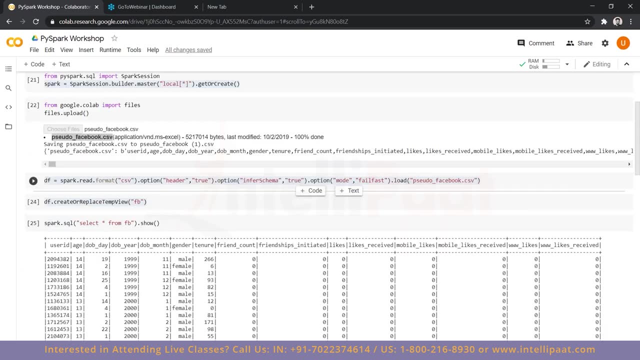 by. But when you have millions and millions of data records, you have a sort of an accurate answer as to how these things work right And something else we can do with it. let us see, let us find some, let us do something. with age demographics right. So let us understand how many friends people have between the ages of 13, to say, 25, and from 25 to 35. So let us go with age average age, Okay, Average average, sorry, not average age. um, average number of friend counts friend. 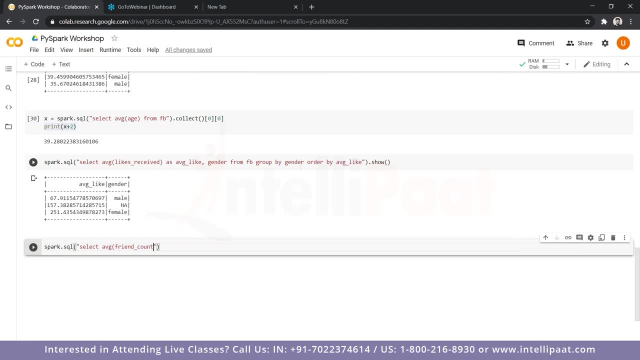 underscore count And we go by from FB. Now we can use a where clause for this right Age could be greater than equals to 13 and age is less than equals to 25.. Okay, So, let us see. Okay, So let us say age 25, uh, we do that and we click on the show. we click on that and we. 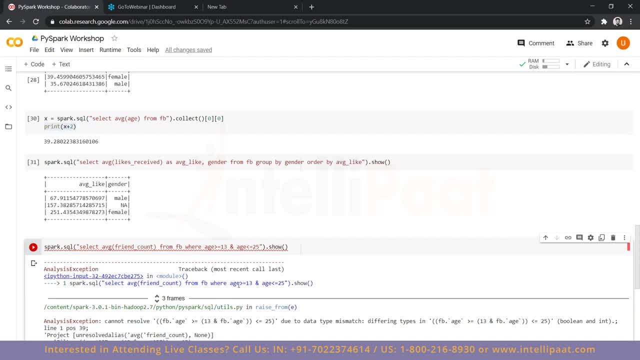 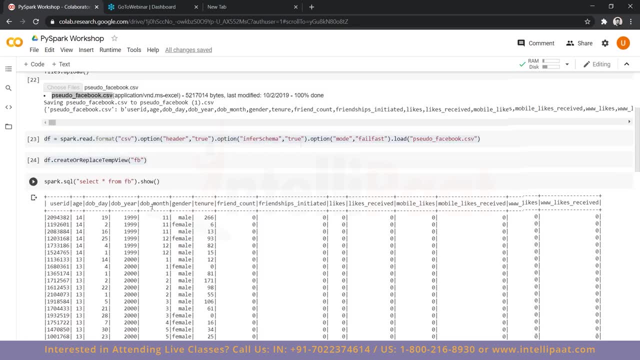 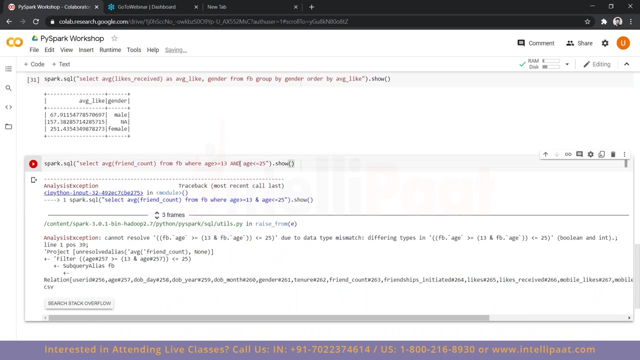 click on play. Oh, actually I think uh, so moment. what did I do wrong over here Just a moment? So is the each okay? Uh, just a moment. Yeah, So actually I got confused for a second there and implemented the uh Java over here. 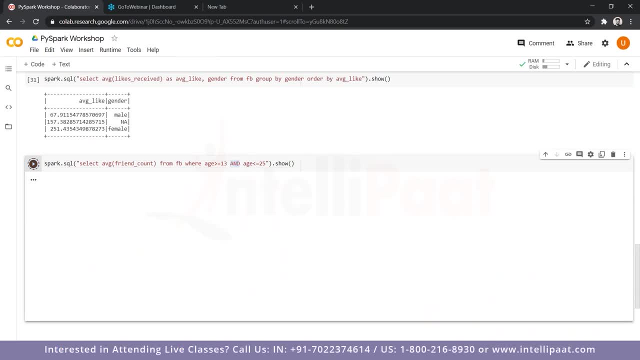 So I wouldn't, I shouldn't have done that. The and percent symbol doesn't actually work with SQL. So for the people with the SQL background, I don't know. Okay, So I forgot about that. Yeah, So when we use the, and it actually works with that. 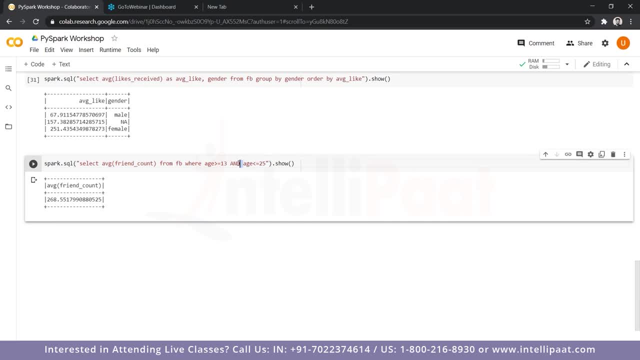 So so, uh, thank you, Deepak for correcting me. Yeah, So yeah, I use the and percent symbol there by mistake. So when you use the and, we get the average friend count to 68.. So that is the average friend count of a person that is on Facebook, but in the ages of 13,. 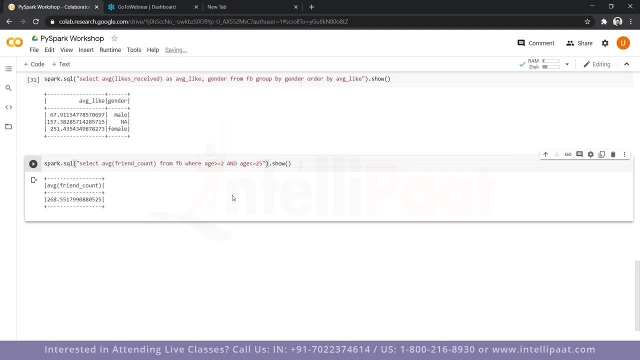 13,, 25, and when we change this to something like 26, to say um, say 50. So let us see how that works out. So that is the uh, significantly less. that is 113. that also tells us about age demographics. 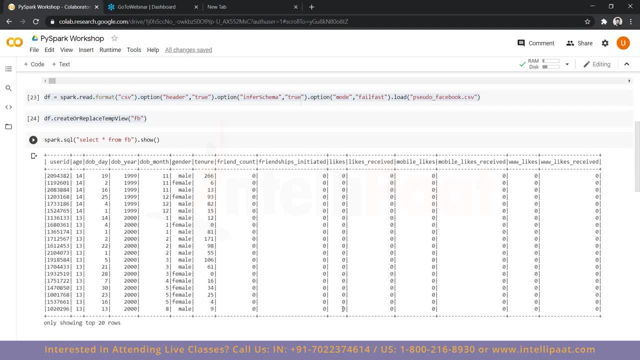 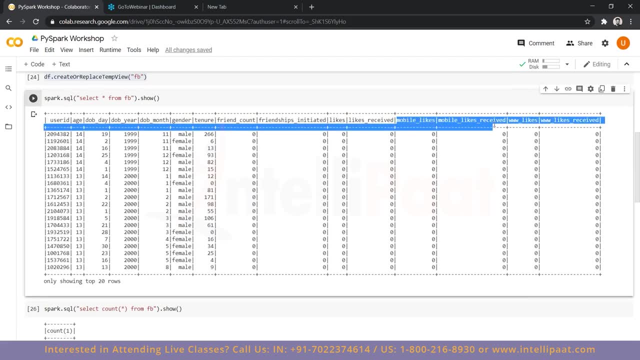 Um, if we want to find out, uh, the usage of individuals on Facebook. So, uh, there are two data columns that are available, That is, the mobile likes received and the WWW likes received. right, Uh, not the WWW likes and the mobile likes. 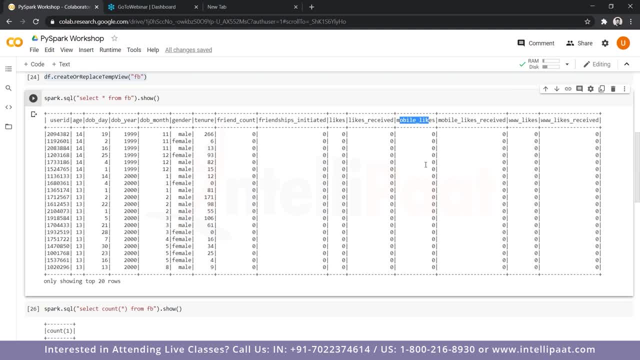 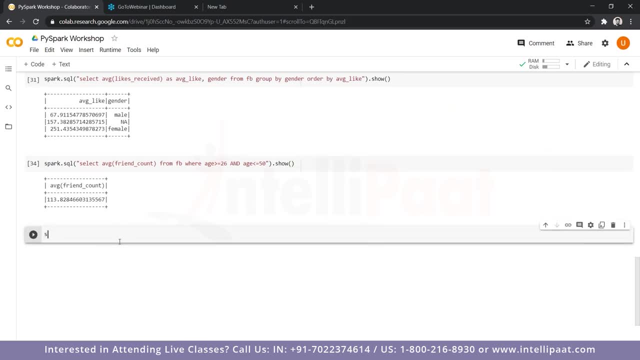 So these might seem like normal sort of columns that are there. We can also uh. We can also determine the usage of individuals like uh at an average. uh, people say between the age of SQL and some moments. Spark dot SQL select average. 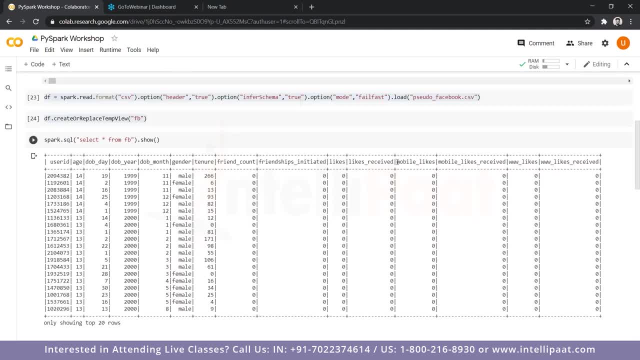 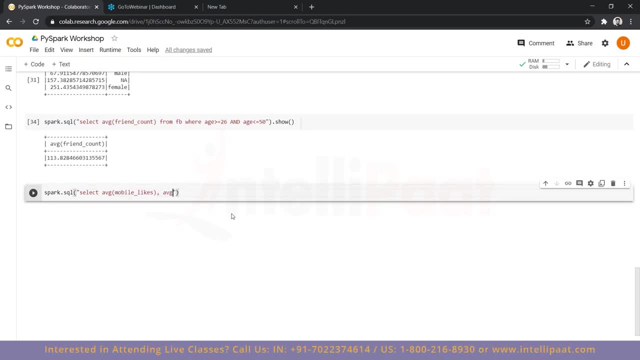 And when we say if you want to find out the mobile likes, you copy that column name and we put it over here and we take average The website likes. So Facebook from browser and Facebook from mobile applications from FB- uh, where age? 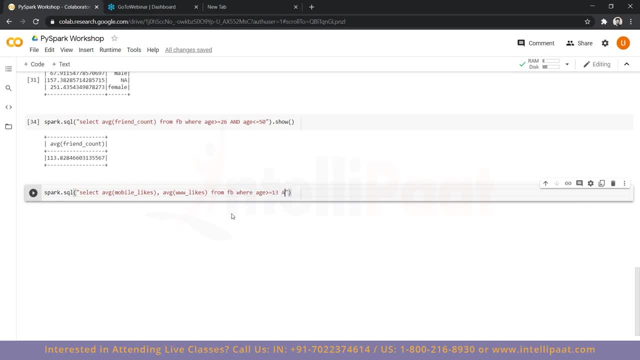 is greater than equals to 13. and age is smaller than equals to 25.. And we type in a dot show over there, We do that and we click on play So we can see that the app It's mobile. Uh, it's about 123 cities. 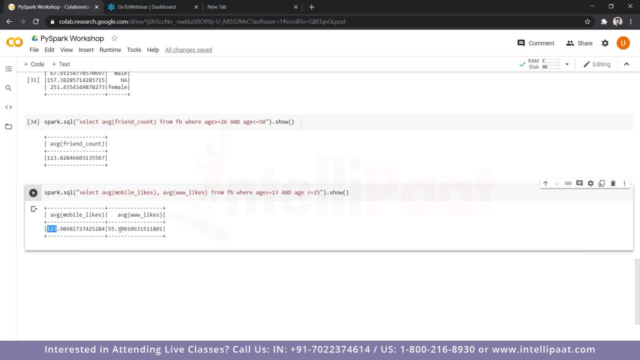 It gives us an idea, essentially that, uh, the web browser usage is quite low these days because everybody has portable devices, right? Uh, the usage of computers for accessing social media websites is quite low anyway. So we can see that this from this particular data that we have right. 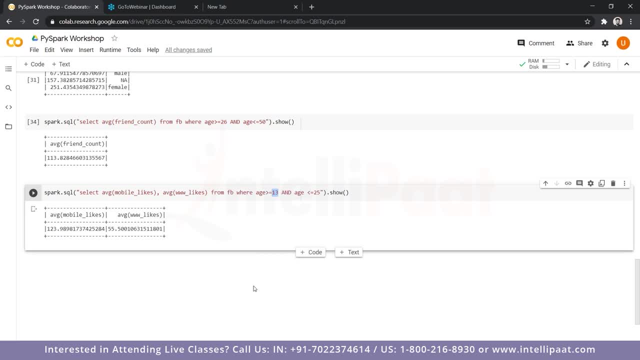 And if we change the age as well, uh, to see if there is any difference between older people and younger people. So we can type to a greater than equals to 26 and 50. Like the previous data, right, Uh? and then we can see that, uh, the web browser usage is quite low these days because everybody 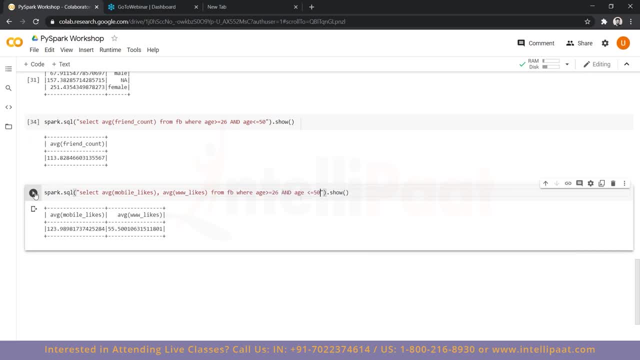 has portable devices. So we can see that this from this particular data right. Uh, the usage of computers for accessing social media websites is quite low anyway. So we can see that this from this particular data right. So we can see that this from this particular data right. 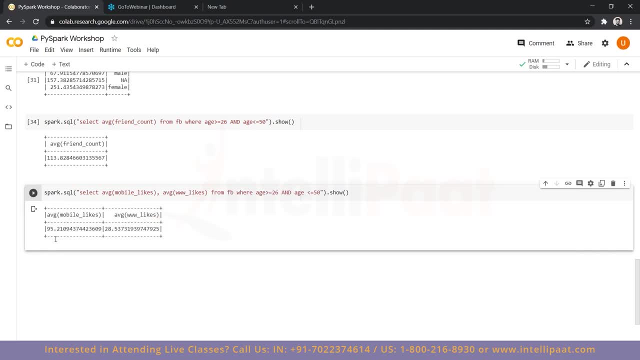 So we can see that this from this particular data right, And when we do that and we click on play so we can see that it's less. but the ratio begin uh almost remains the same. So it's a mobile likes higher and average uh web browser likes are low. 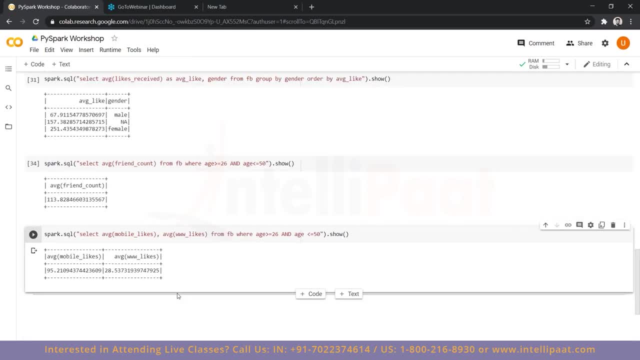 Right. So these are sort of the things that you can do with it. You can also perform some- uh- complex mathematics with it as well, So these are sort of things that you would have to do if you want to find out any relations. 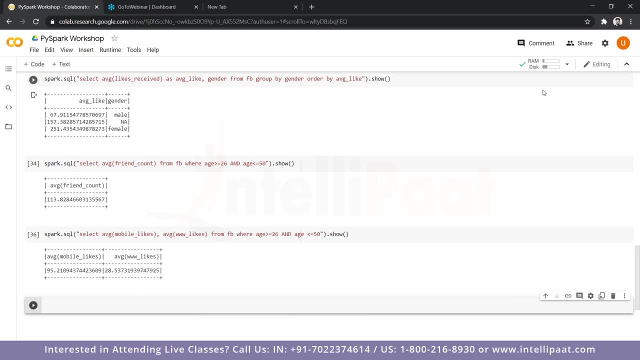 uh, between the data. So this is the last thing that I'll tell you about this before the course advisor actually joins us. right, Just a moment. So instead of using the Spark SQL context, right, You can do some other things as well. 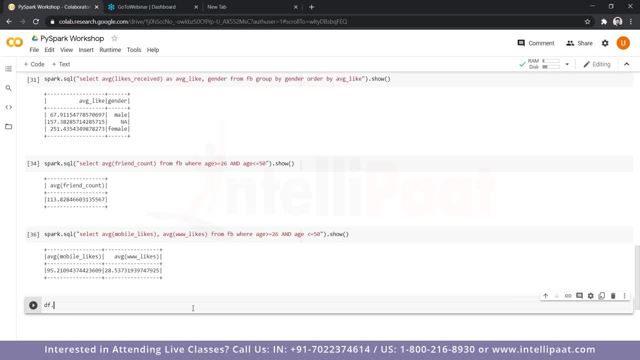 So data frames are not just limited to Spark SQL. There are other ways you can refer to them. So, for instance, if you want to use something other than Spark SQL, right, If you're coming from a development sort of background and you want to do some complex modeling with your data. 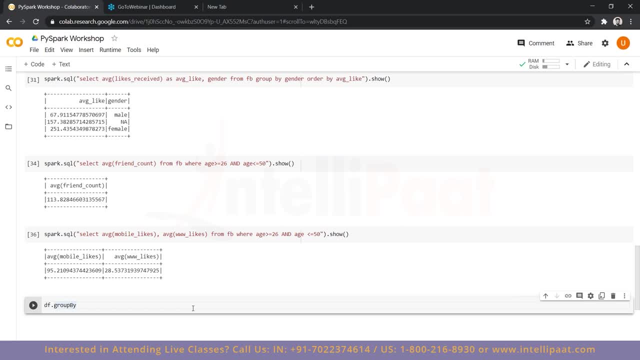 right. In that case, you'll use the group by like directly on the DF, instead of using the FB, which is the virtual name for that. in this SQL context, you'll use group by And, for instance, if I want to refer to a column name. 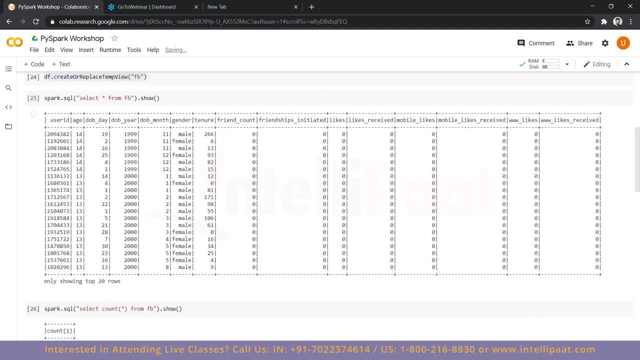 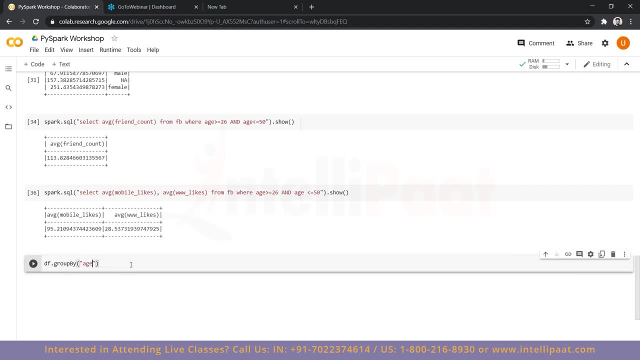 in group by right, So I can simply type in: for instance H, For instance H, let's use H. Let us group all of the data by H, right? And then, once we've done that and we want to do something else, 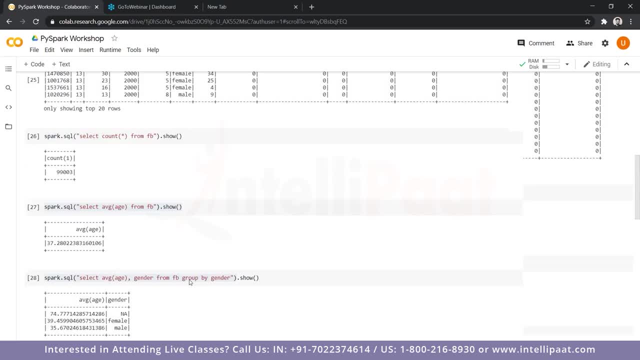 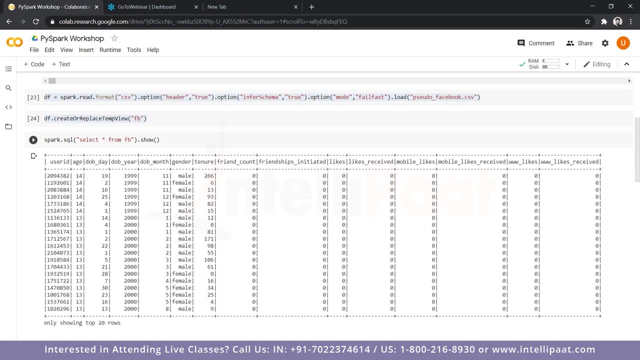 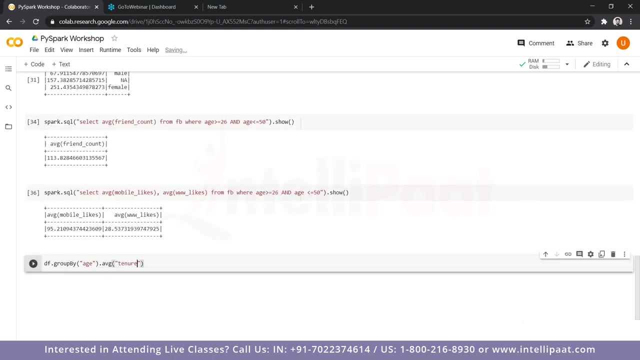 for instance, we want to calculate the average, And for average I mean, say, we want to find out the tenure of the person on Facebook, right? So let us use the tenure column name. So once we've done that, then we will type in order by: 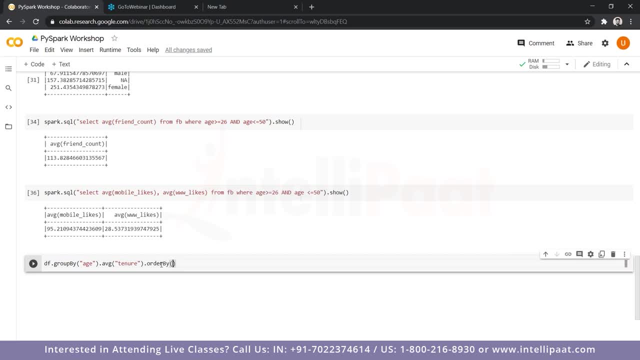 So we will sort this data by the, let's say, H. We want to sort this data by H, right From lower to higher, if we want to sort it like that, And then if you want to sort it by lower to higher, 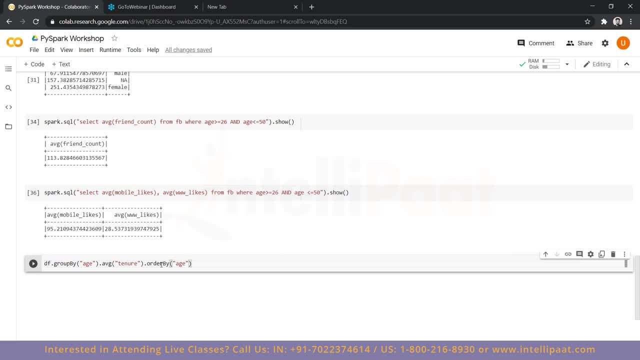 we can simply go ahead and given the ascending value as true. If you keep it, if you don't actually add this, it's by default considered to be true, right? If you want to actually arrange it in descending order, right, it'll actually give you the ascending value. 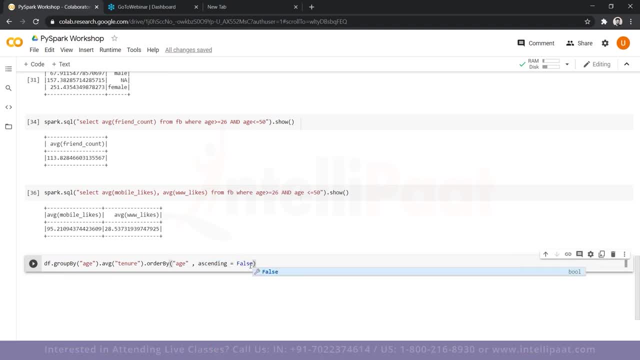 as true. So if you keep it, if you don't actually add this, it's by default considered to be true. right, It'll actually give you the data in descending order. So, firstly, we'll do it in descending order. 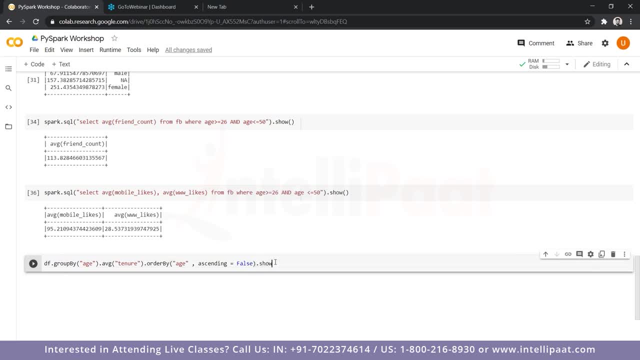 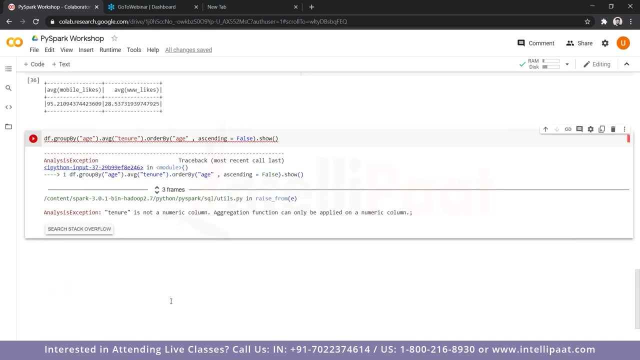 then we'll do it in ascending order right, And we type in dot show. So once I do that and hopefully, if there are no mistakes, it should run. So there's an issue with that. Tenure is not a numeric column. 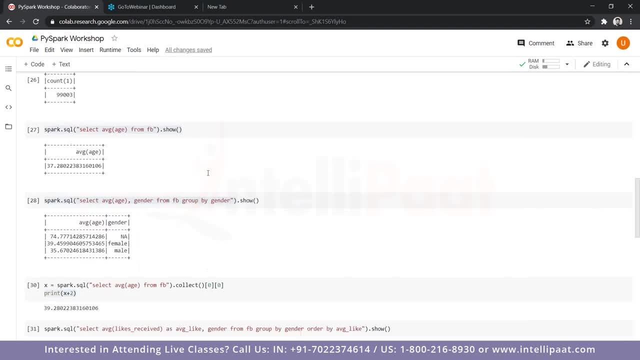 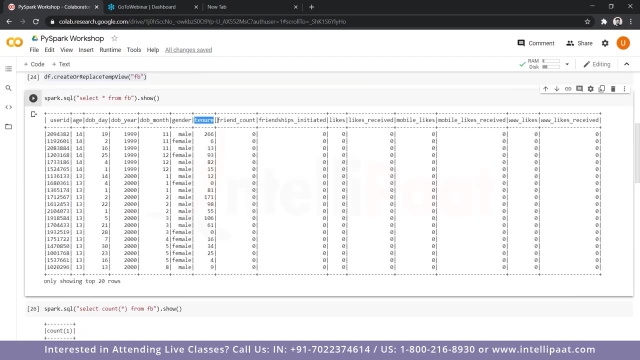 All right, so this particular column is not entirely numeric, I believe. So there's some problem with the data set in that regard. So I'll not use tenure. let us use something else. Let us use friend account again. So there must be some string values as well. 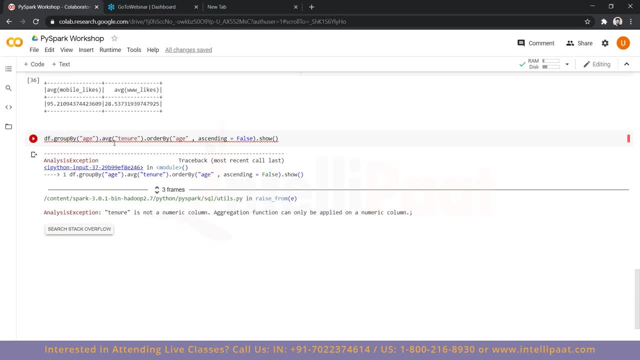 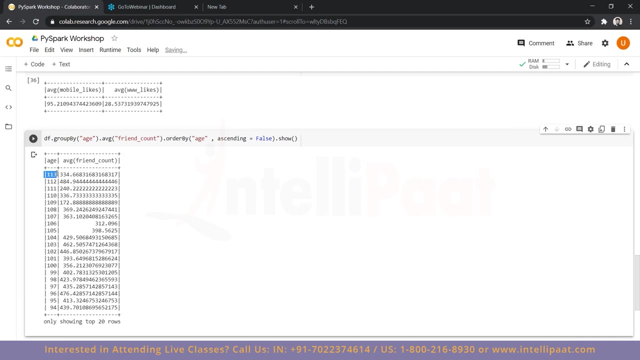 So it's not entirely a numeric column. in my opinion, then There are string values in that as well. So we'll change this to friend count and click on play. So that is something that we have. So we can see that there are people. who've given wrong ages as well, or maybe impossible ages as well. There are as high of ages as 130 that are there on Facebook. So that is there, And the average friend count, which I believe for the person that is of 113 age on Facebook is about 334.. 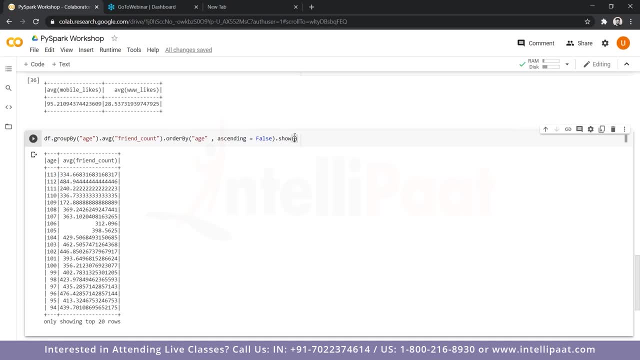 There's 112 and so on and so forth If you want to see a lot of these to us. So if you type in 113 over there, we'll see 113 records. Click on that And it starts from 113.. It goes all the way down to- I think it will go down to one- It'll actually not go down to one, I think- the minimum Facebook age: I think it will go down to one. I think the minimum Facebook age limit is 13.. 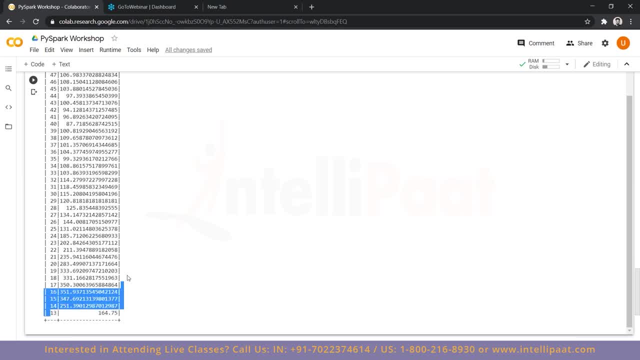 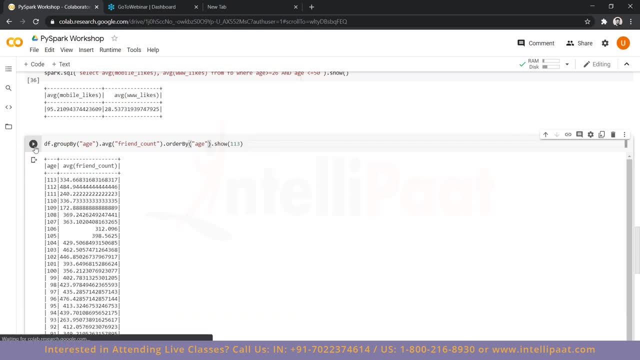 It will go down to 13.. So it goes down to 13. And from 13 up we have this, And if I simply remove this and click on this particular button, the play button, we get the data in ascending order as well. So it starts from 13 with the average friend counts of 164.75.. And we go down, We get the average friend count statistics for every age. So this is how easy it makes us makes this particular job to be right. 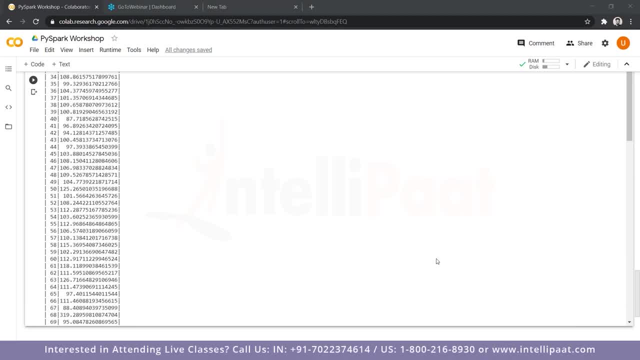 So hold on tight. I'll be contacting my course advisor now to guide you guys with the career opportunities that Vice Spark has, the career opportunities that Big Data has in general, to guide you with any of the questions that you have career-wise. So I'll resolve some technical doubts before I actually do that. 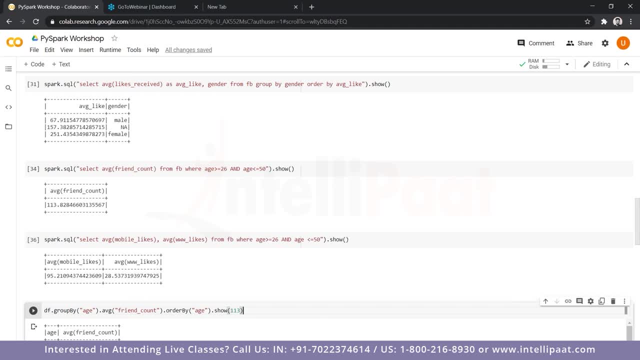 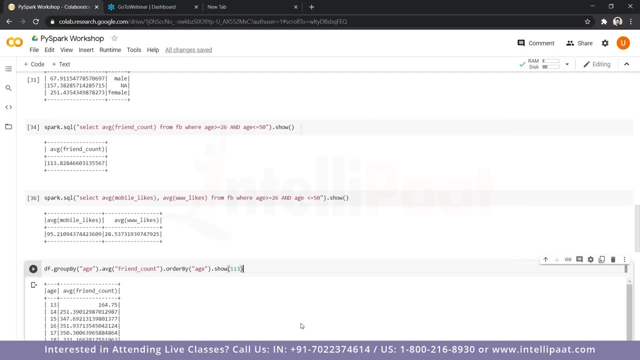 How do we integrate Spark with machine learning? So Spark also comes in with libraries called MLib, Like Spark has a library called MLib Spark. MLib deals with MLib, MLib deals with the cluster-based machine learning computation. So basically, creating machine learning models is a very daunting task when you're dealing 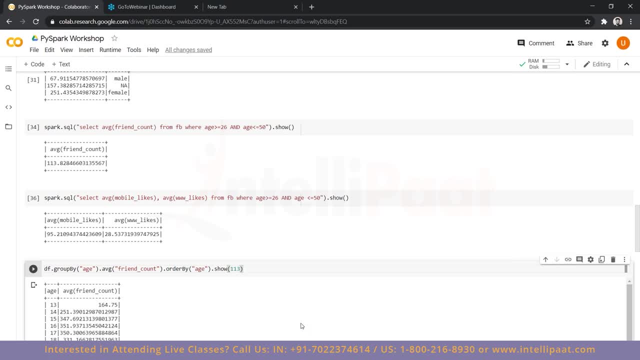 with big data, right? So you're not going to be actually dealing with machine learning in a linear sort of format on one system. You're going to be dealing with creating machine learning models using the processing power of multiple systems. So for that case, Spark also provides the MLib libraries which you can use for machine. 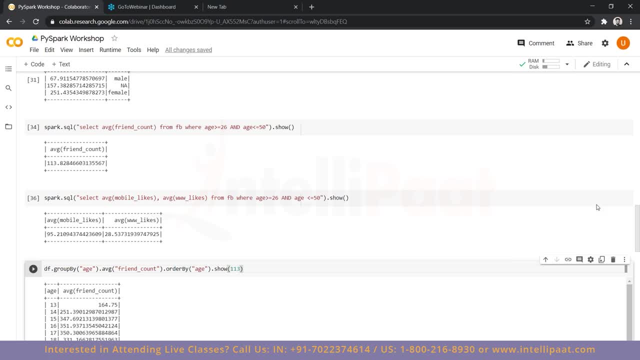 learning purposes? Okay, So data science roles: how much by Spark is required? Okay, So this is quite an interesting question. For data science at a base level, you don't need by Spark at all, right, If you're dealing with data analytics, right? 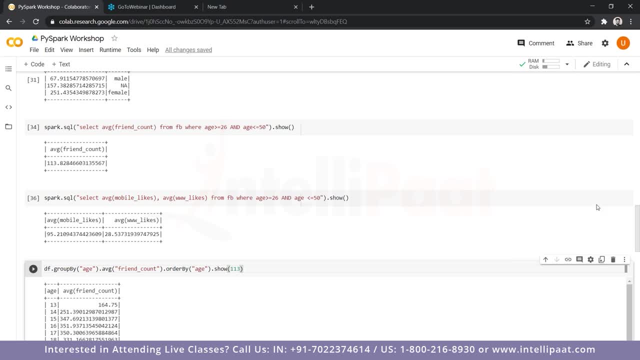 Data analytics on its own is not that well of a paid sort of a profession, right? Data analytics is the entry-level profession in data. right, It's the basic level profession. When you get into big data you get quite a high bump in your career relationship, right? 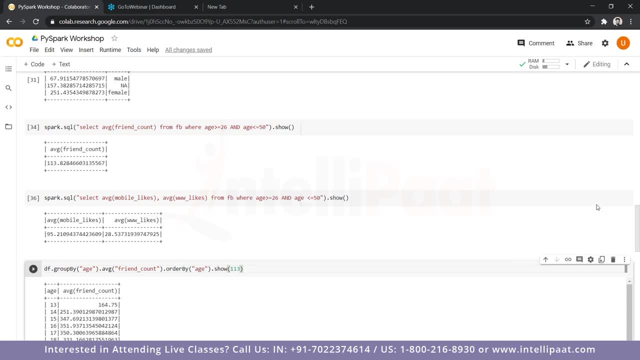 Right, Okay, That's a good resume, So to speak, because you now know how to handle data at a very grand scale, which is the case with a lot of big companies today. right? So, once you understand how big data analytics work, like data analytics when you're dealing. 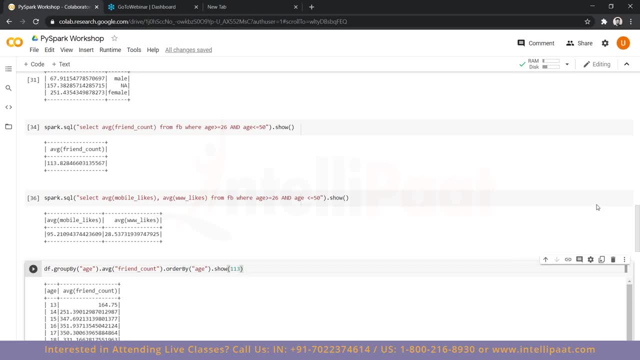 with big data right. Then using that knowledge, you can integrate that pretty easily with your Python knowledge, say, for instance, in data science right, Or your R knowledge in data science. So, instead of doing your data analytics, data science jobs. 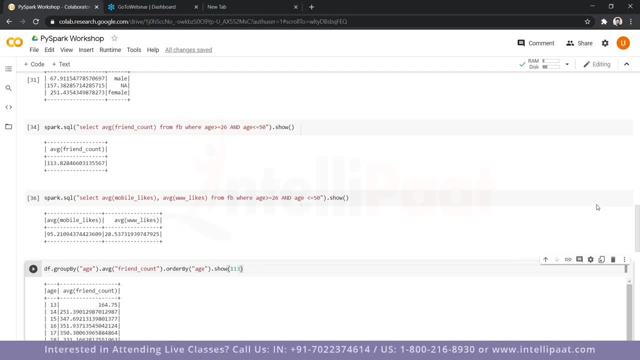 On small data sets, like you were doing earlier. now you're doing that same job on big data, And that is what is required in today's industry: Somebody who knows big data and is implementing data science with big data, using data visualization with big data, using cloud services with big data and then implementing machine learning. 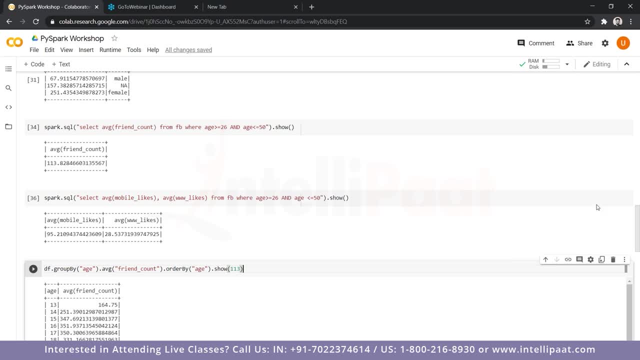 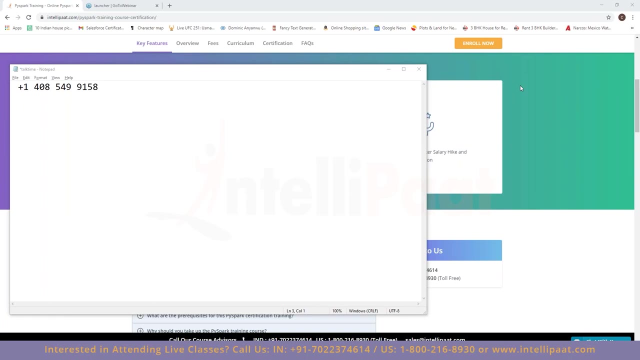 and artificial intelligence with big data, because your machine learning algorithms and your artificial intelligence algorithms will be extremely accurate if you're creating them with big data, Because it takes a lot of data together to create data Okay. So thank you so much for your participation and have a great day ahead. Bye, bye. 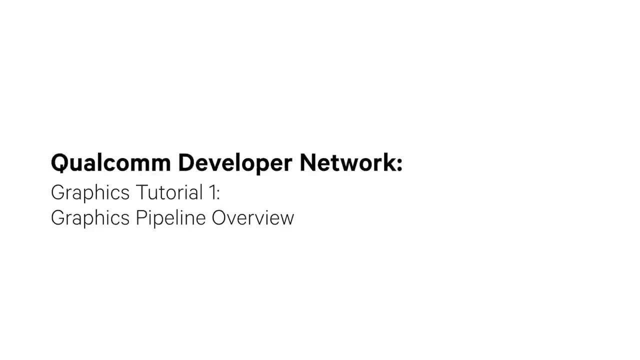 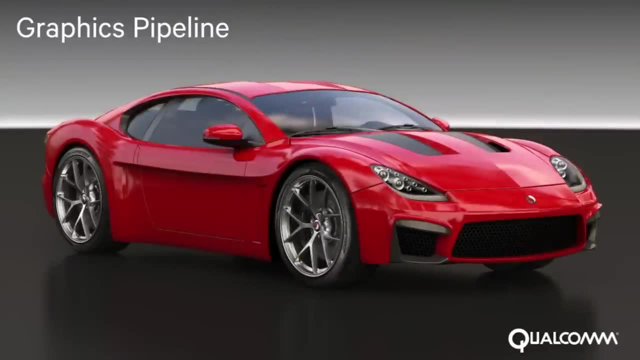 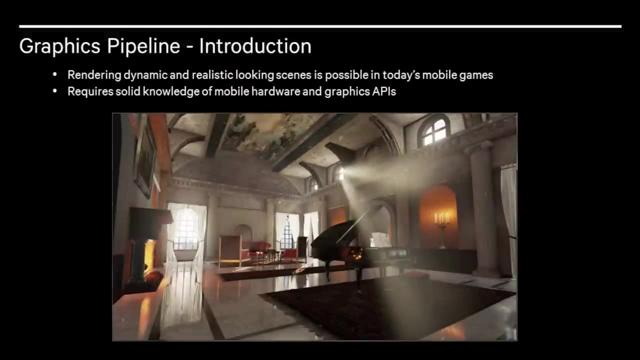 Hi, I'm Pete Brubaker, a staff engineer with Qualcomm Technologies. Today I'm going to introduce you to the graphics pipeline. This is a screen capture of a demo scene running on mobile hardware, As you can see the results we are able to achieve on mobile hardware. 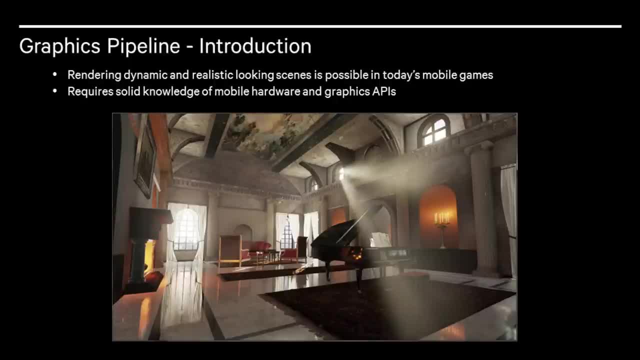 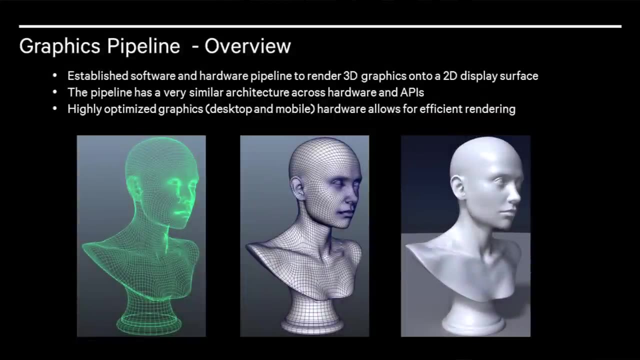 are exceptional. Building scenes like this requires solid knowledge of mobile hardware and graphics APIs. In this presentation, we're going to introduce and explain the graphics pipeline from a high level. What is a graphics pipeline? A graphics pipeline is a set of software and hardware to render 3D geometry onto a 2D surface. The pipeline has evolved. 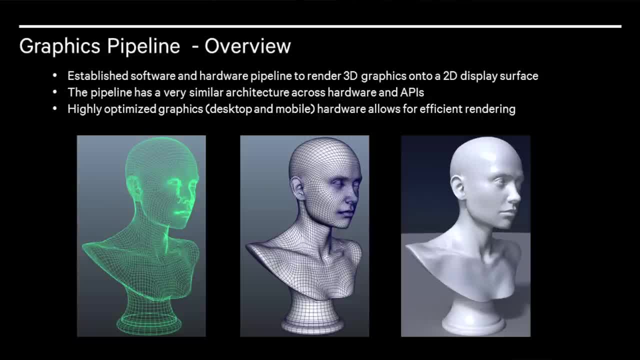 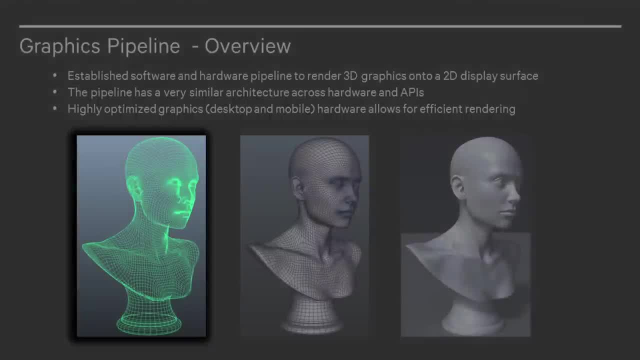 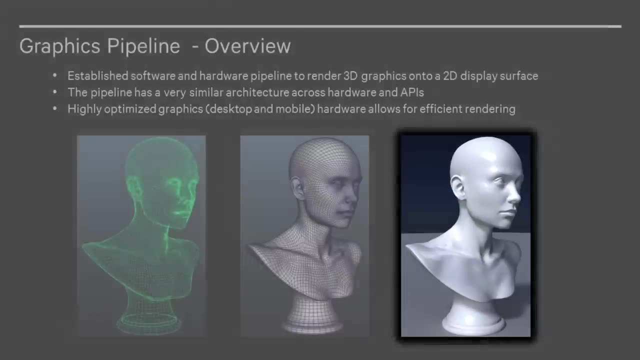 over years through many revisions of APIs like OpenGL and DirectX. Most of the heavy computational work is accelerated by specialized hardware. The image on the left is a highly detailed mesh and is shown flat, shaded and rendered on the right. Let's dig deeper into the pipeline and see what happens inside the pipeline.